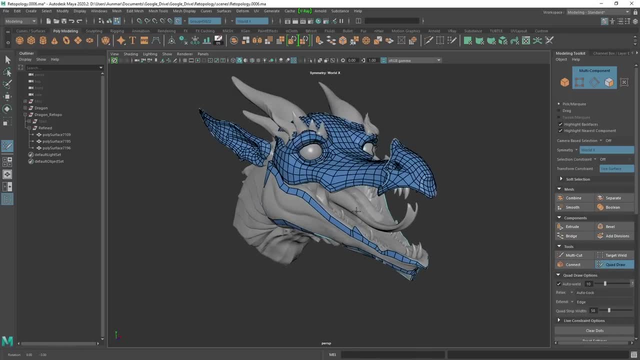 So I'm going to show you guys everything about Quadraw here in just a moment, but I did want to say a big thank you for Richard Brice Gore, who gave me the sculpt model, and I'll see you in the next video. Bye. 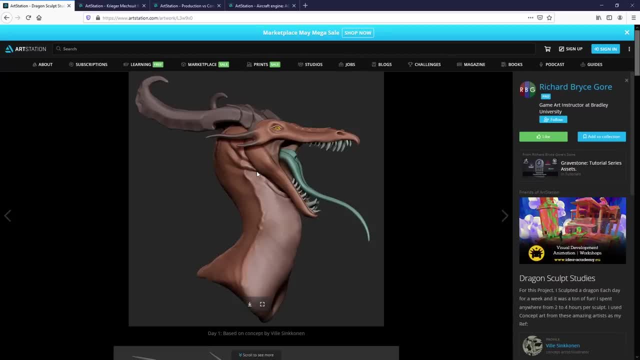 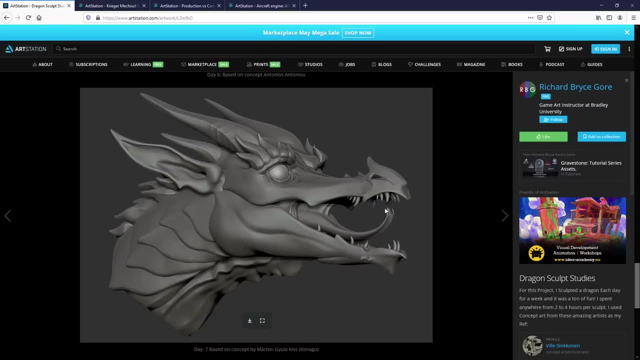 You can check out his work on ArtStation and I pulled it from one of his daily sculpts that he did here right off of ArtStation. So we were talking about topology and I really wanted to kind of demo this on this cool looking model. He also does some YouTube videos and tutorials. 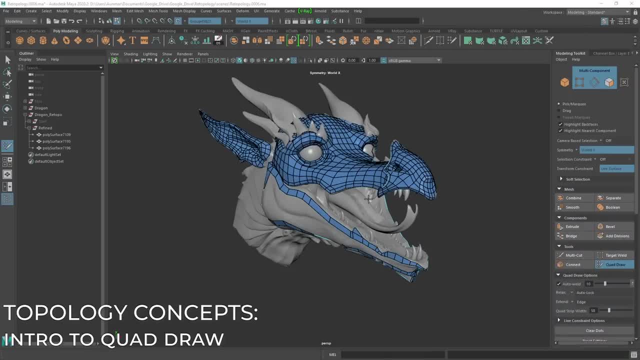 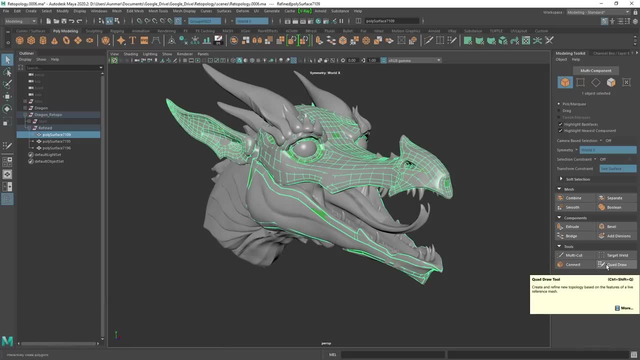 so make sure to check that out. So now that we're back in Maya, you can see what I have here, okay, So the first thing I want to cover is just the tool Quadraw and everything you need to know about it. So the key thing here right now is if you already know how to. 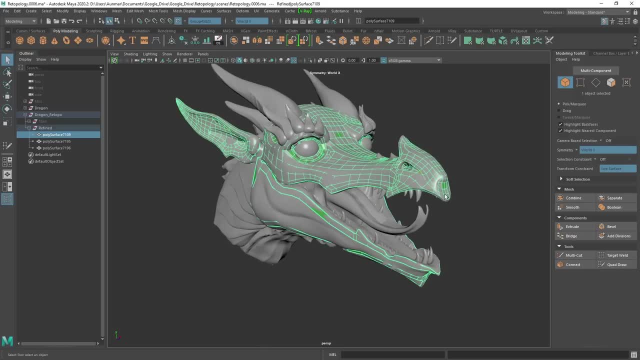 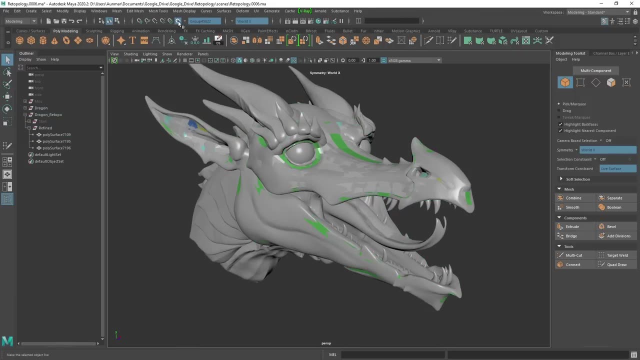 do Quadraw? go ahead and skip to the table of contents down below or to the next section, and then we can start talking about topology. But first let's go ahead and take a look at how to use Quadraw. So I will go ahead and grab this dragon model. I'll hit control one to isolate. 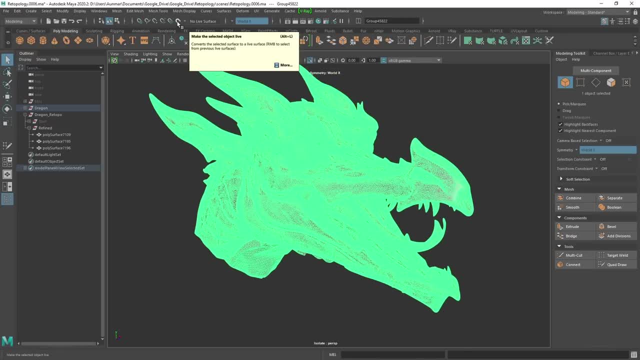 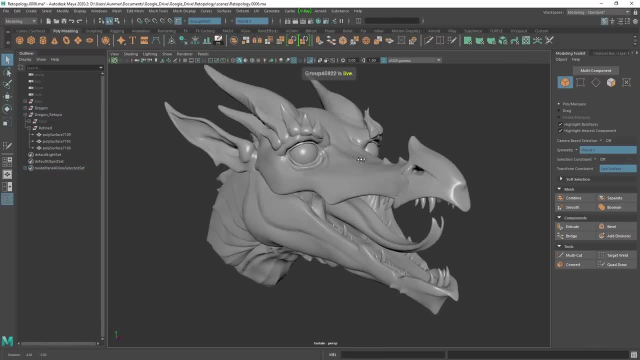 and I'll go ahead and do what's called set live surface or make selected object life. Okay, So, with this dragon selected, I'll go ahead and hit this magnet up top here and you can see that it went ahead and set this live surface. Now just to. 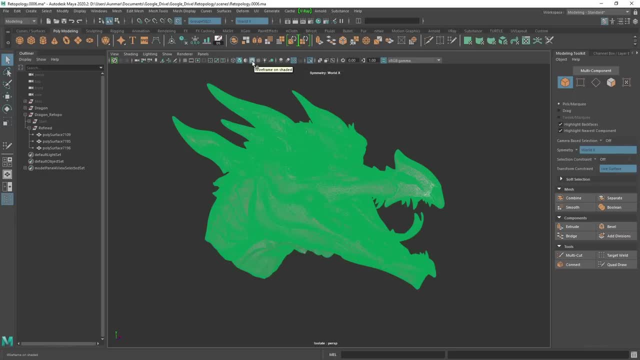 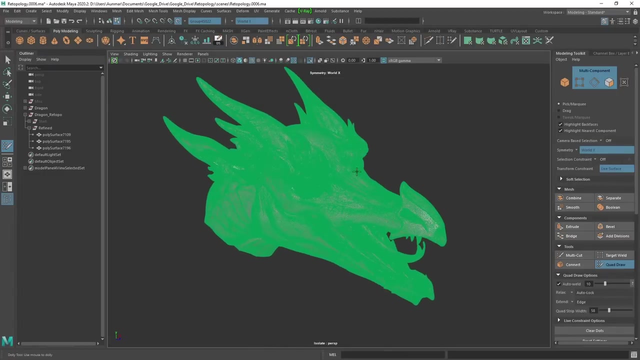 be sure how do we know if we go ahead and hit this edge or wireframe on shaded here you can see that it's green and that signifies that this is now a live service, so you can no longer select it. All right, So if I go ahead and enable Quadraw, you can see. now I can start. 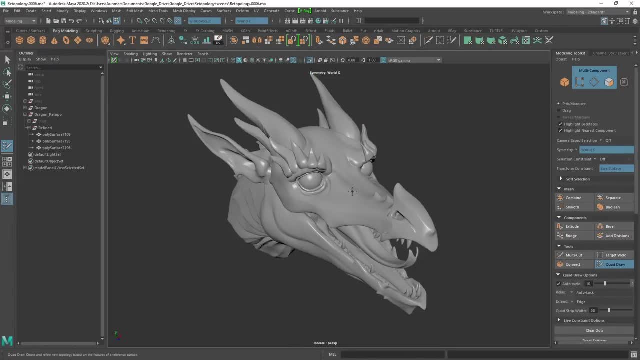 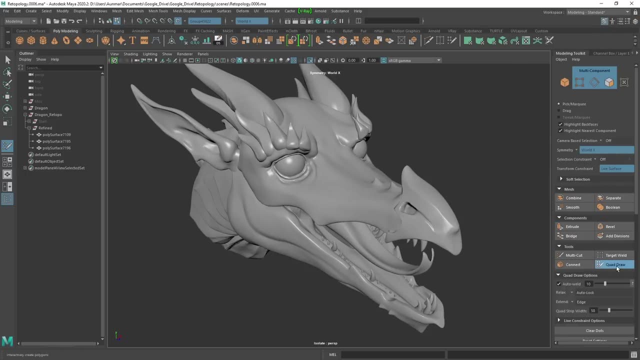 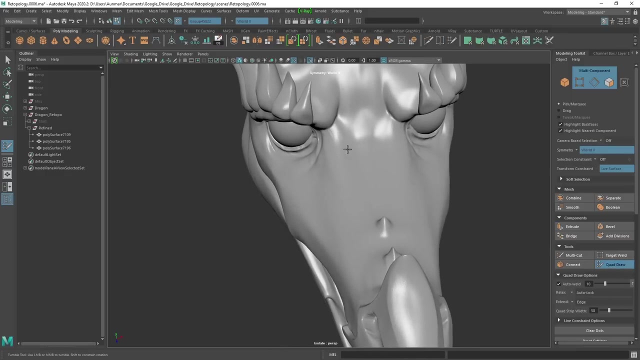 I get kind of a different looking cursor, I'll go ahead and turn off the wireframe on shaded mode and begin plotting some points down. Now again, you can get to that from the modeling toolkit and enabling Quadraw here. Now Quadraw works, It's kind of in the name. It's you draw quads, All right, So we're going to plot. 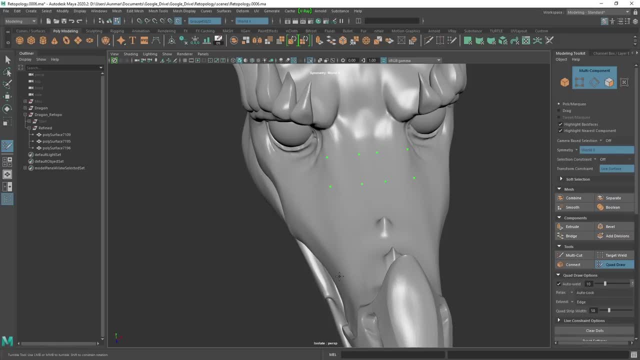 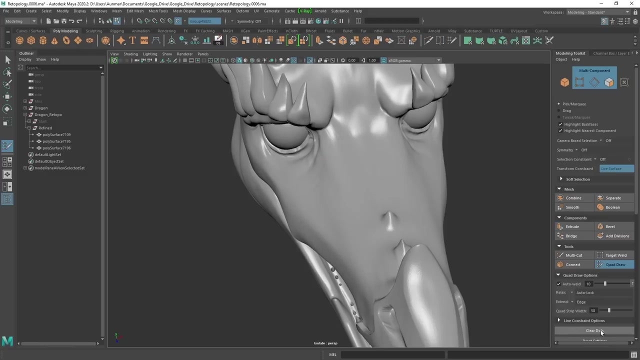 four points. So, as you can imagine, each one of these points here that I'm left clicking is a vertice that equals up to a quad or a polygon. All right, So if I actually go ahead and turn off symmetry, because I don't want to confuse anybody right now and we can do a clear dots, 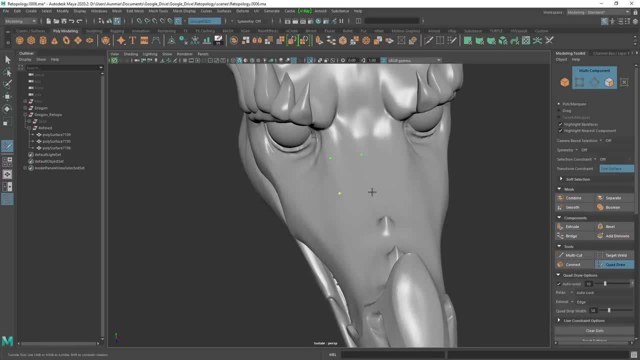 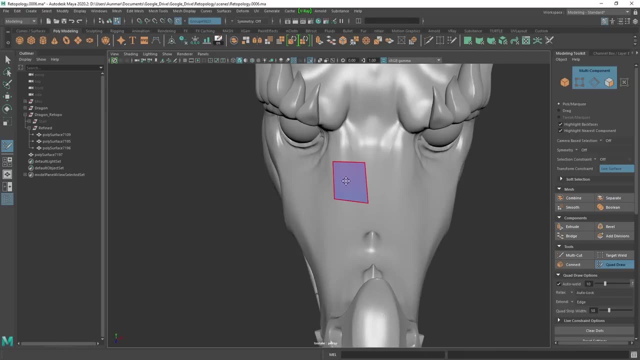 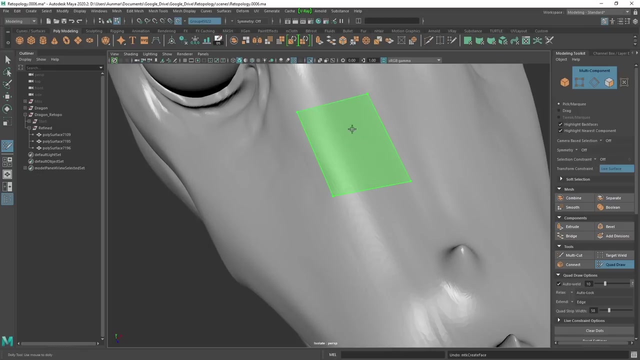 down here on these settings. So I'll go ahead and just do 41234 just by left clicking And then you kind of hover on the inside here and hold shift and then left click once you're inside And it lets you know that once you're inside and you're holding shift it'll let you know. 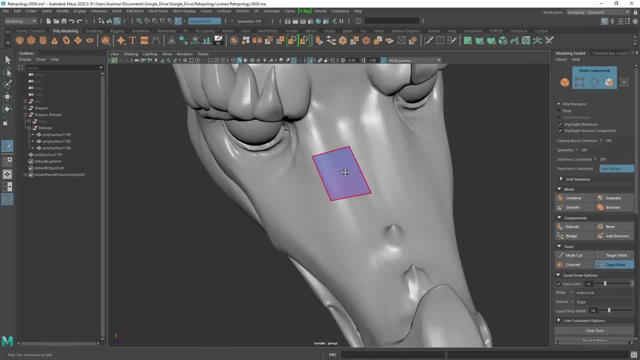 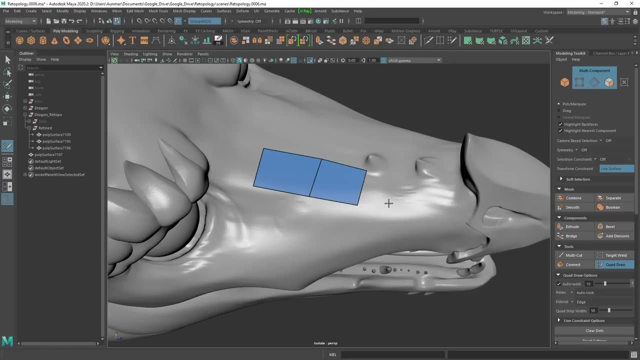 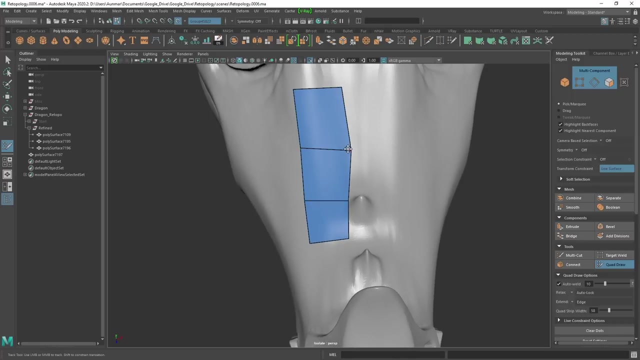 this icon here, or this highlighting effect that you can click and create a quad there. Okay, Now, once you've created the initial quad, you can continue to plot points down and continue to create more polygons and quads here. Now, obviously, there's way more tools than just left. clicking some vertices. So I'm going to go ahead and do 41234 just by left clicking, And then you can just hover on the outside here and also bring your mouse to the inside. and then you can go ahead and just left click and continue to plot points down and continue to create a quad there. 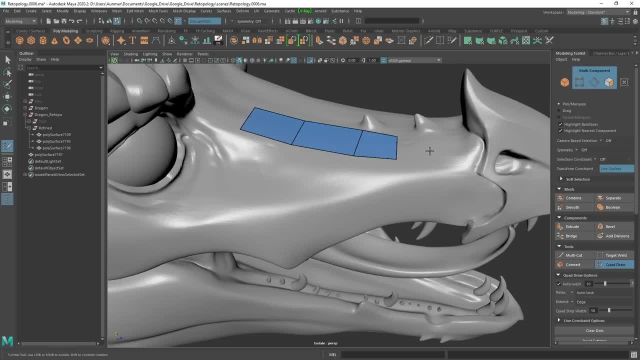 Now, once you've created the initial quad, you can continue to plot points down and continue to create more polygons and quads there, And then you can press shift and hold shift and hold shift. I highly recommend just taking a look at some of these settings here. 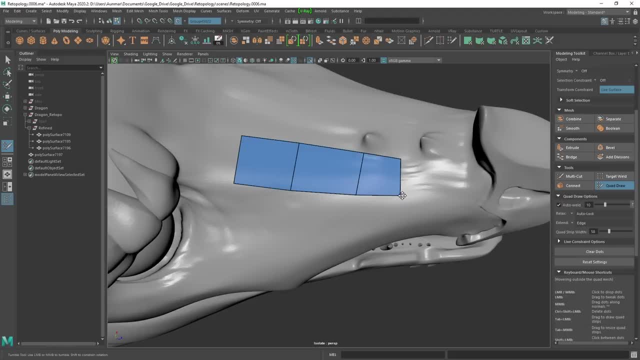 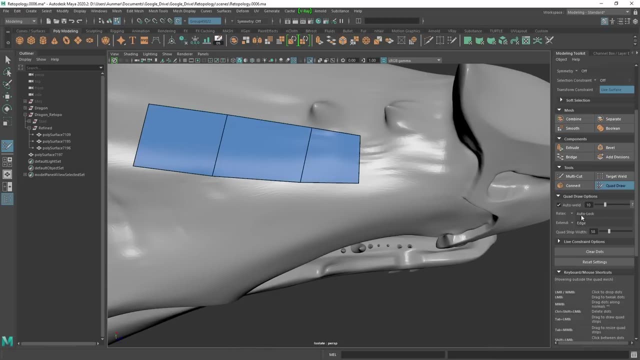 Now, if I go ahead, you can see there's auto weld here. if I drag one of these points here closer to the other points, it'll automatically snap and weld. Okay, So you can change that setting by here. And then you have kind of some other options which we'll look to in a little. 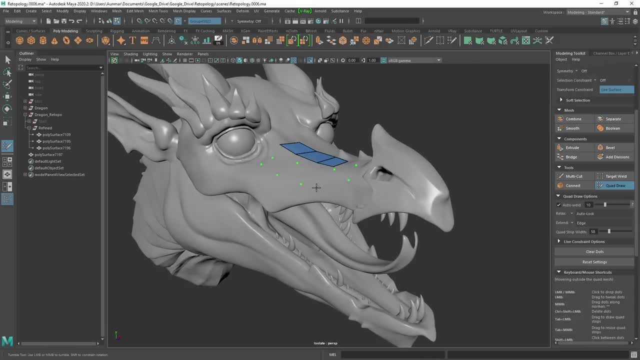 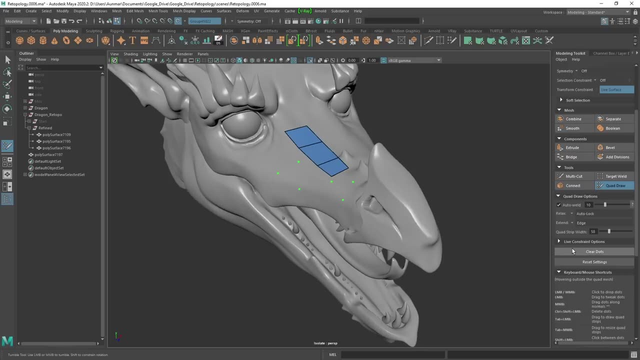 bit here. Now, if you accidentally create like a bunch of points, and you accidentally create a bunch of points here and you accidentally create like a bunch of points and you you want to delete them, you can hold Ctrl, Shift and left click. Or if you want to clear everything, 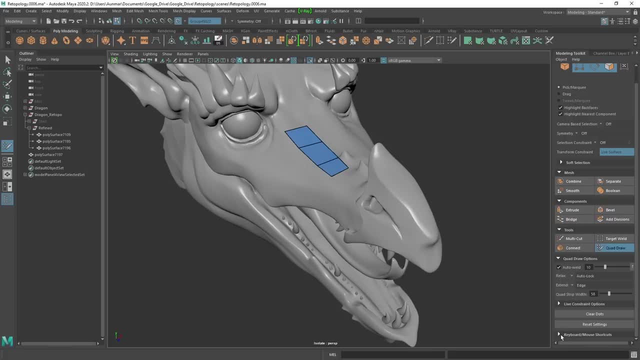 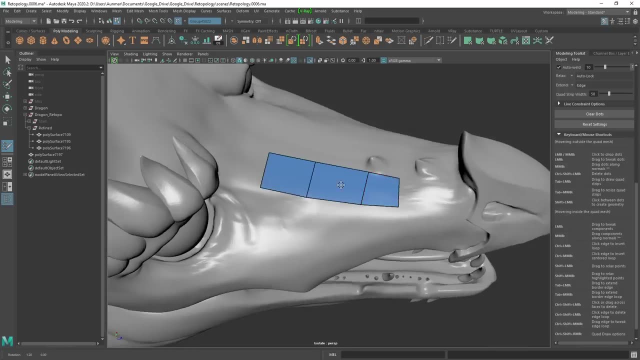 you can simply hit clear dots Now all the way at the bottom. here you can see keyboard, mouse and shortcut, So we'll quickly run through the majority of these here. So we have left mouse button which is just simply creating the points here And then by holding Shift on the inside. 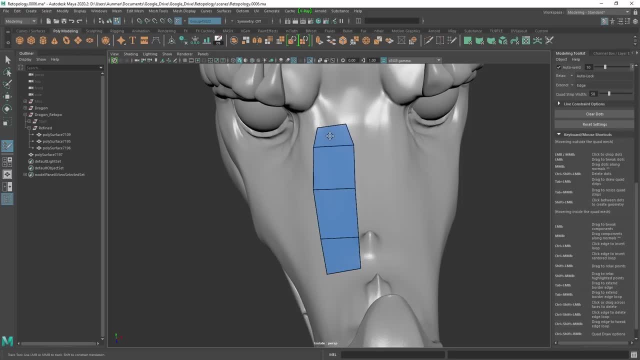 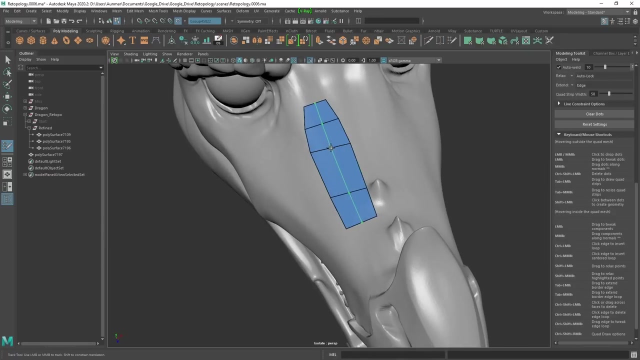 that's going to create a new face. Now middle mouse button is going to move and manipulate your edges, your faces and your points here. Okay, just by simply holding middle mouse button. So it's just a way to tweak and modify things. Now, if you, let's say, hold Ctrl and left click, 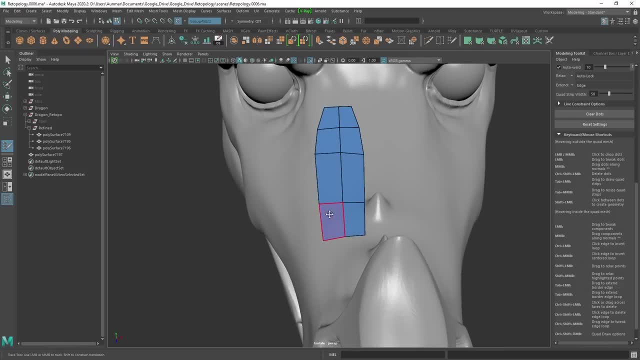 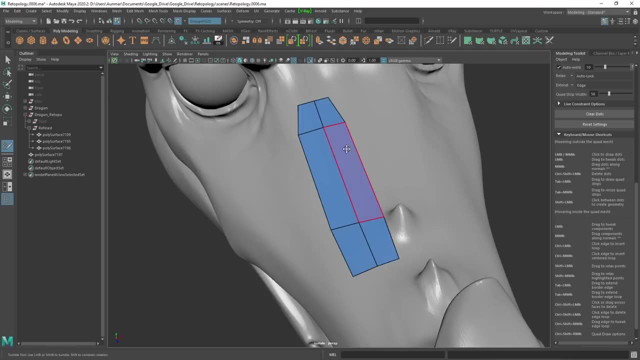 all, right, now you've gone ahead and added an edge that runs down here, So what you could do is use Ctrl Shift and start left clicking if you wanted to remove some edges, or hold Ctrl to left click and add edges. So Ctrl Shift. 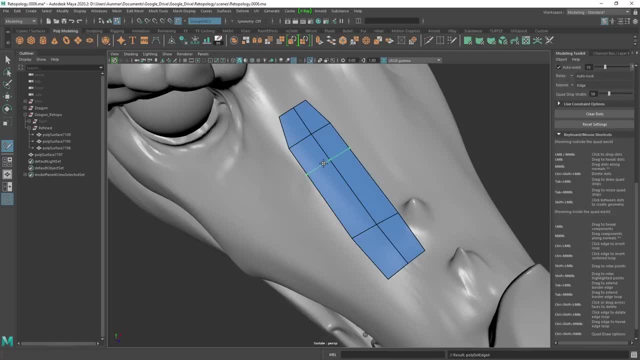 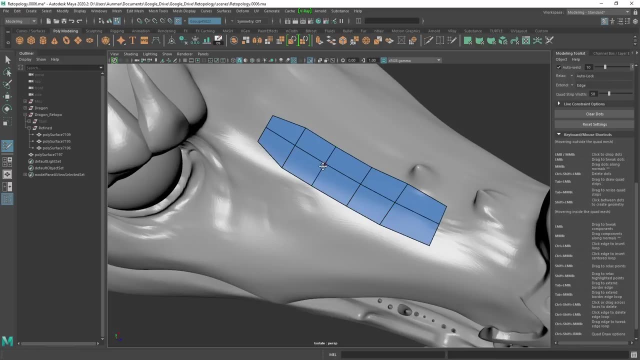 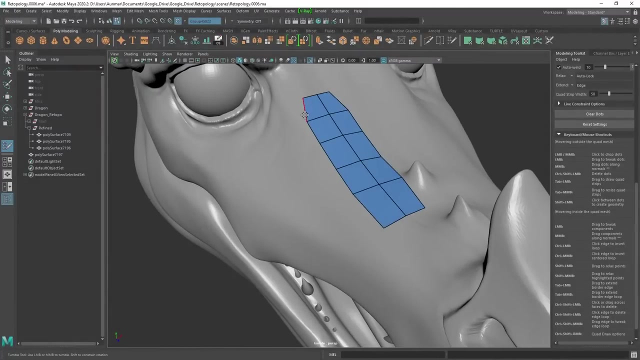 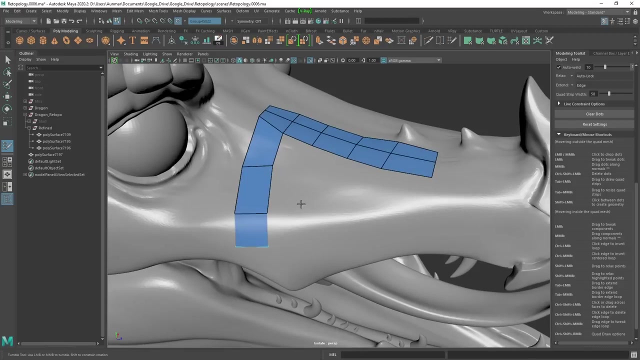 Shift to delete and Ctrl to add. So that's Ctrl, Shift, left click and Ctrl left click. All right, so you have those there Now. another cool thing that you can do is use tab. Now. tab just allows you to just grab the edges and allows you to just copy edge face edges along the surface. 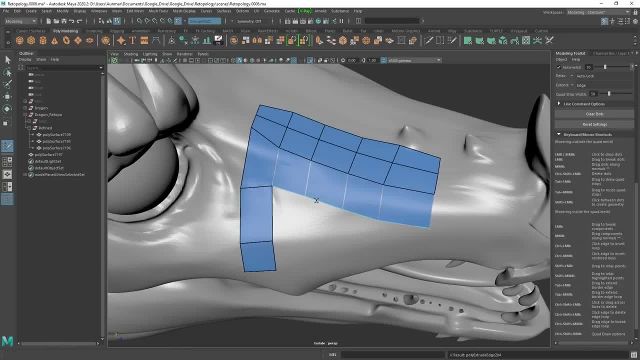 Now you could also hold tab and middle mouse button to do an entire edge face. Now you could also hold tab and middle mouse button to do an entire edge face. Now you could also hold tab and middle mouse button to do an entire edge face. So just like you can. 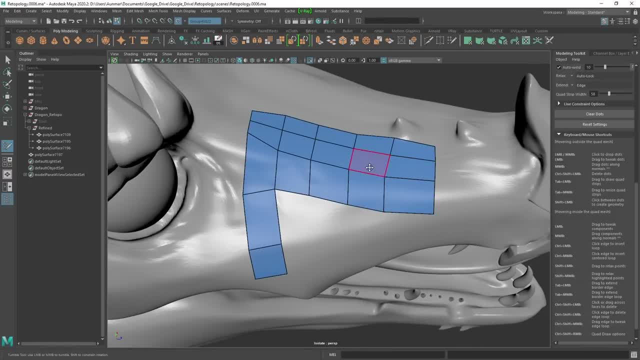 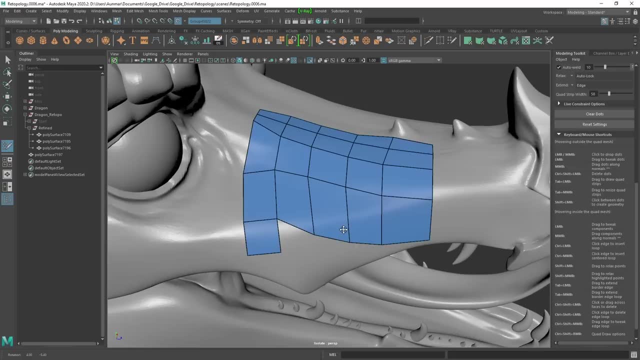 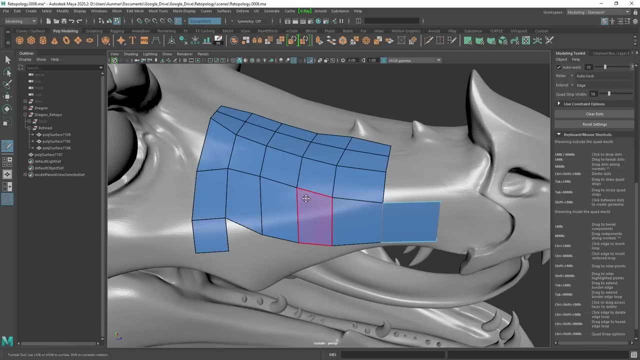 kind of hold Ctrl Shift and, you know, remove entire edge loops. you can hold tab and middle mouse to copy entire edge loops, or tab and just left click to copy edges. Okay, now again, as you start to build up some surfaces and you don't want faces, you can hold Ctrl Shift and just start. 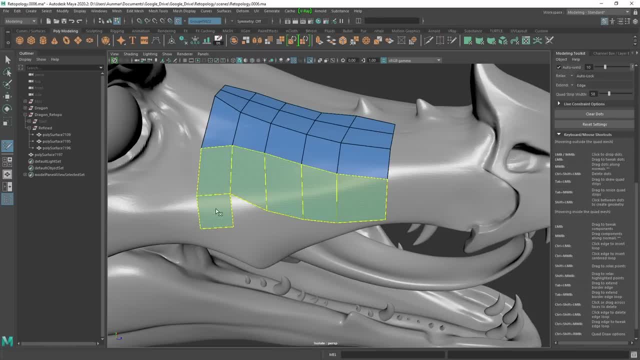 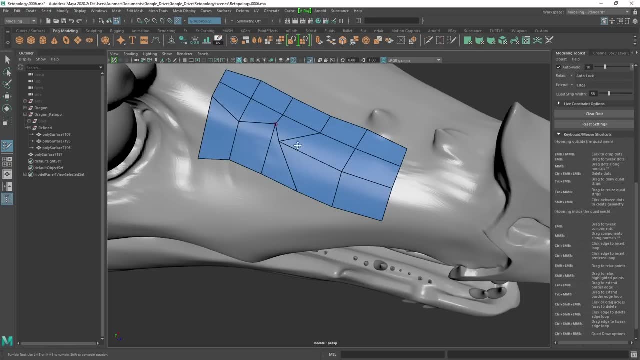 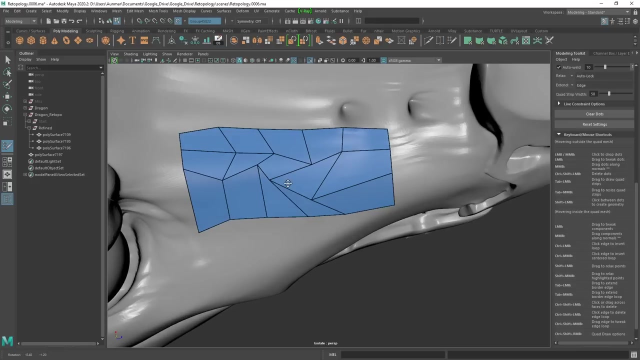 deleting them. Now you can click and drag, hold as you're going and delete entire edge loops or face loops. that way, And you can, let's say, if things are a little bit messy and unorganized like this, you can hold, shift and do a relax. So shift- left mouse button does this nice relax and 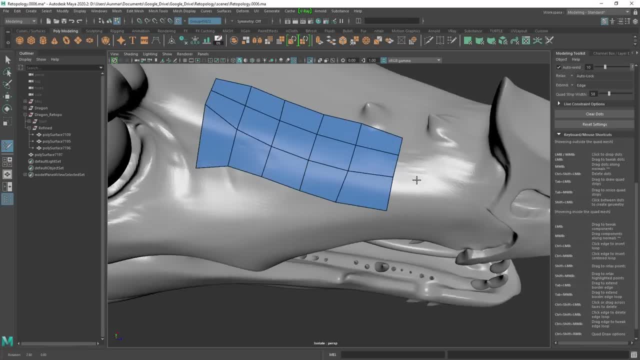 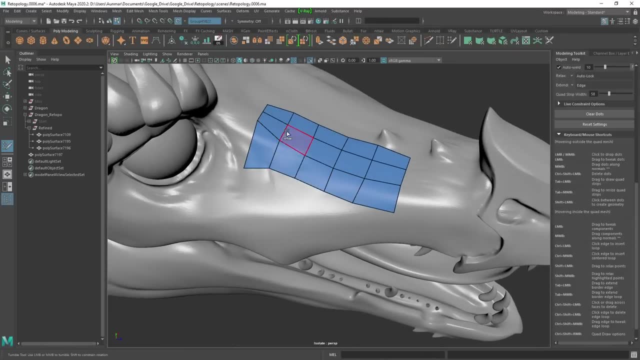 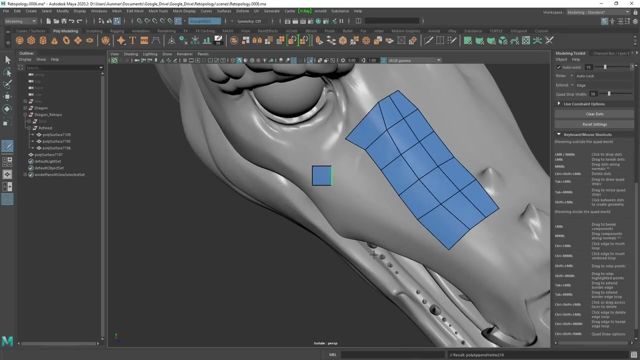 look how it just kind of evenly distributes all of your edges Alright. so I would say that is the majority of the tools here that you're going to be using as you're continuing to build up, And I'm going to show you how to do that. So if you're just starting out, you can just hold tab and just 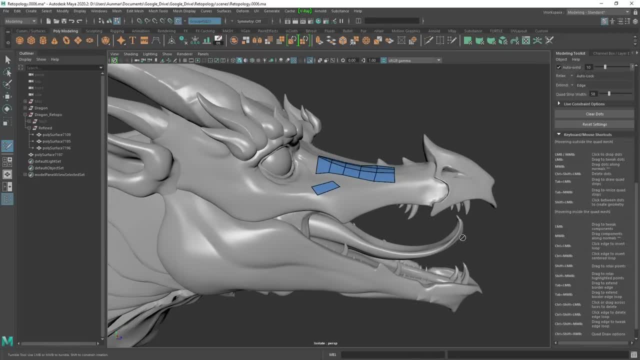 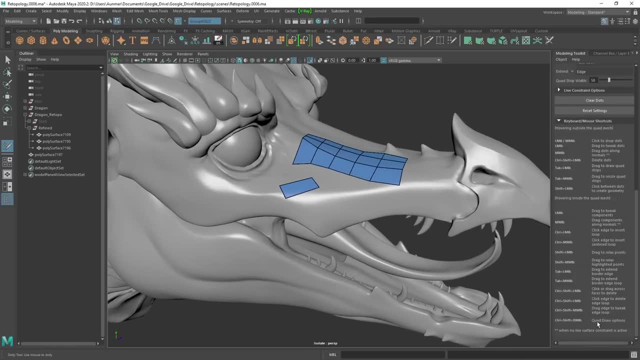 click and that'll just kind of plot a face here. So if you're going through and adding some tools, you can do that. I guess the last thing here is a quad draw tools or options. So if you hold Ctrl, Shift, right mouse button, you can grab these tools here. So as you saw, like I can hold Ctrl. 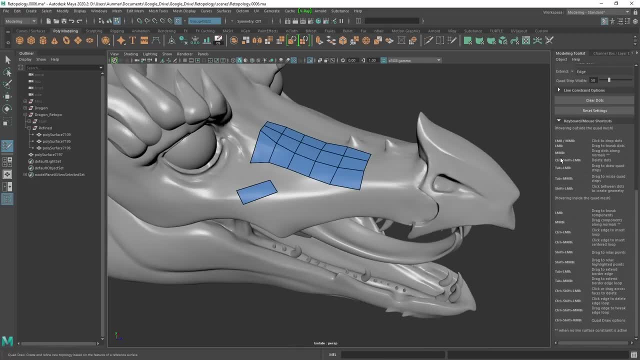 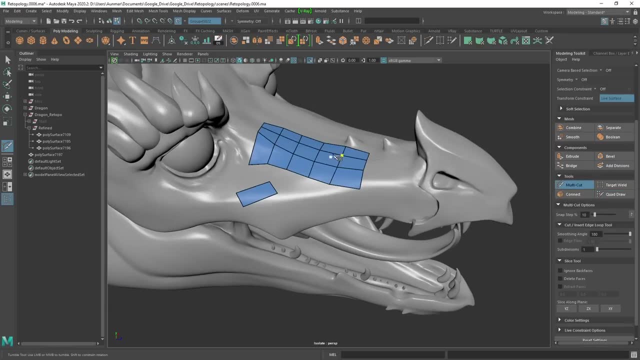 Shift, right click, clear dots boom. Now the one nice thing to keep in mind is you can hold Ctrl, Shift, right click, grab multicut or just simply grab it from the multicut Here, or, of course, hold Shift as you're kind of in quadro mode: shift, right click and grab. 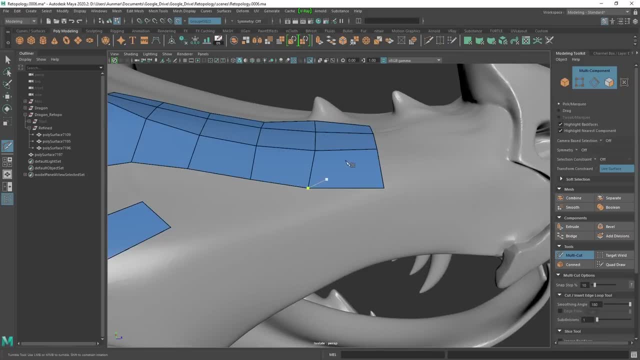 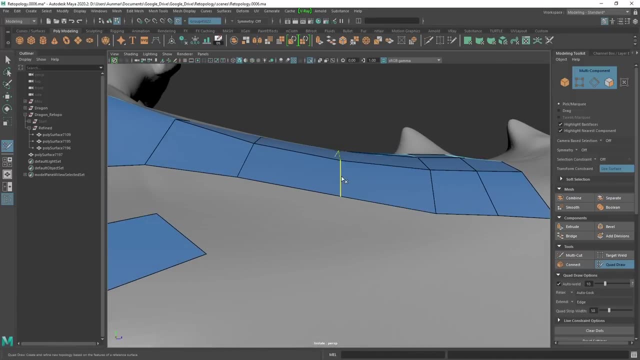 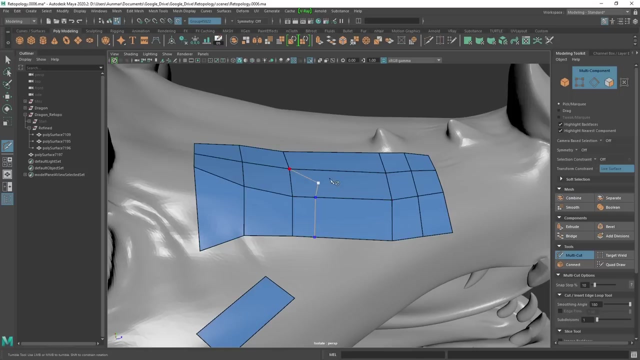 multicut. Now what's nice about this, as you're grabbing multicut, is it will snap to the live surface, So you can see that I'm going in and adding. so if actually I delete maybe this one and then I am cutting in some edges, you simply can do that And it'll add all of these edges. 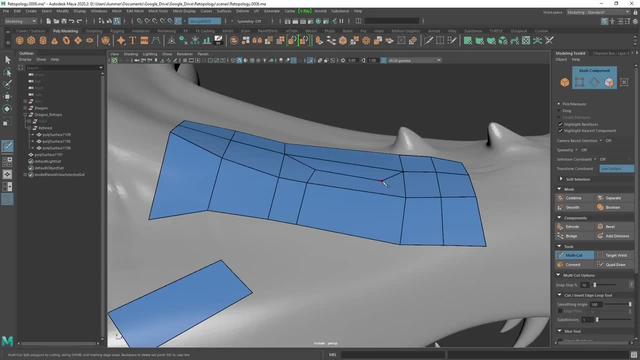 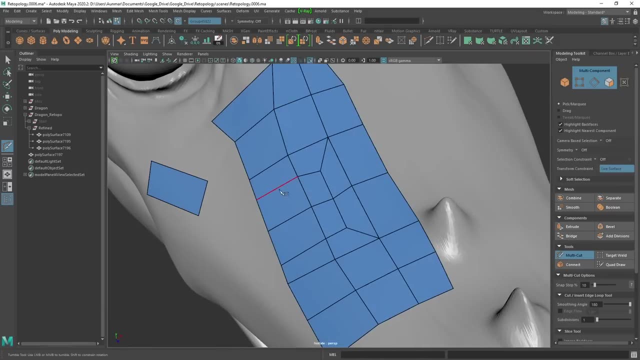 and snap them to the surface, which is really cool, And you don't have to worry about going back and snapping something. So the multicut tool works right within there. So, boom, you can see how that just adds in all of that topology there. 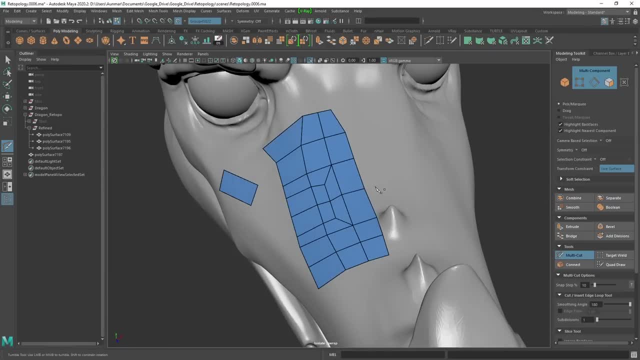 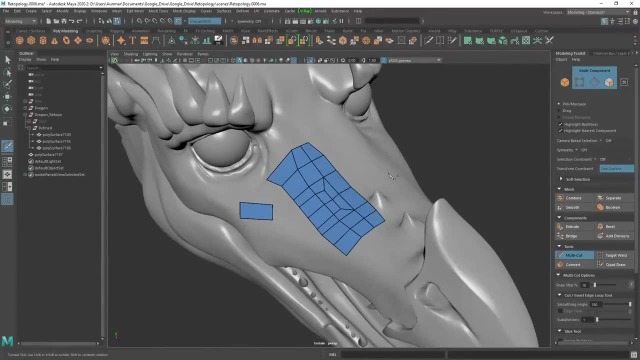 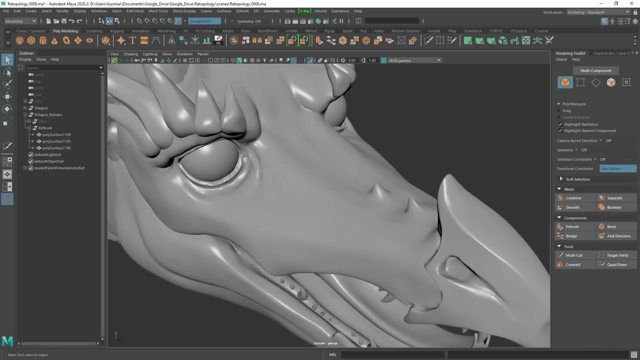 and it snaps it along the surface. Alright, so that in a nutshell- or I would say is a pretty high level- quick rundown on how to use all of the quad draw tools, or the majority of the quad draw tools. Now let's get into the important part, which is edge flow and topology. Alright, 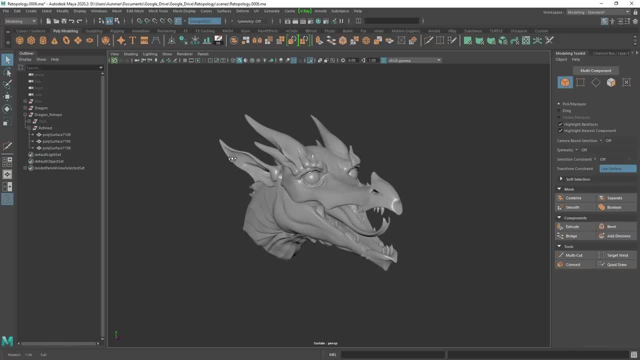 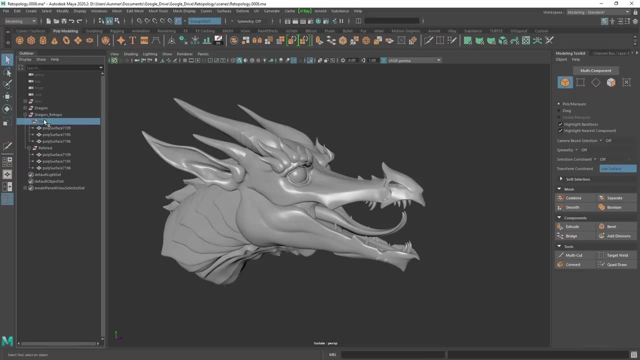 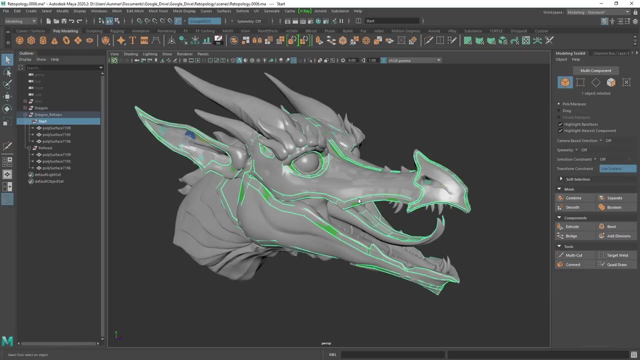 so now that we've gone through and understand how to use quad draw, let's take a look and now really understand retopology and topology and edge flow. Alright, so the number one thing that I can, I can tell you for topology and retopo is if I go ahead and show you this group here. 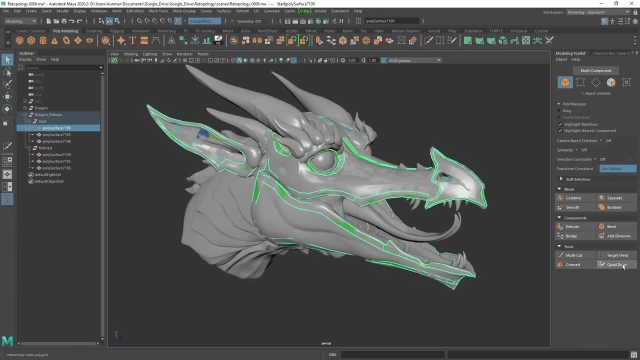 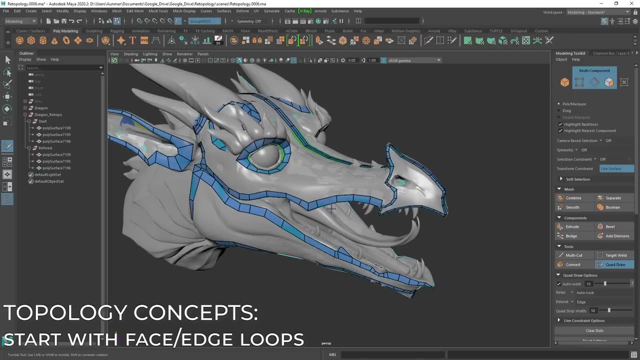 and it's this start group here, And if I go ahead and hit quad draw, take a look at this: The number one tip when starting out and retopologizing your models is to start with your edge loops and face loops first. Alright, you can see here that I've done that. 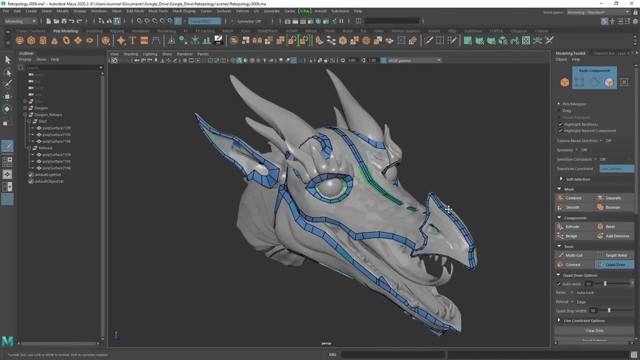 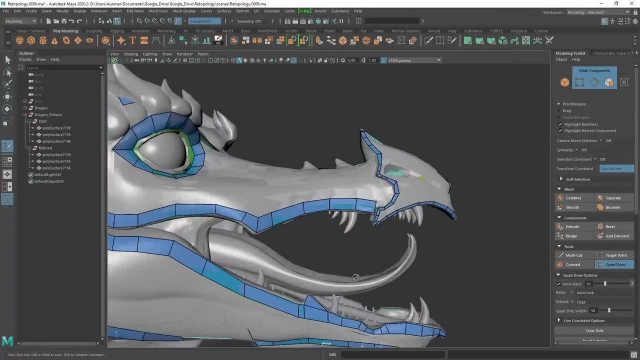 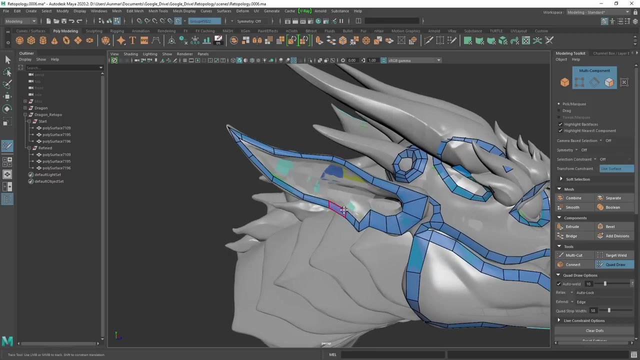 this is exactly what I've started with. everything that you see here in the blue And you saw, you see that I'm focusing on the eye loop, I'm focusing on the mouth loop And you can kind of see I have the horn and nose area here And you know I've gone and worked up the ears. 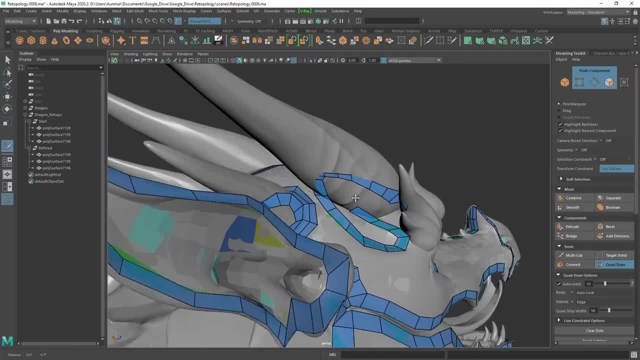 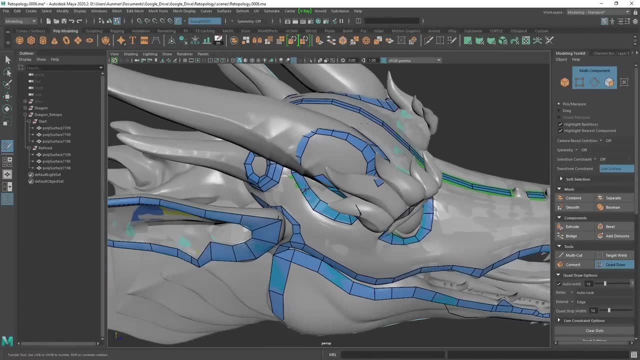 as well, And I'm just kind of starting And you can see all these details here as well. you can see, here I have kind of that skull deformation in there, So I know I'm going to need some topology to focus on that. And then where the horns are coming out right Now, this is a fairly complex. 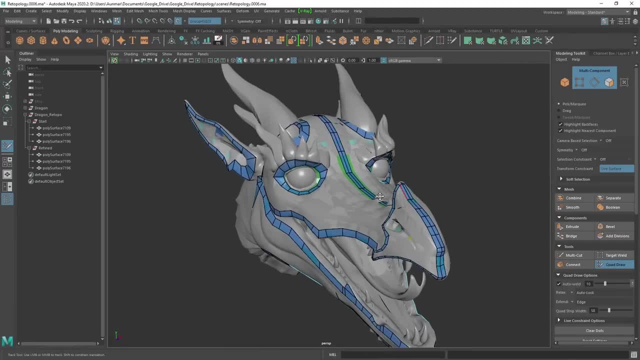 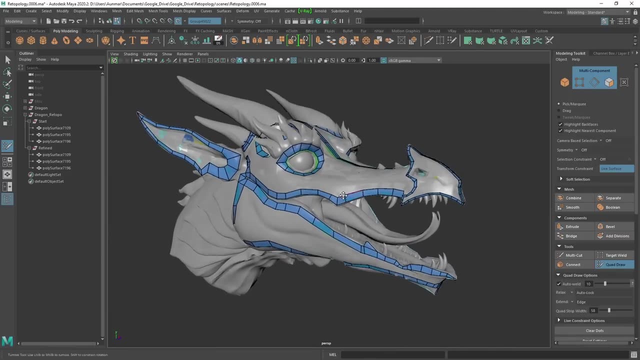 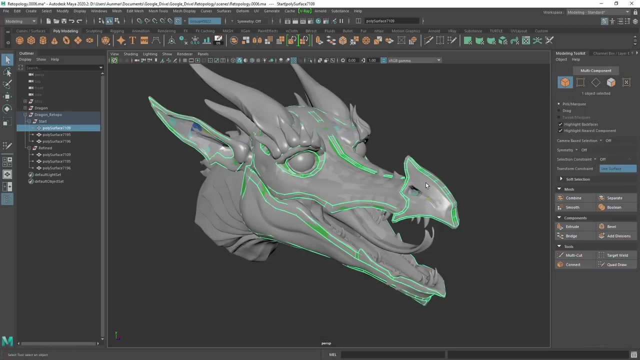 model. But what I'm trying to show you is how you can take these, the simple key concepts, principles and workflows and apply them to complex objects. Alright, So now the next thing you want to keep in mind is: you want to start with edge flow in topology first, All right, And you want to make 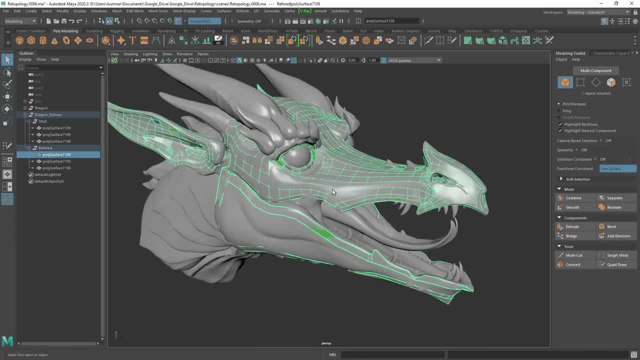 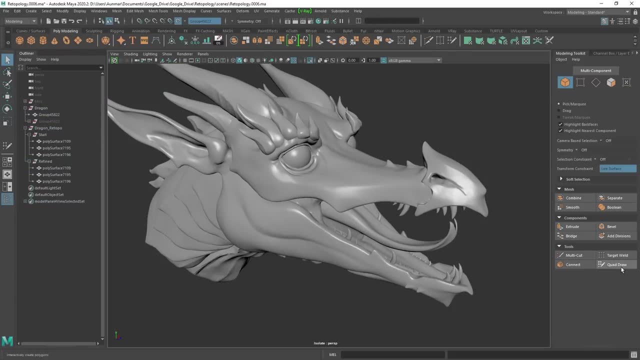 to kind of keep a good spacing of your face loops. So if I go ahead now and drag, grab my dragon here, kind of isolate that And I'll go ahead and enable quad draw. you want to go ahead and, like I said, 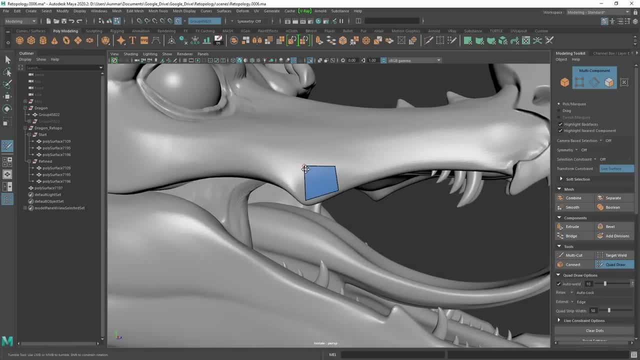 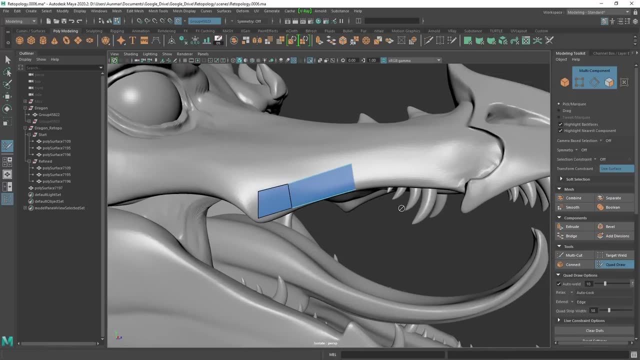 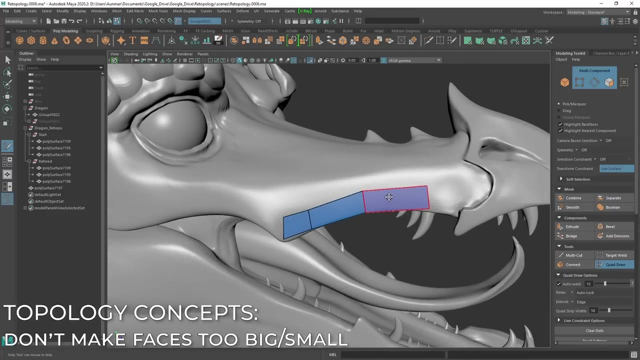 kind of just start with a good distribution of edges. Now, you don't want to go too small. So if our do right now is to start with edge flow and face loops, that don't here is, don't make them too small or too big. right, use kind of your best judgment. Now, what I mean by that is, if I go, 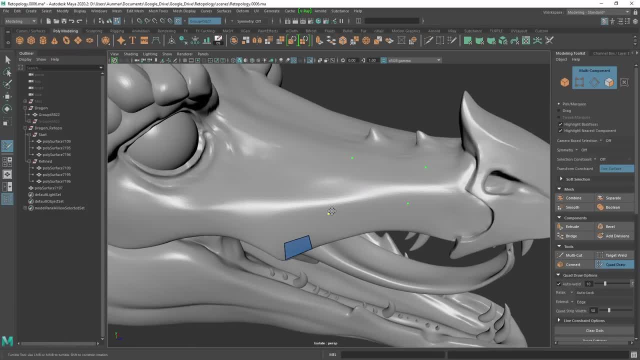 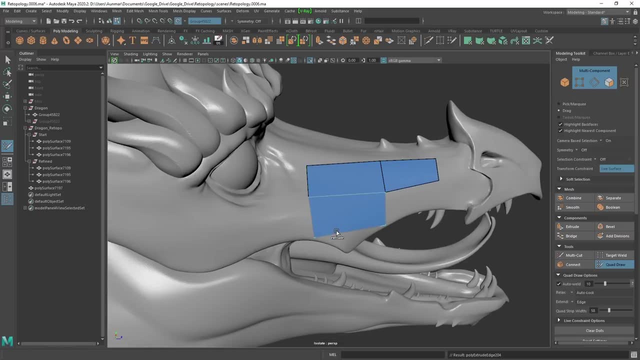 ahead and plot this face down here and you kind of start with this. you can see that it's like: okay, so I'm going to kind of start with this face And I'm going to just start extruding out. right, and we're starting to extrude out and we're starting to cover a lot of surface area here. 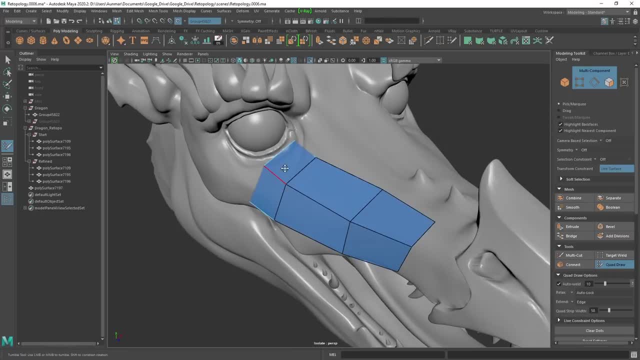 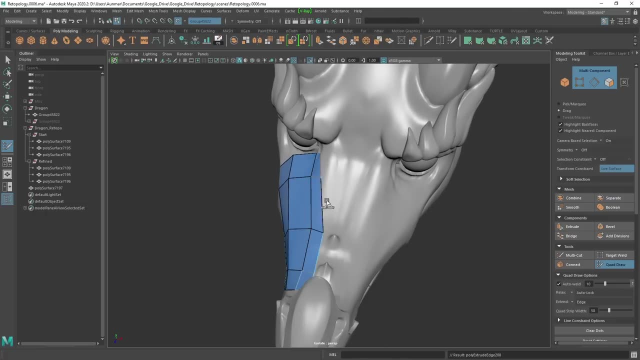 But you're going to eventually reach a point where you're like, okay, well, I need to add more detail there And I need to add more detail there for the nose and then the eyes, eye. how do I go about that? right? So I see this a lot when students are starting out. 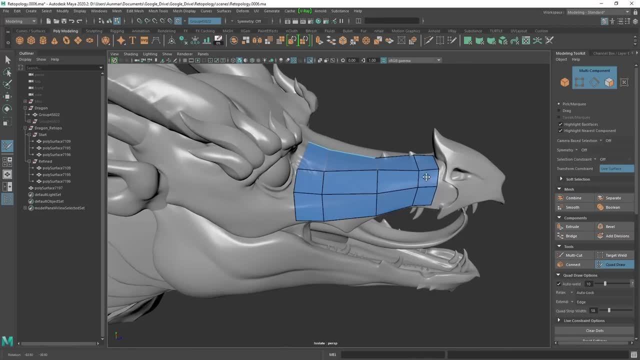 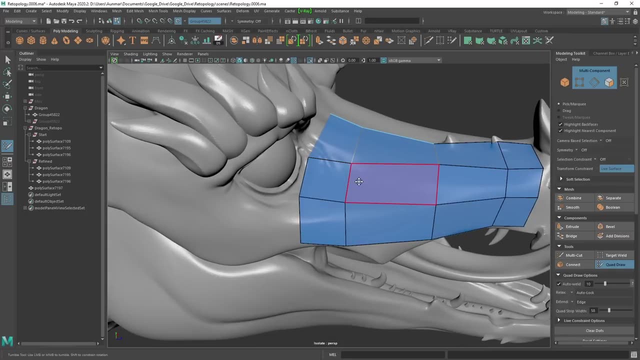 they just kind of want to cover the the most ground as possible, right? And then when you do this, this is setting you up for a lot of challenges: to have to cut in manually, which is the complete opposite of using a tool like quad draw, right, you kind of want to just use multi. 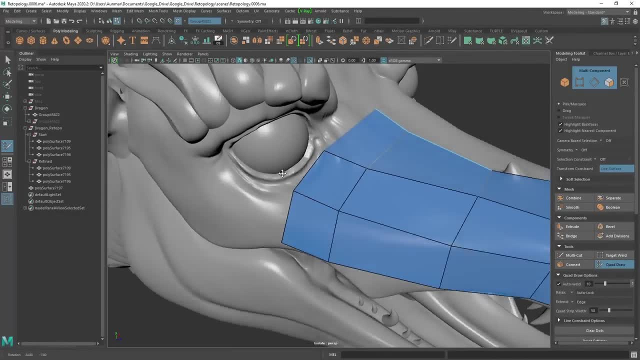 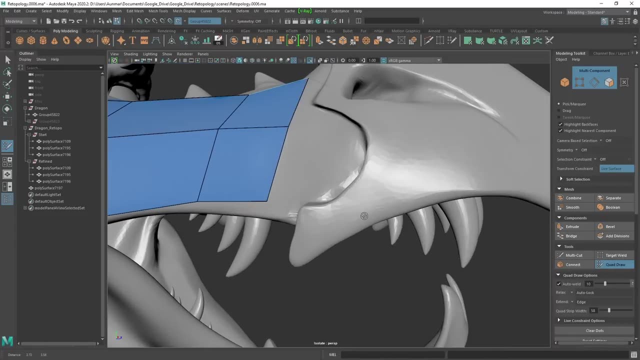 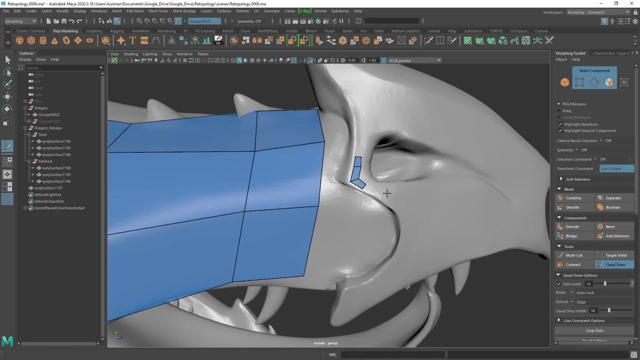 cut towards the end, as you're finalizing rerouting edges right And now on the opposite end is: if you got something like this, then for something that's even like kind of detailed here you're starting with really, really small faces. okay, So think about it. as you know, time is money clicks as money. 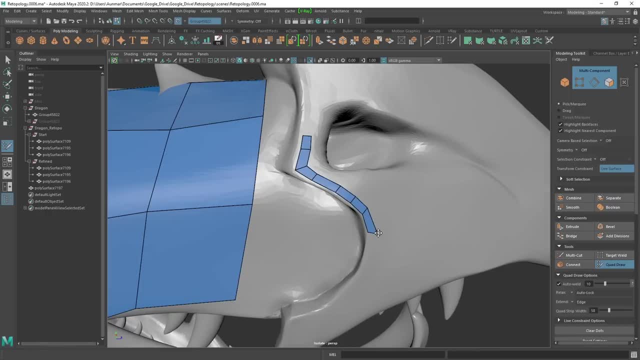 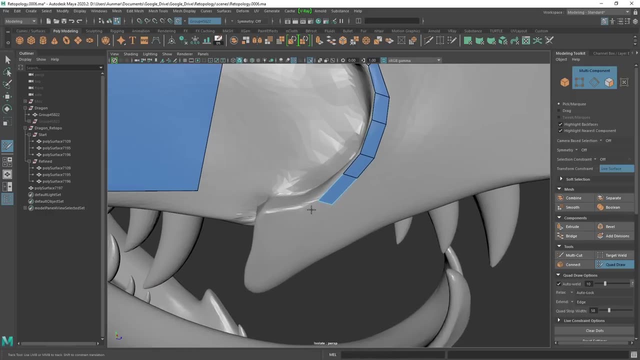 and just the amount of effort that you're spending here working on, you know, retopo, when your models, if I'm going in here and just adding, adding, adding, every one of these edges that I'm adding is essentially more, more clicks right, And not even from a timing standpoint but from a 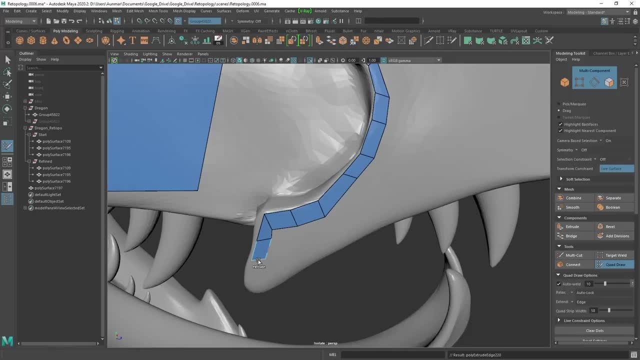 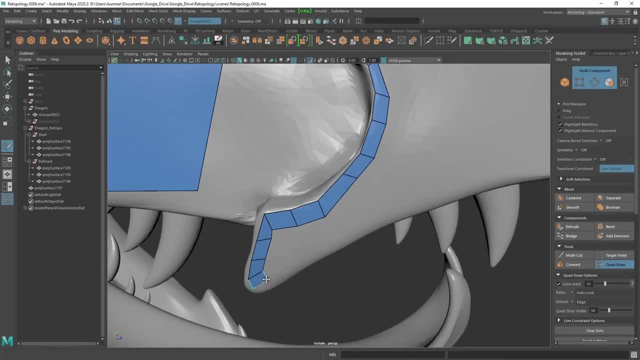 now it's just way more to deal with And I'm just kind of creating a lot more problems or a lot more to worry about down the road, right? So you can see how I'm adding this And sometimes you don't even notice you're doing it. you're so zoomed in you're like, Okay, let's keep going. 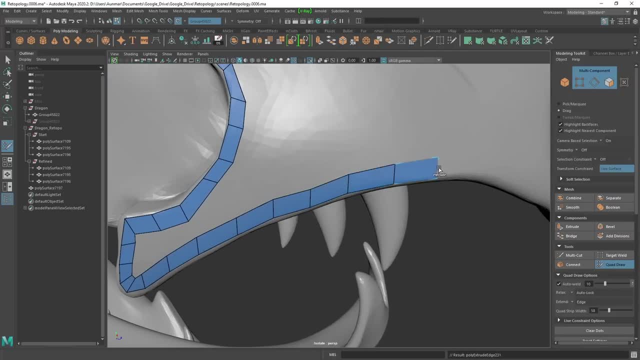 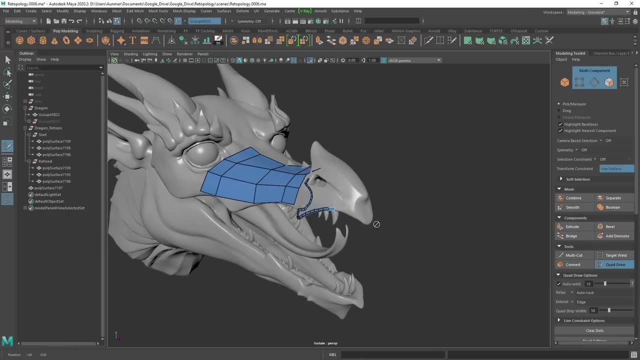 let's keep going. And you're just adding geometry, adding geometry, And then you zoom out and you're like, Oh crap, Like I've added way too much detail here. I don't have enough detail here. Do you want to keep a good high level view here, right? So if I'm kind of going, I mean 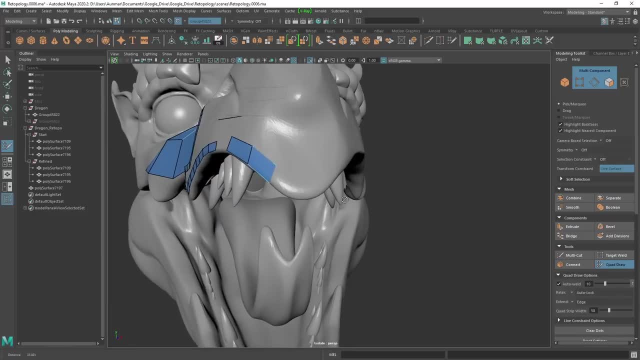 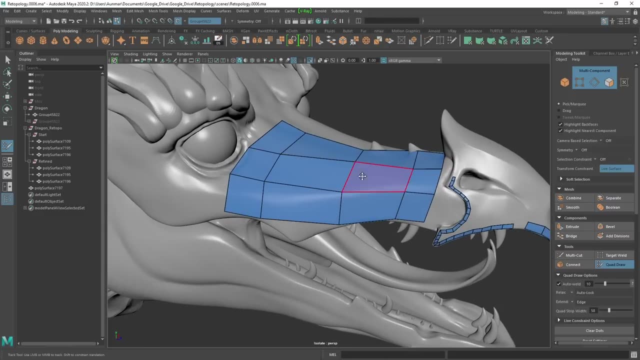 I kind of just keep a good, nice, even distribution, you know, and the good thing is you can always add more as you need it. So just find a good happy medium between large polygons and small polygons And depending on the surface of your details, that's definitely going to be. 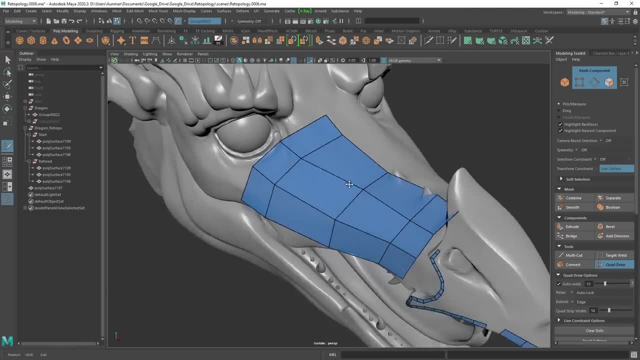 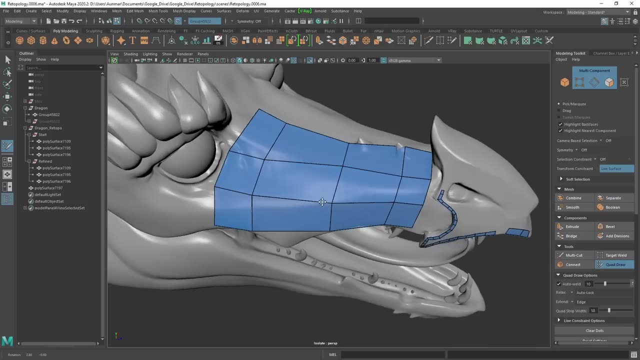 something that you want to keep in mind from the get go. All right Now, now that we understand we're focusing on edge flow, we're focusing on face loops, we're keeping in mind a good size and distribution of edge flow. Now we want to make 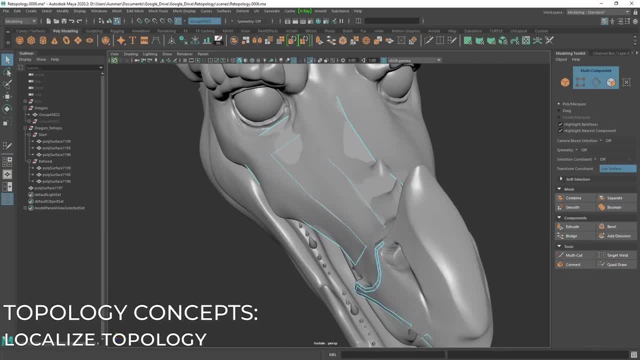 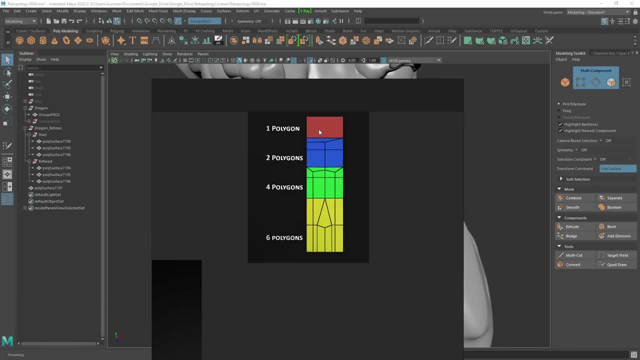 sure to understand how to do what's called localizing topology, which is something that I covered in my last video, right? So I'm going to pull up my pure ref here And you'll see this, this, this image here, this kind of legend that I use, where you're starting with one polygon. 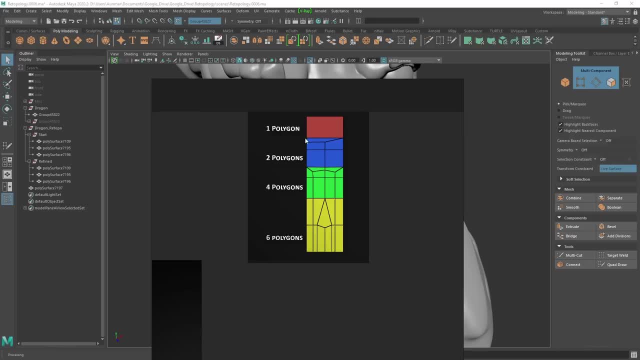 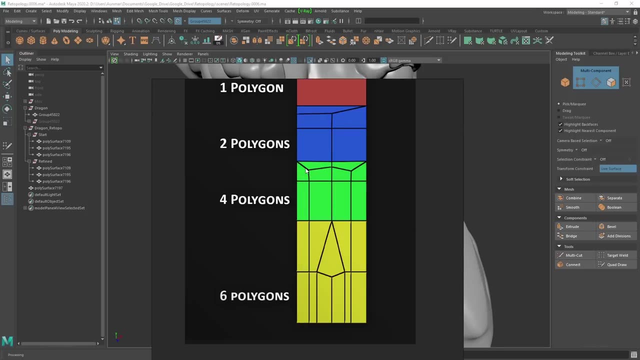 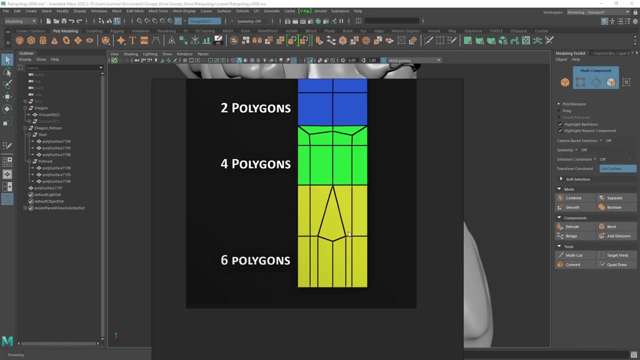 you can take that and convert it into two by splitting or adding this looping edge here, Or you can take that and continue it even further and add four. So by using this method here, where you're kind of adding these faces here which allow you to add two more faces, And then you can take that and split it and add. 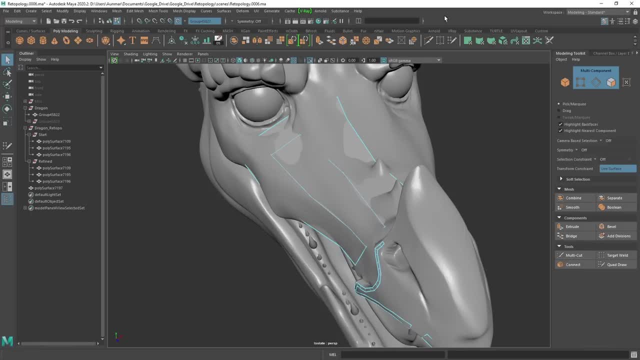 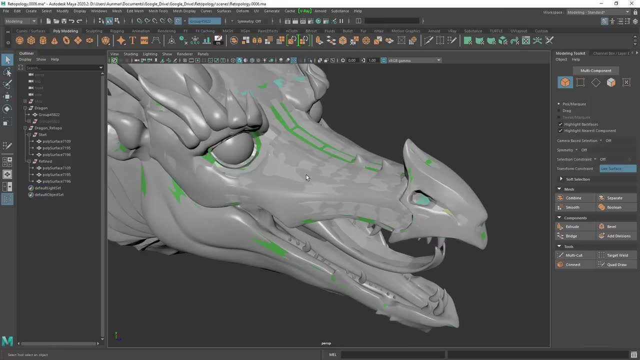 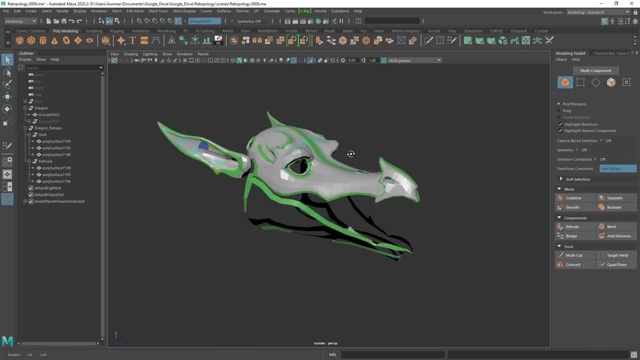 what's called a diamond or a kite quad. Okay, So if I go over here, so I'll go ahead and just simply delete this And what I want to do is show you what I have here, which is this: okay, now, if I go ahead and control one isolate, you'll kind of see what, what I've got here. 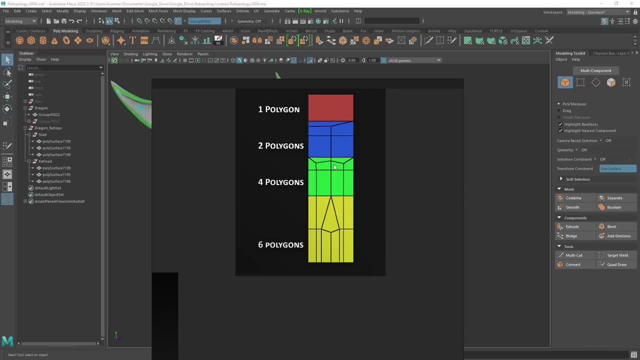 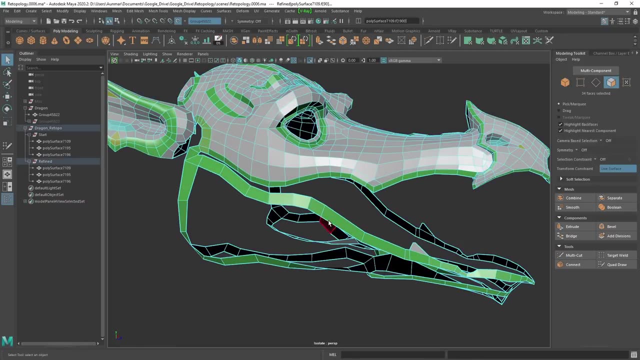 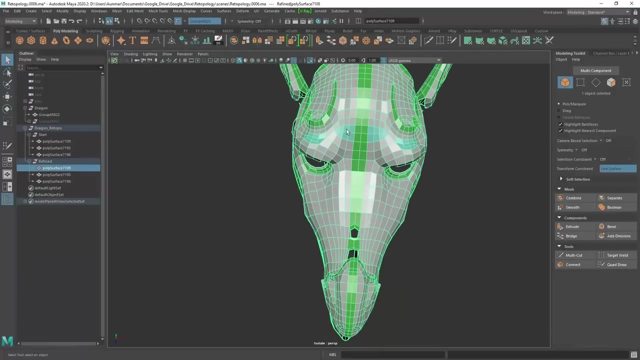 So, based off of this legend, here you can see what I have going on. Okay, so the key thing here actually is: the green faces are my edge loops. These are the edge loops and the face loops that I started with initially. Okay, so I started with these. 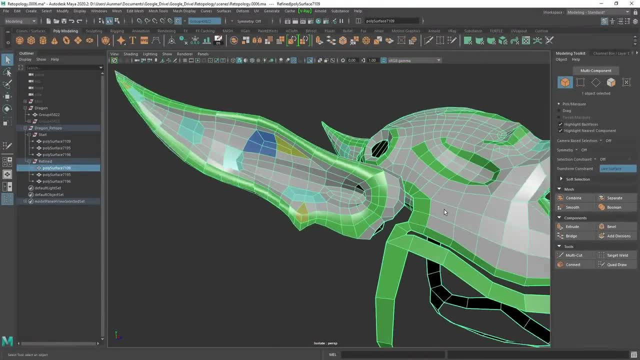 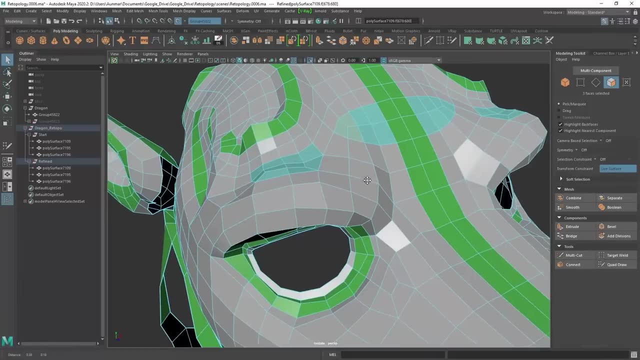 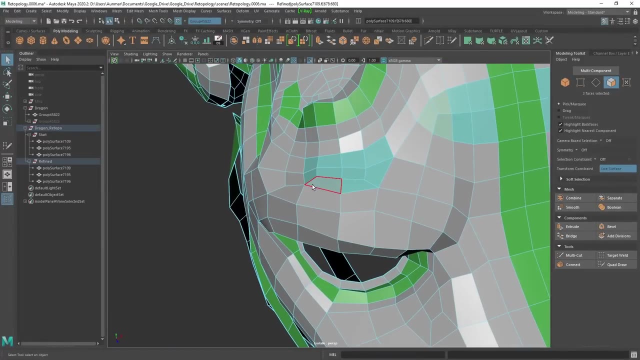 And then you can see that I've gone now and added a lot more detail, Okay, and I'm using things like these kite quads here. So I've kind of highlighted them, As you can see, and I'm using, you know, kites. I'm adding these kind of this two to four. So we're starting with two faces here. 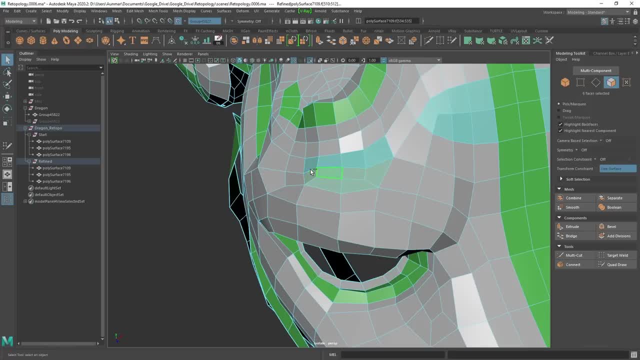 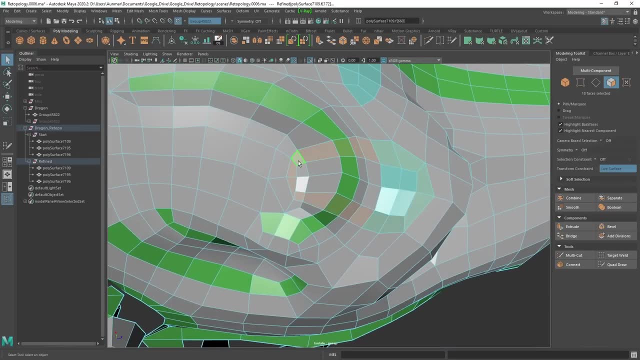 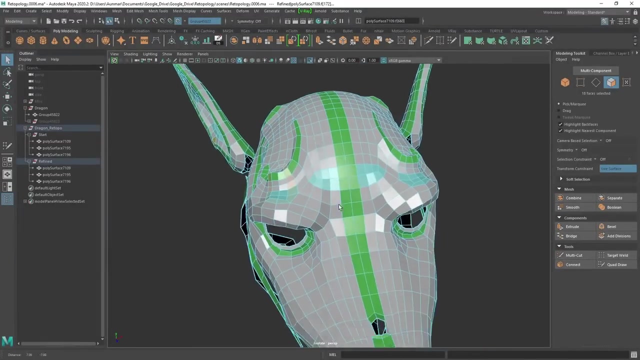 And then we're adding in these faces that allows us to have 1234.. Right, And then that you can see, I can localize this topology and this allowing me not to have and not to carry that topology through all the way through the rest of the skull, And you can see that exactly happening here. 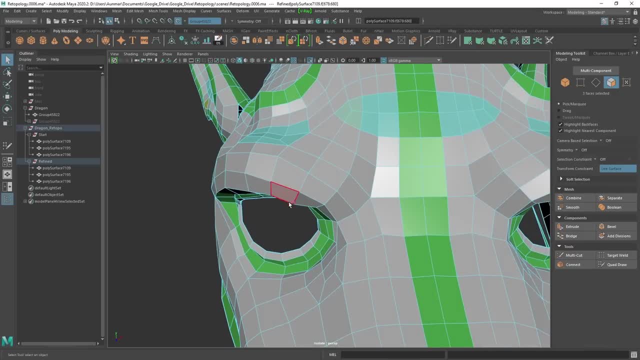 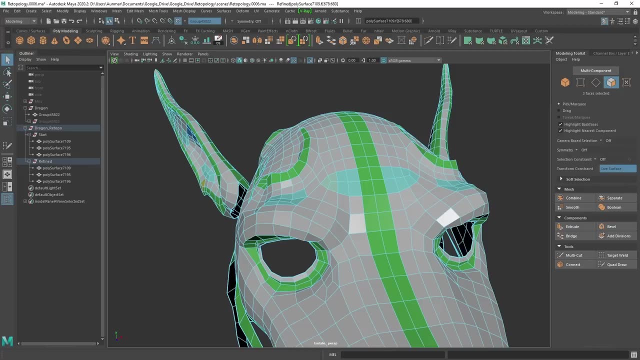 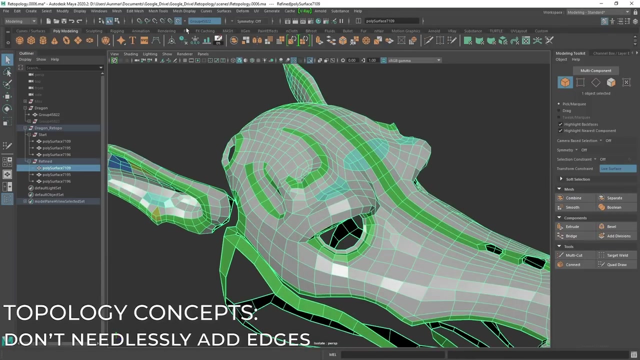 where I have this kite quad here and I just need another edge or two for the brow area instead of having to take and adding in these edges all the way throughout the skull. Right, So, because you want to avoid adding in a needless edges. right, So you can see that I have my quad draw face here. 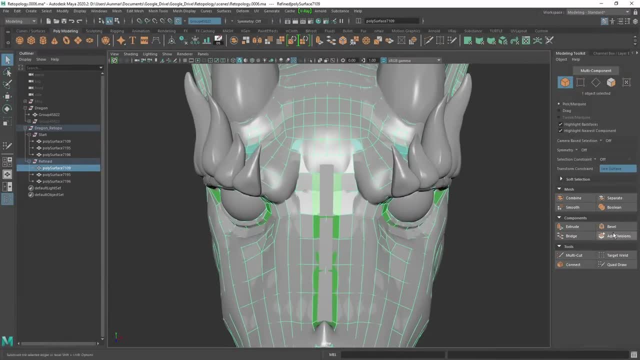 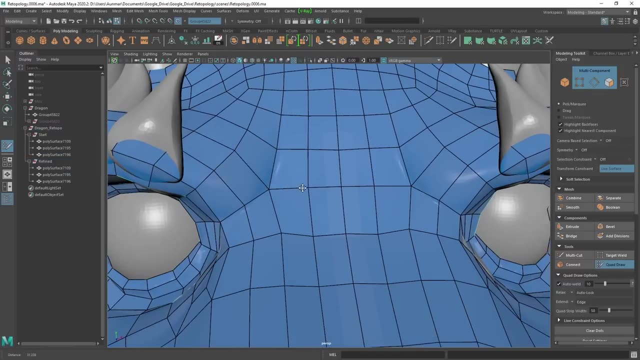 And if I wanted to add some edges, to add the some more detail. I don't want to adjust so you can see kind of this brow area maybe may need a little bit more detail. Well, I don't want to just simply, you know, just start adding in edges like so, because that's just going to add edges. 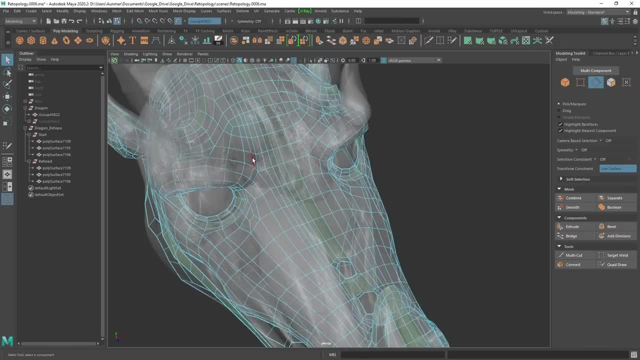 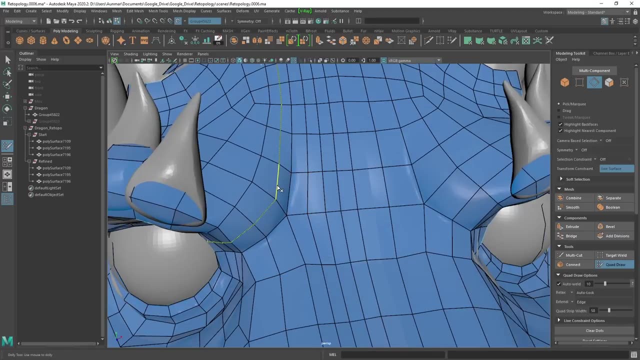 throughout the rest of the model And look how just that messes everything up, Right? So adding these three edges here really, really dirty things up. So I can go in here and I can delete these edges, or by holding Ctrl Shift and clicking those. that's going to help, right? and 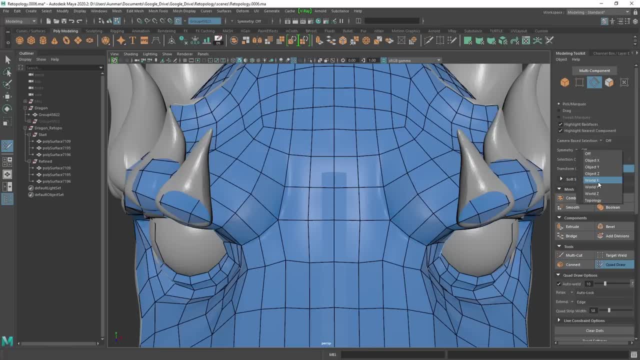 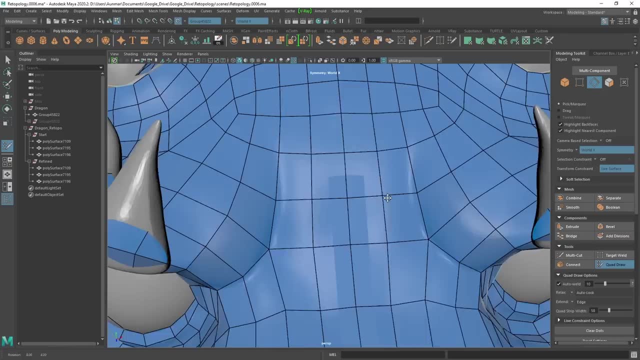 then now what I can do- actually what I always recommend- is to use symmetry with world x here, And you can see I need a little bit more geometry. So I'm going to kind of quickly show you how to do this live. So if I start with this one here, you can kind of see where I'm going. 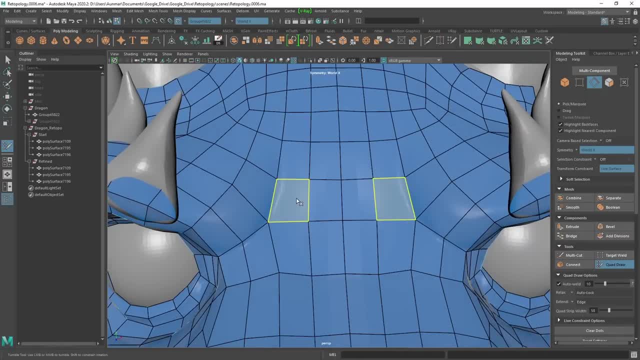 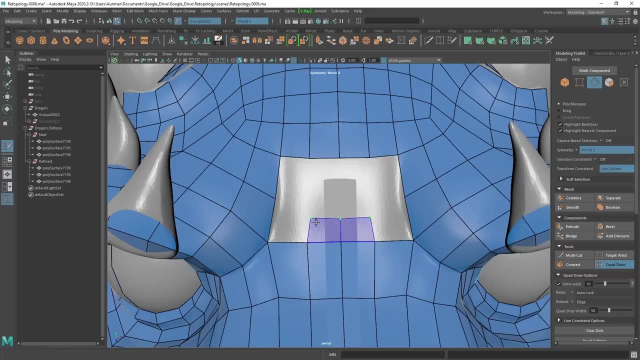 to try to work. So I want to work in this area here to add some more detail on the brow. So I'll go ahead and kind of delete these faces here And then now I'm going to go ahead and add in these faces like so. So watch out. 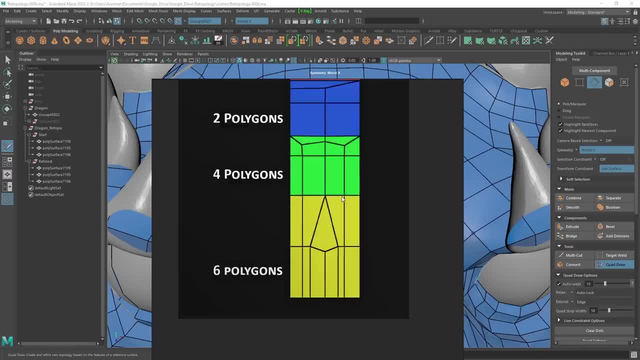 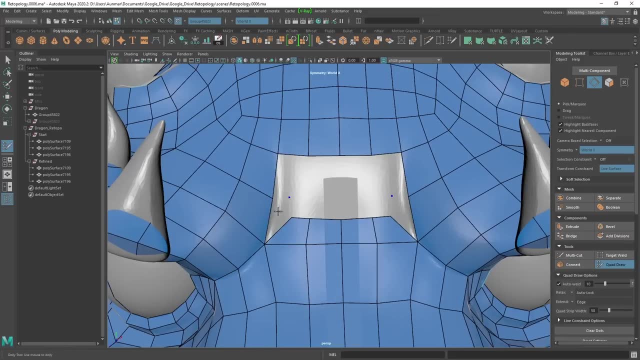 I'm kind of going ahead and starting to add that and the technique that I'm using is this one right here: how to go from two to four. So I'm going and adding in this piece here. So now that I've got that, I can go ahead and start adding in this geometry And we can start to get more of that. 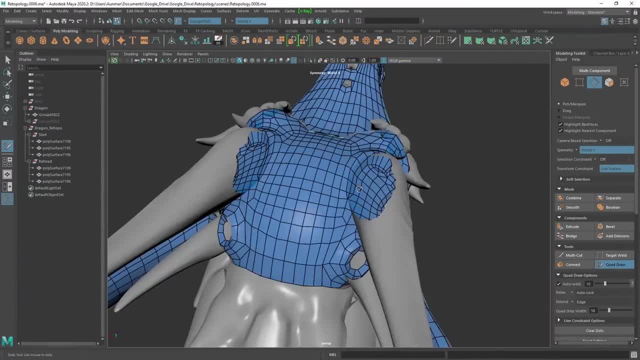 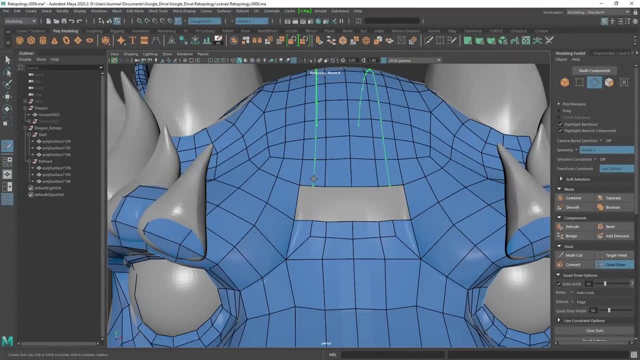 detail here and more of that geometry, And then now you can see I can go ahead if I wanted to add that throughout the rest of the model, So I could go ahead and add it there, Right? and you get something like this And I'm just left clicking to add those faces. 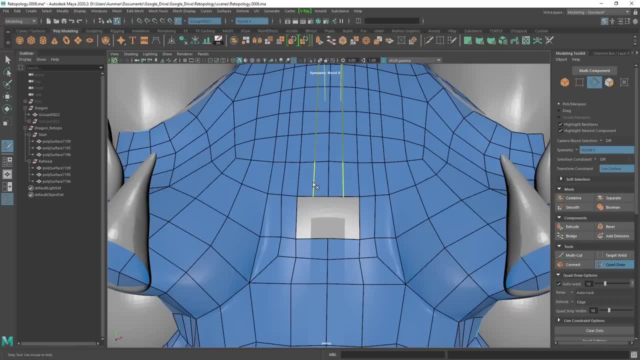 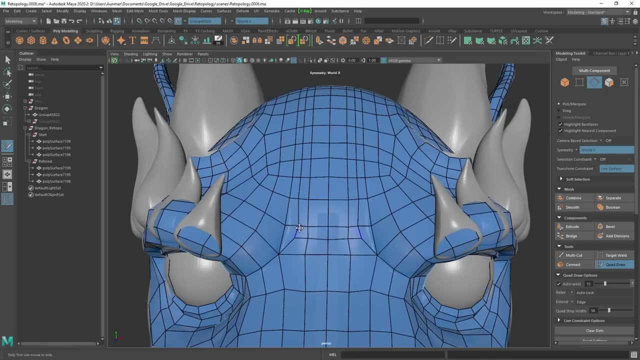 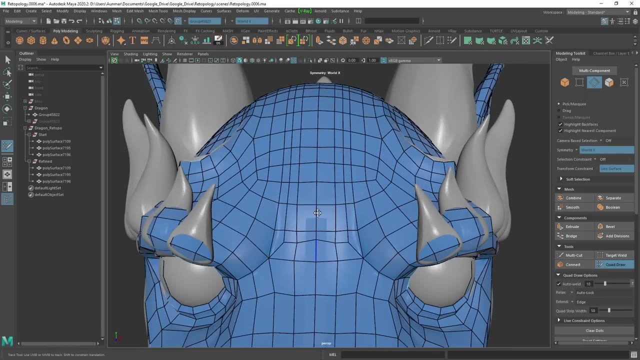 here, And then I can go ahead and remove this one and just go ahead and bridge that across. Alright, so now we get this, which is going to help us hold this brow area a lot better, And I can hold left, click and drag to do this, relaxing that we talked. 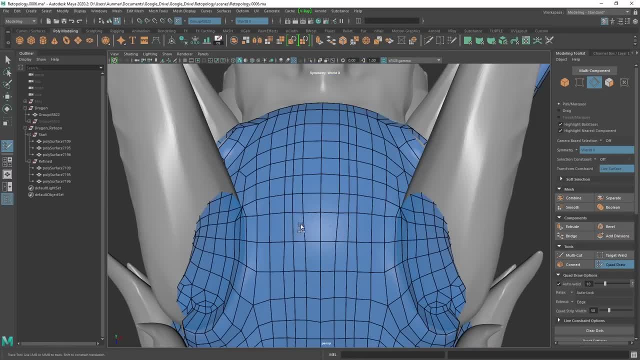 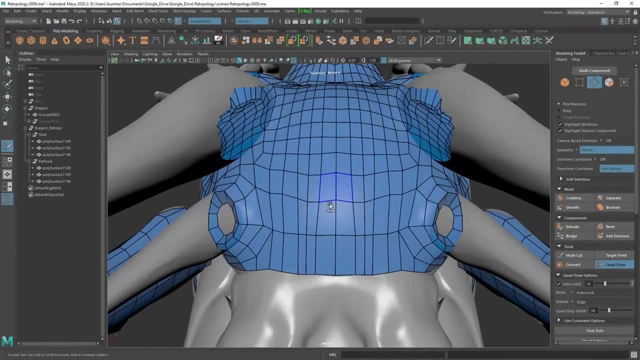 about. So now that's going to help kind of space this out a little bit and give us a nice distribution along the mesh, And so we're just adding in some more form there, Alright. so you can see, with symmetry plus relaxing, we're getting some nice good detail there, right. So 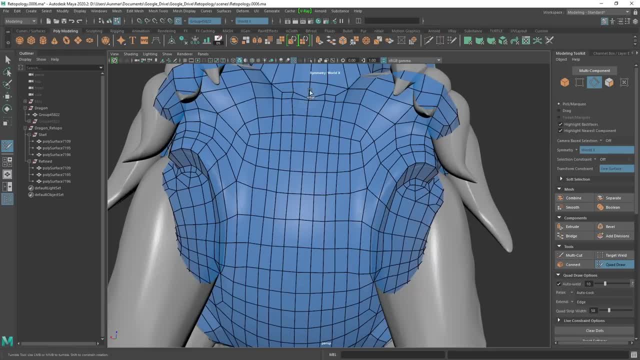 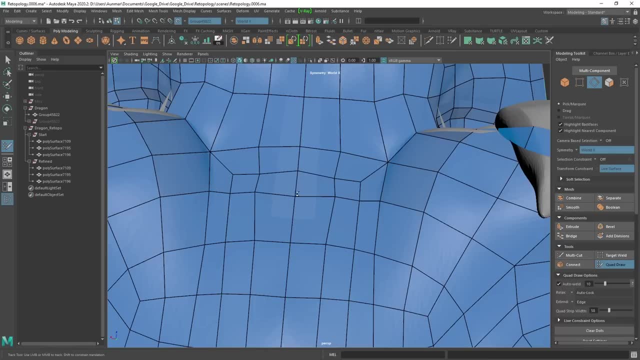 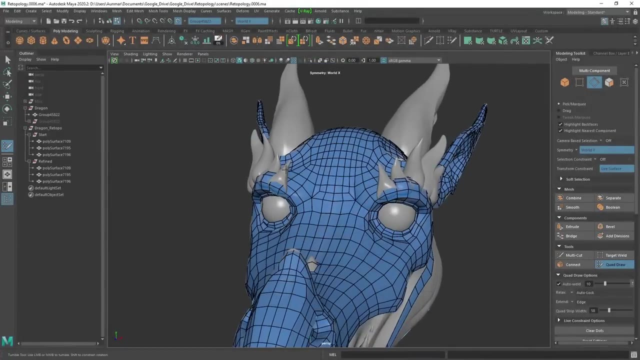 this is just one example of how you can add some more geometry and and route your edges here. So you can see I need to clean up just a little bit here. Sometimes it acts a little bit weird, but there we go And there you are. So you can see how I've, how I've done that. Now, even though this dragon is a 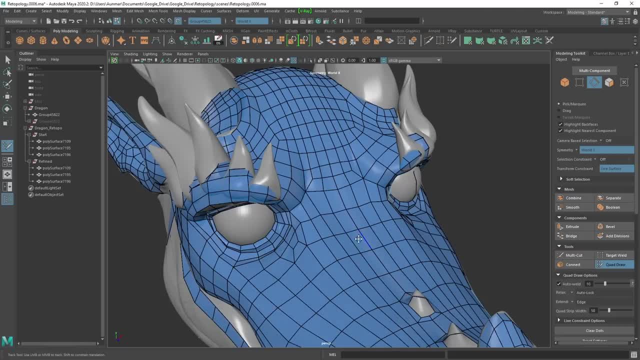 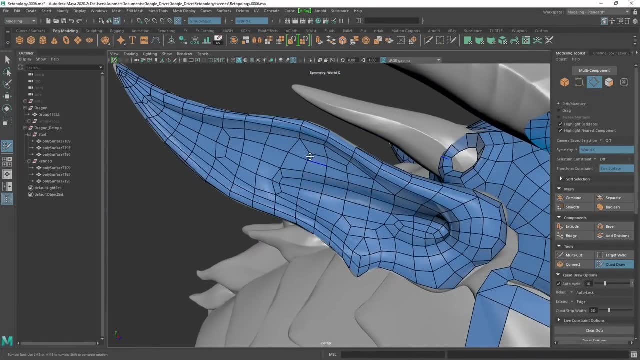 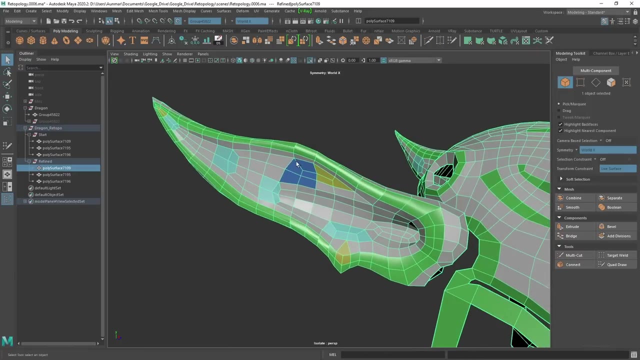 organic model. these techniques can be applied to hard surface examples as well. Okay, so now if we take a look at this ear, I think this ear is a perfect example of this technique in this workflow, right? So if I go ahead and isolate this ear, you'll see. you know something very organic here. 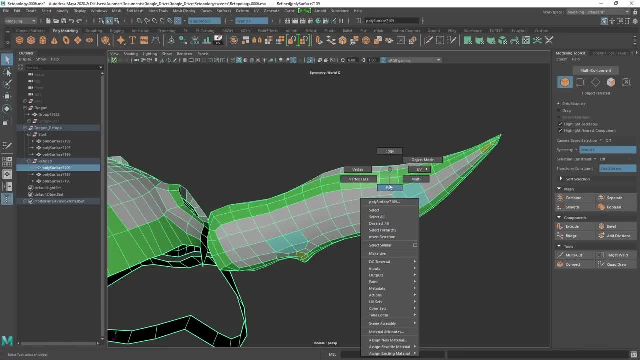 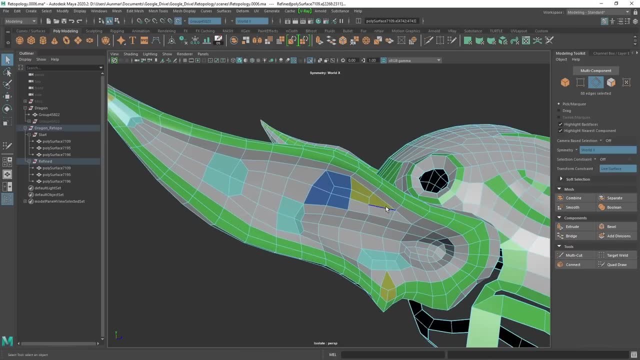 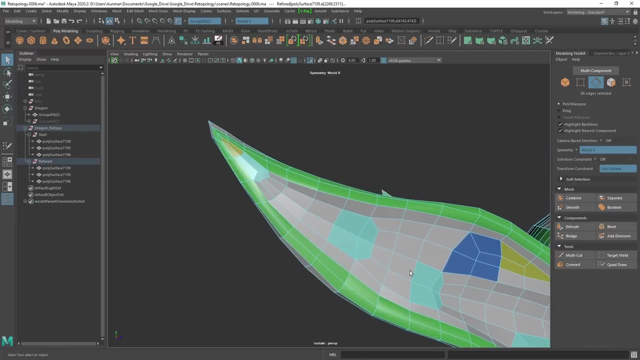 So I'm showing you the green edge loops, So the face loops here. so these green face loops are the edge loops that I started with And you can see that you're going from a lot of detail here. we need a lot of edge flow and topology and polygons. 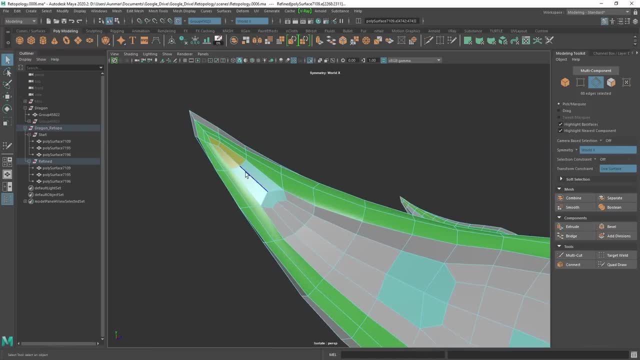 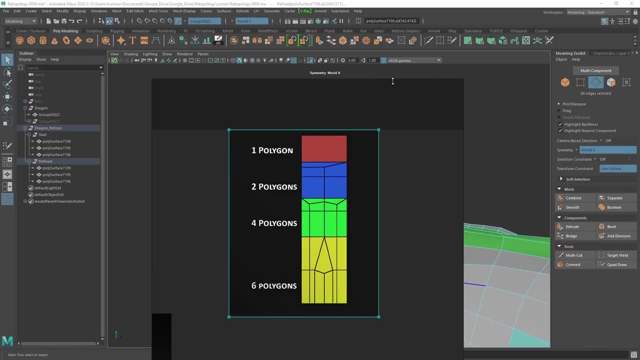 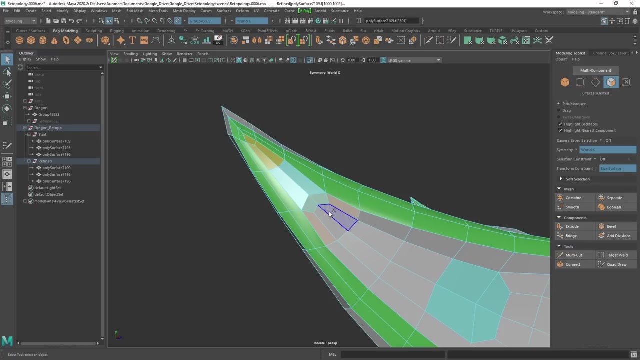 but it ends up here and this very fine point. So you can see, if we go back to this, the polygon techniques, Here we're going from two to four, to six and then back down, right. So you can see, I'm starting here with the two And then I'm adding in this technique here where I'm getting the four. 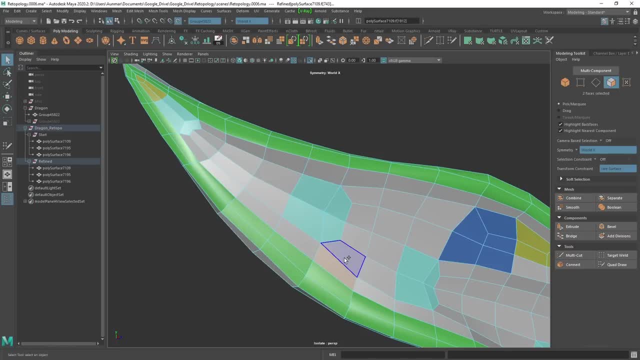 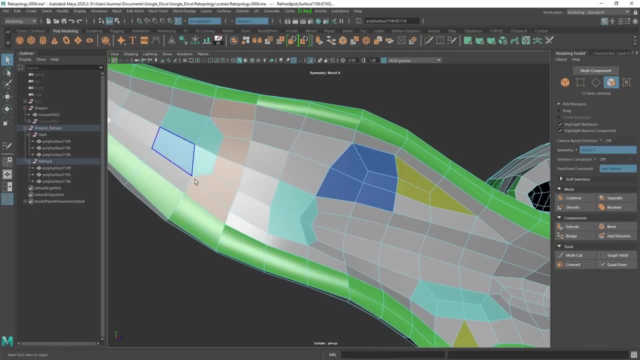 And then I'm doing that again. Right, So I have the four, and then now I'm getting 123456.. Right, And then it's even more right, So I can go ahead and do that, as I'm going for the ear canal here. 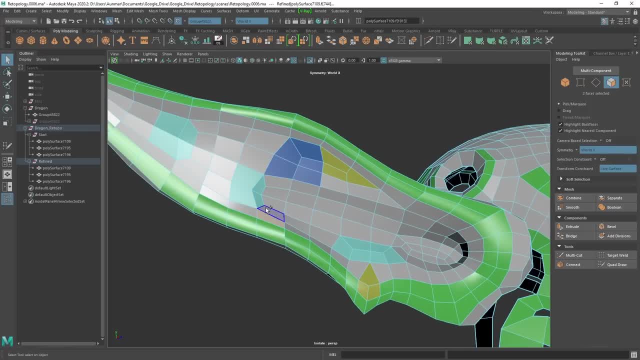 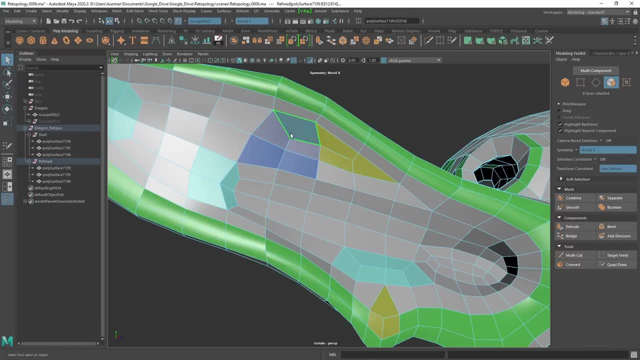 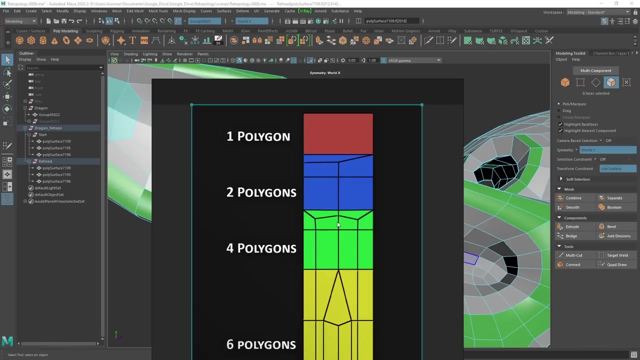 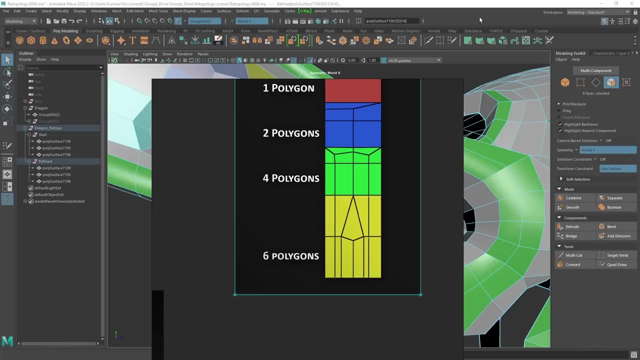 So we're gonna 12345 and then 12345678.. Right, And then this technique here here is this routing the edge that I'm using right here. There's two polygons right about here, Okay, And then you can see the kite that I'm using here, which is this yellow technique here. 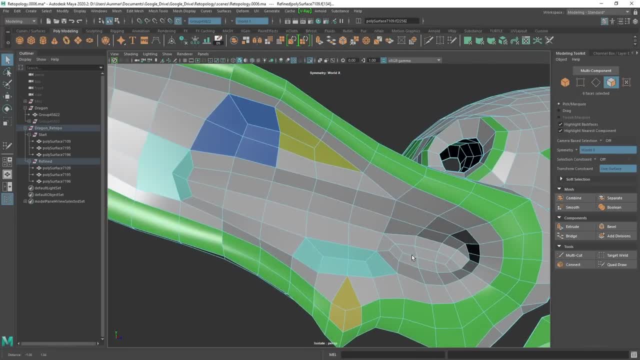 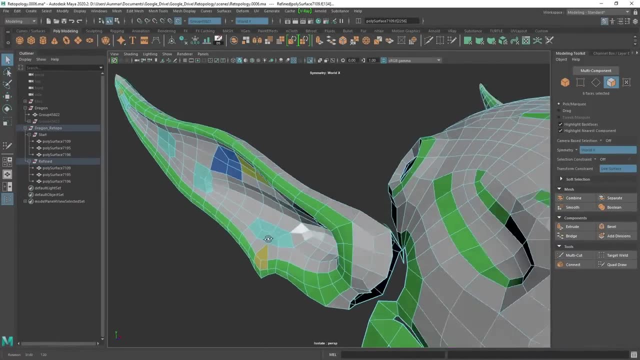 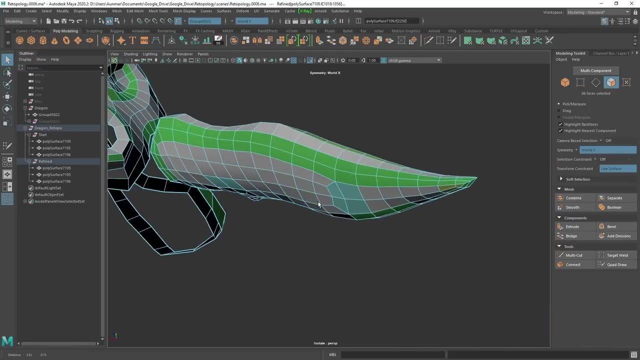 right about here. Alright, so you can see how I'm using that all throughout the mesh right, And I'm using that especially for something as complex and organic, but everything is still, is still manageable, right And is organized. I can select these And you can still see I have a nice clean face loop here. 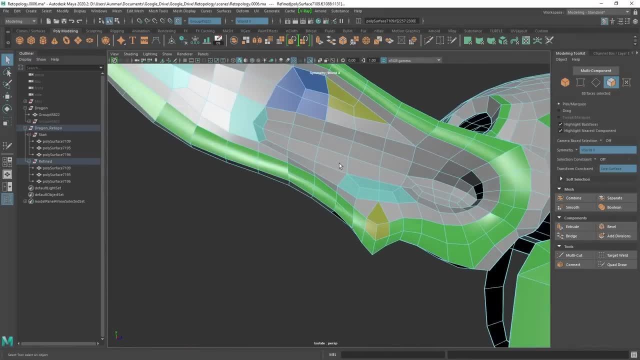 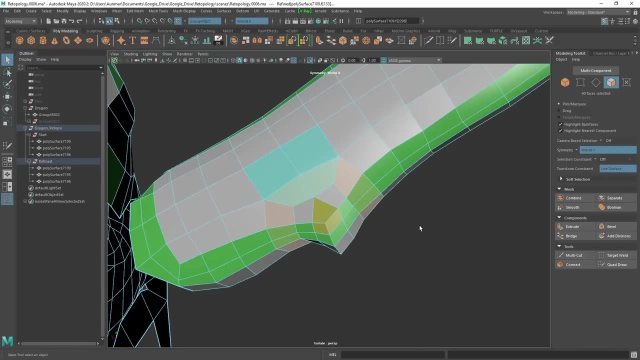 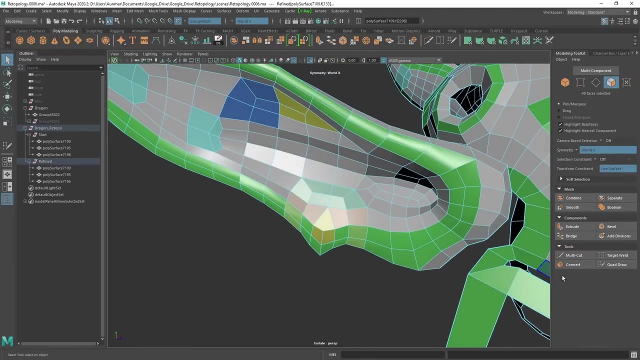 I select this. I have a nice clean face loop there. I've gone ahead and added in kind of this: this routed, this edge flow here, these face loops only in this area. So this is this right. here is a perfect, perfect example of localizing your topology and only adding topology where you. 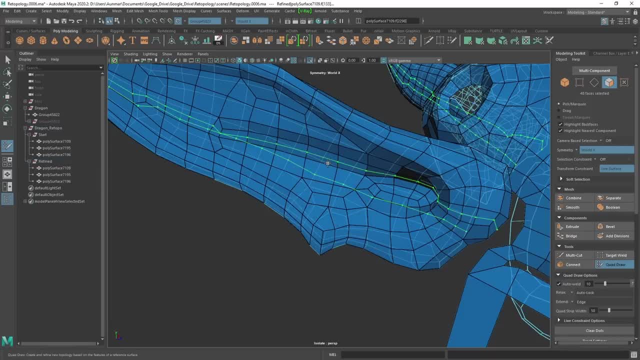 need it. Okay, because I don't need to just continue to route and start adding in things where I don't need things. So I'm just going to go ahead and do that, And then I'm going to go ahead and do that, And then I'm going to go ahead and do that, Okay, so I'm going to go ahead and do that, And 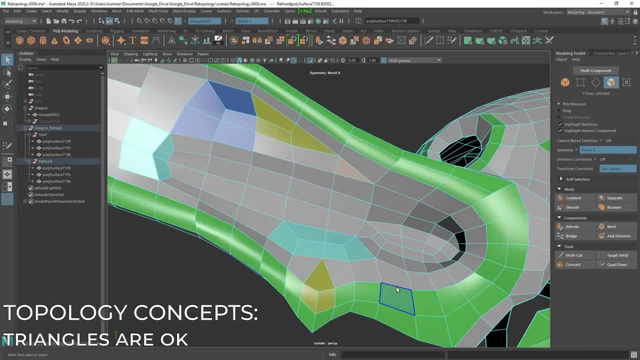 then I'm going to go ahead and do that, Okay. so I'm just going to go ahead and do that. Okay, all right, Because the other thing I wanted to show you is I'm mostly using triangles right Now, in triangles in areas that aren't deforming and for retopologize or low poly. 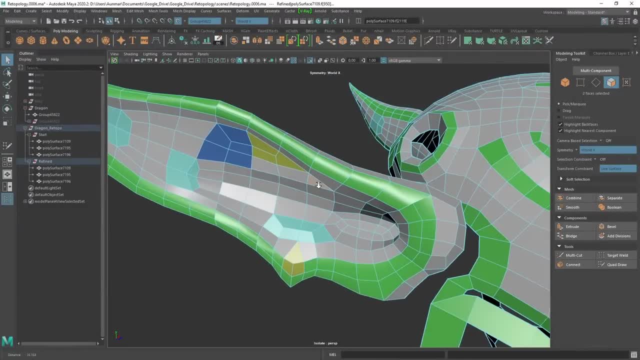 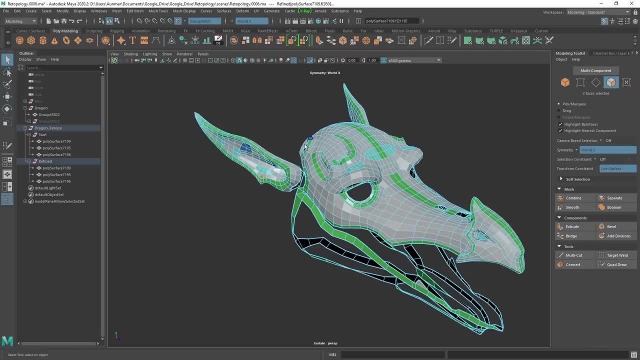 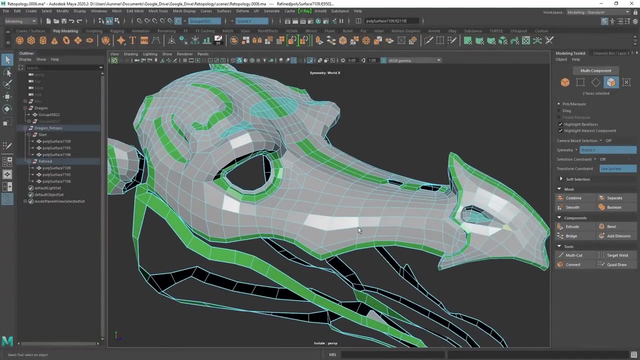 models is 100% fine. You can keep triangles and use triangles as needed without having to add more complexity to your models. Alright, so you're starting to see that being applied all throughout the mesh here And you can start to see. you know, hopefully it's starting to make sense where that's. 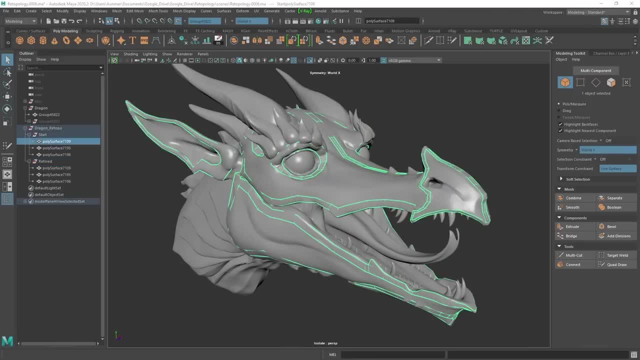 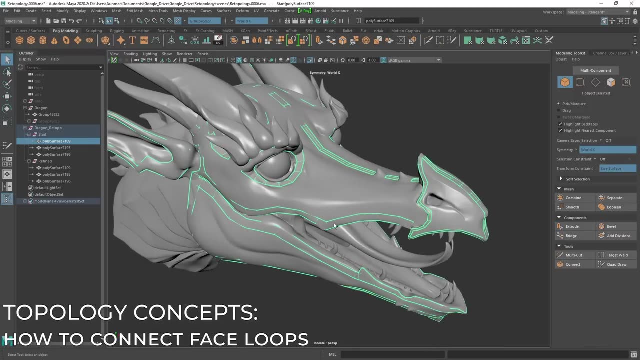 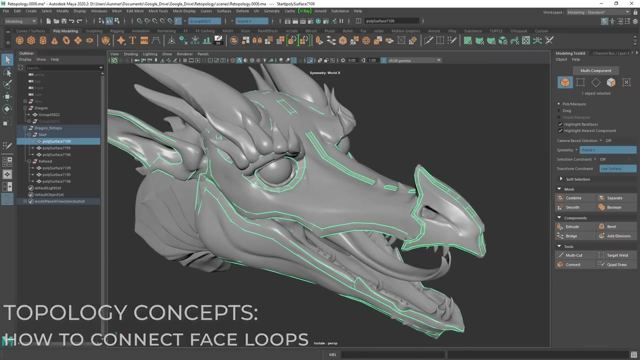 happening in practice. Okay, Alright, so the next step that I have is: how do you go ahead once you add the face loops is go ahead and just make sure to add good, clean, even distribution of edges throughout the rest of the model. So, if I go ahead with, this is the earlier part of the 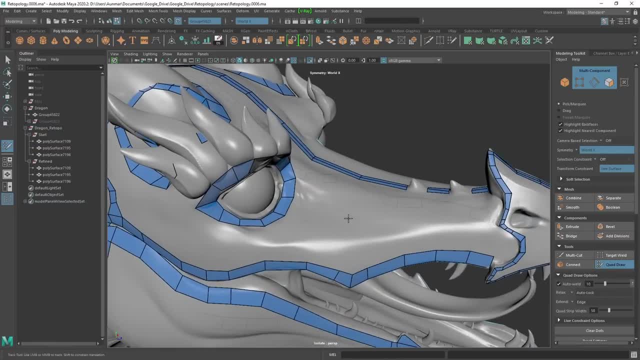 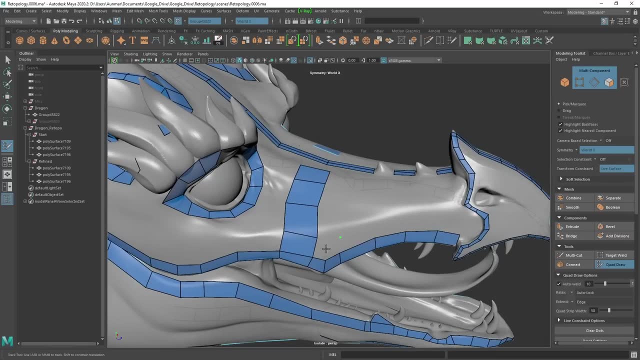 process. So I'm going to go ahead and just quad draw on this part of the model. What I don't recommend doing is this, where you kind of just starting here and then building up and it's just a lot more clicks right And then you can see like if I add maybe some, some geometry here, 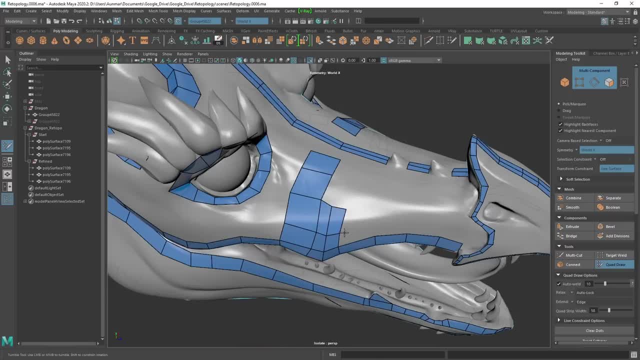 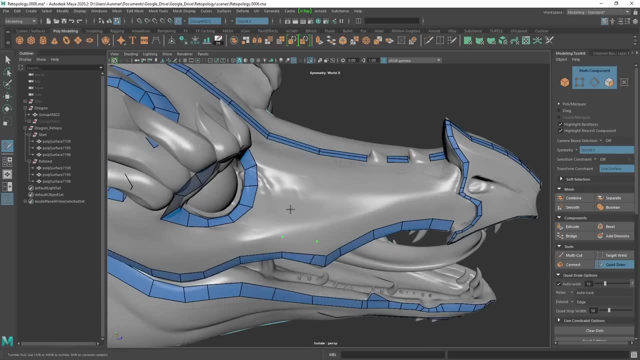 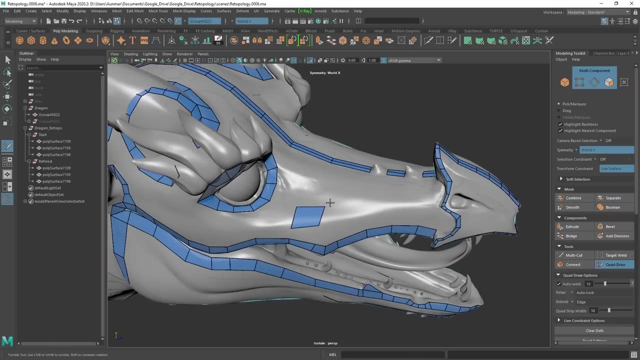 and going up and we're just, we're just adding a lot more clicks. So what I can do, right, if I hold Ctrl, Shift, left click to delete all that is, instead I'm just going to go ahead and kind of add in these larger faces that I know I'm going to add detail to. 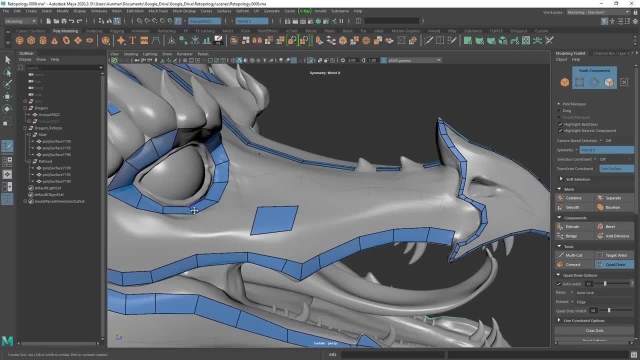 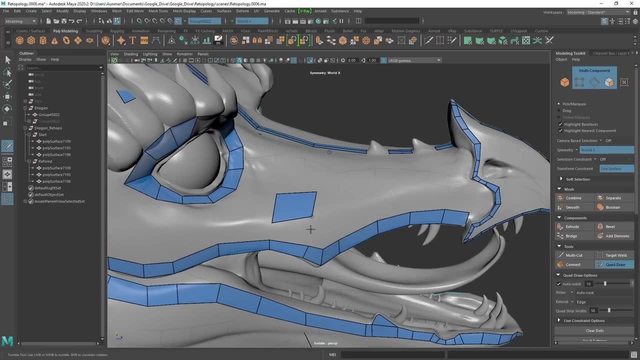 right, And I'm going to want to make sure to match: the end geometry here edges to the end geometry here at the target. same thing going horizontally and vertically here. So I can go ahead and just kind of, you know, add in some of these geometries. 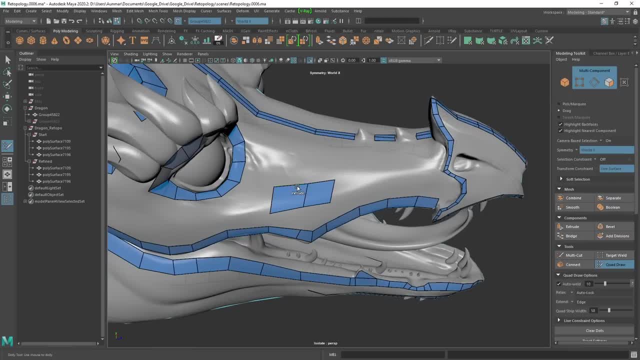 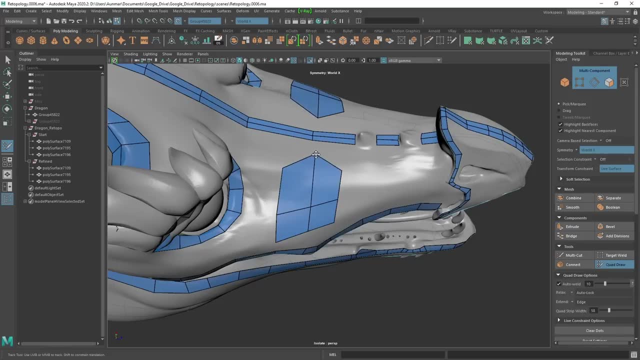 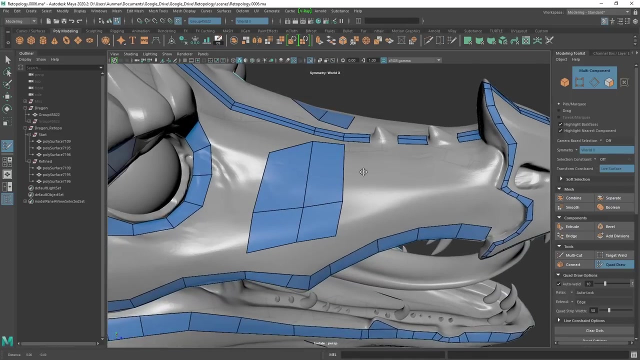 or these edges, And I can just make sure that I have the edges to copy over. I'm using tab and middle mouse to copy these over. So we're going to get something like this here And we can see one to right about here And I can use tab again to get somewhere right around here. I won't merge. 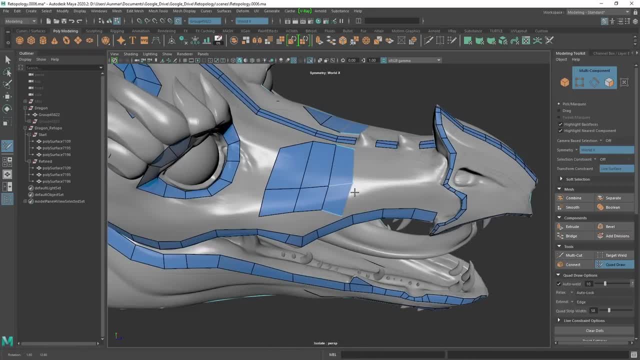 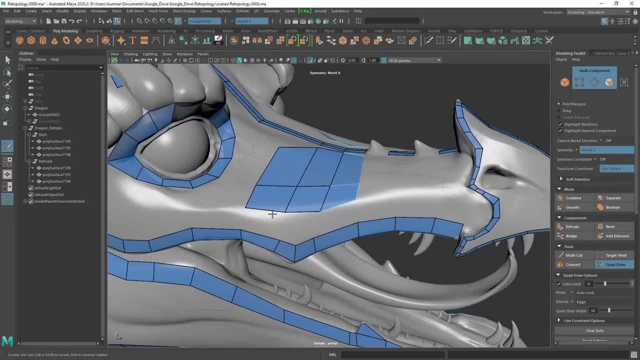 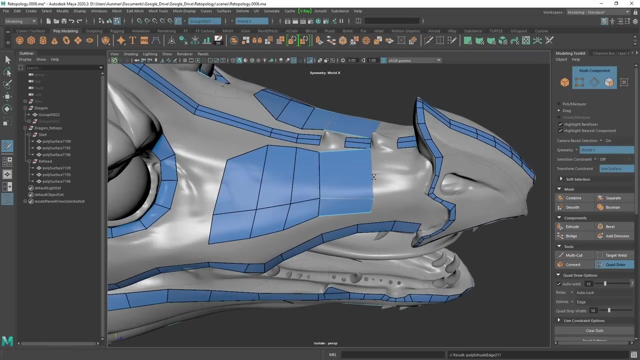 these or weld these. yet Now I want to make sure I'm using a fong and a blend, or a blend, And I'm using the highlights of the object to make sure that I stick with, you know, conforming to the main curvatures of this object, right, So? or our models here, so we can have something like this: 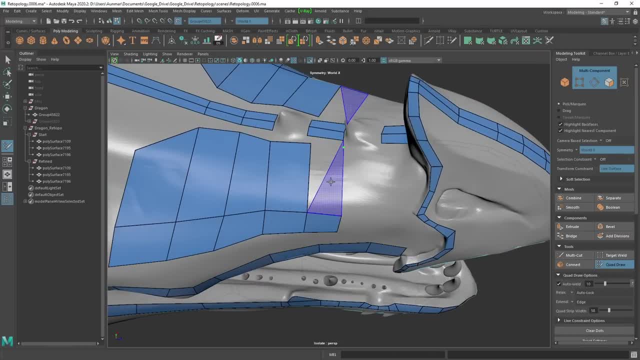 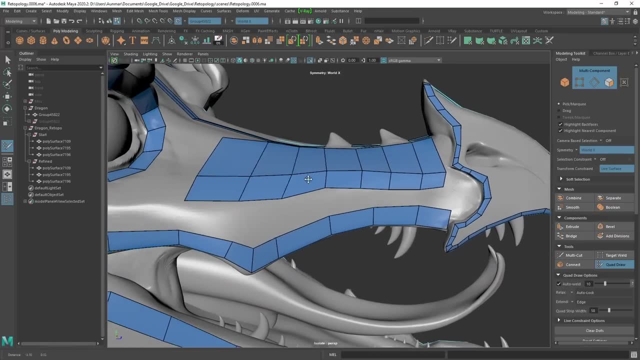 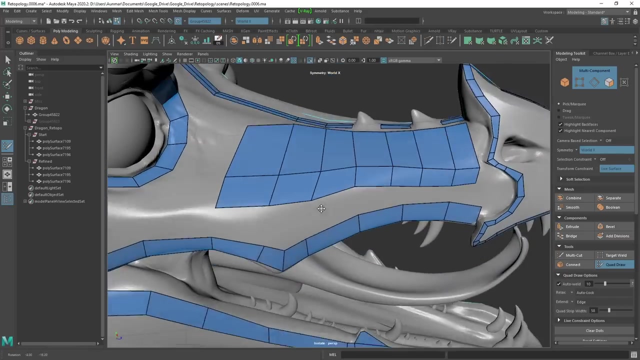 And there we go, Just kind of redo that face there, And then I'm going ahead and just adding that across So you can start to see now, okay, I have a pretty pretty close here. I know I'm going to do like kind of this kite quad effect on this piece here And I want to 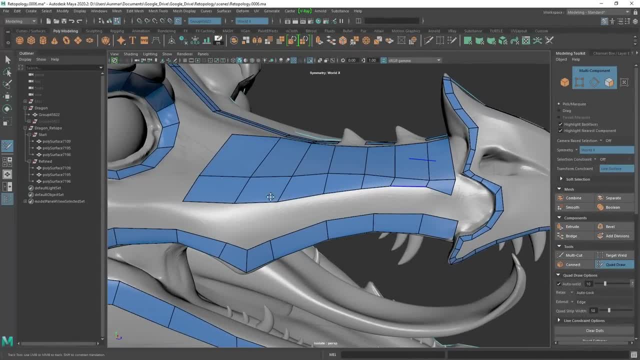 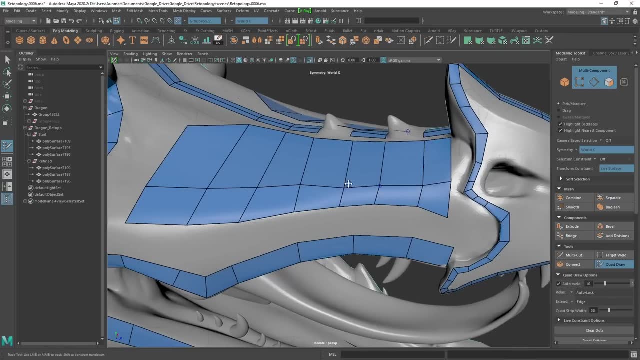 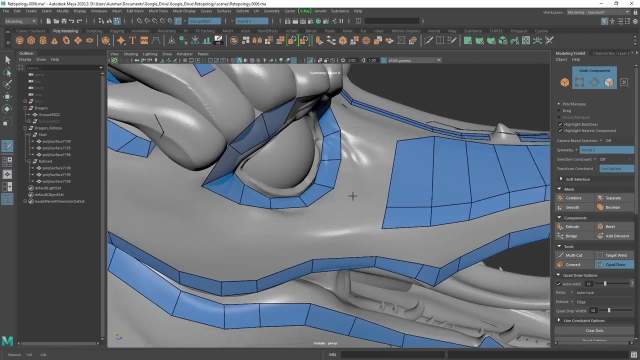 make sure just to kind of match and conform to the surface. I'm looking at this broad highlight here on the dragon And then I'm going to add in another kind of face here or manipulate these vertices here. So there we go, something like this: That's looking pretty good. And then now 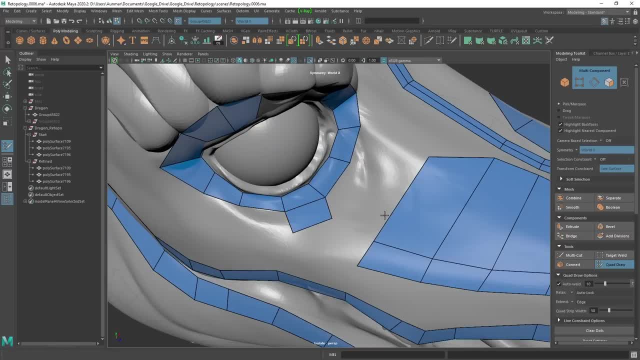 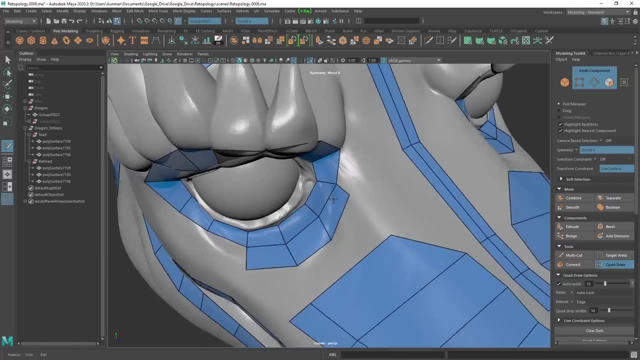 I want to start building off of this I so, if I go from this, I now the orbit of the eye, I can start to kind of come out from there And then I'll start to know pretty close how much geometry I'm going to need to match up between the two. 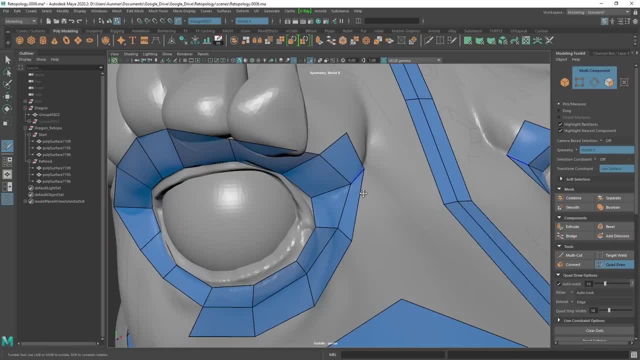 We get something like this. I'm going to keep this one right about here, And I may. it looks like I'll probably have to add one that runs right here. Actually, what I did is added some more detail. I'm going to make sure this part of this case, I'm going to make sure this is also. 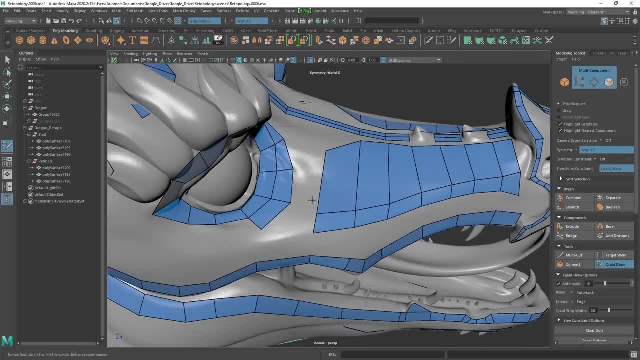 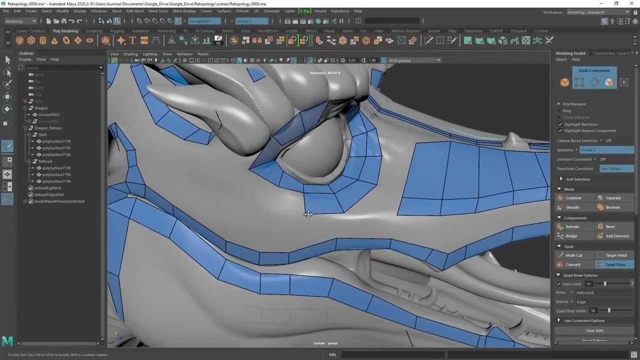 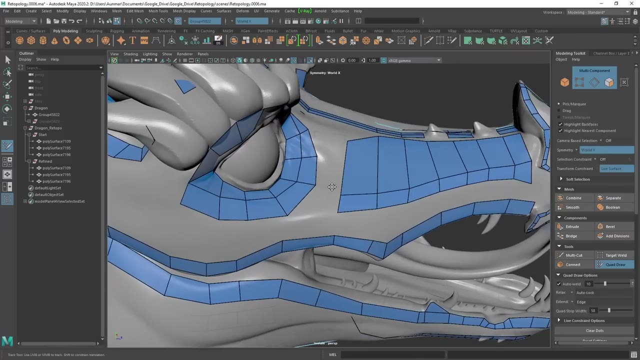 detail that ran there. but we'll come back to that one. I'll show you at least how I handled that and we can start continue with this. we can start to see that I'm going from here continuing the orbit of the eye, so I'll kind of stop right there so we can at least kind of see how now I'll connect. 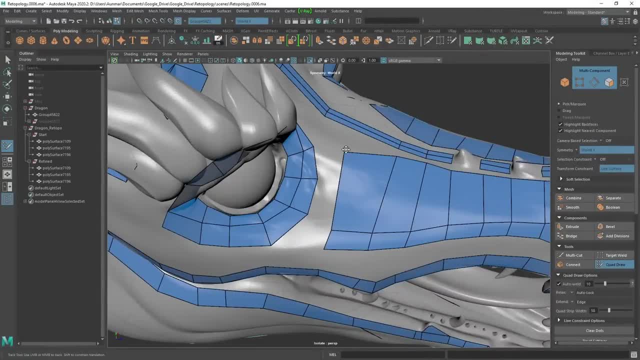 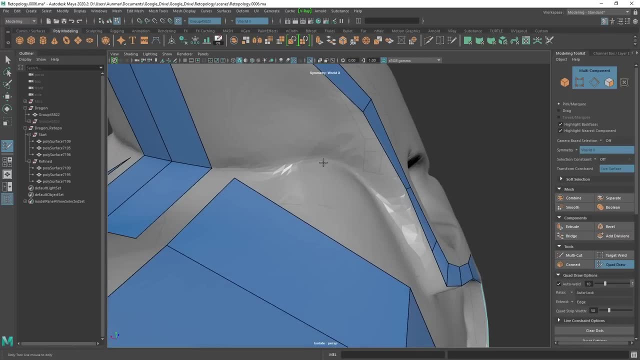 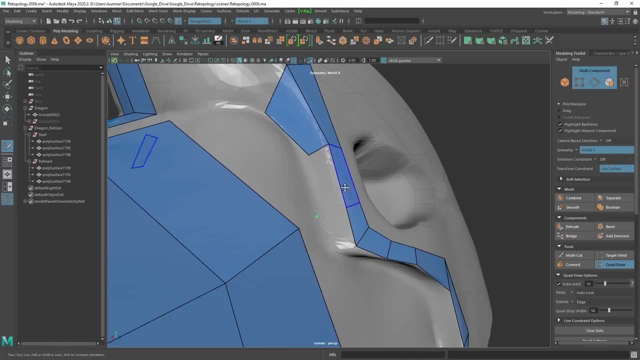 these parts here. so I know now I'm going to have to match one, two, three of these edges, along to about this part of the the dragon's nose. so now I'm going to come down to here and we're going to see how you know, we're going to merge these two pieces here. so if it gets a little bit, 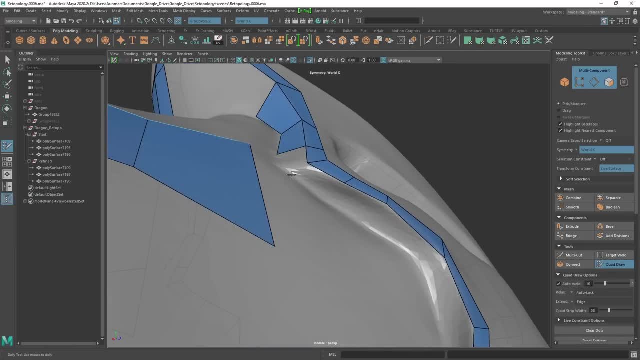 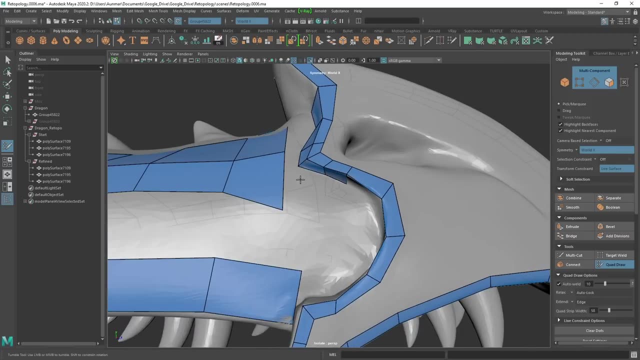 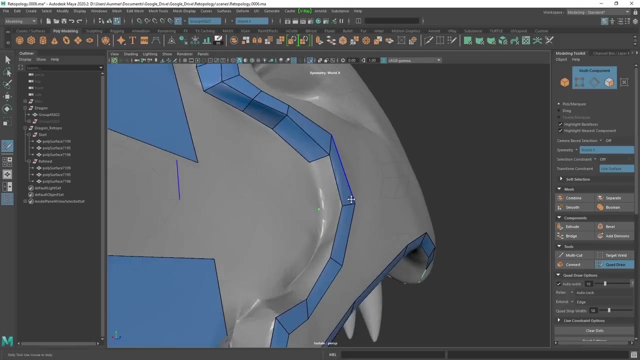 tricky. I'll just go ahead and tab left click and that should work and this is why I didn't go crazy and add too many pieces of geometry. but I'll show you kind of how you know, we'll see how I handle this area here right, and I'll go ahead and continue that. 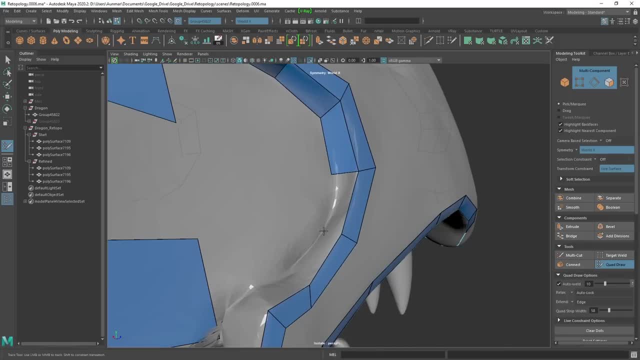 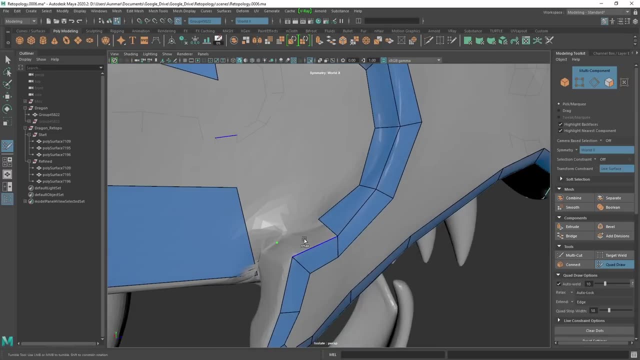 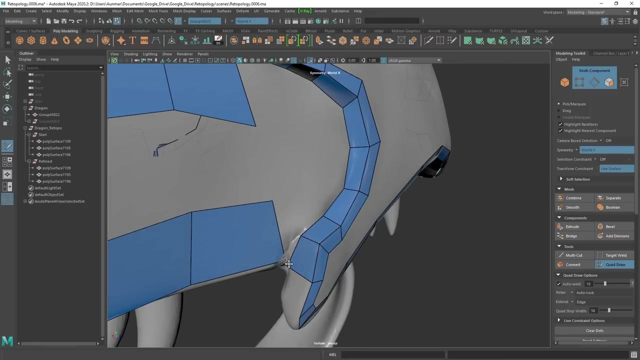 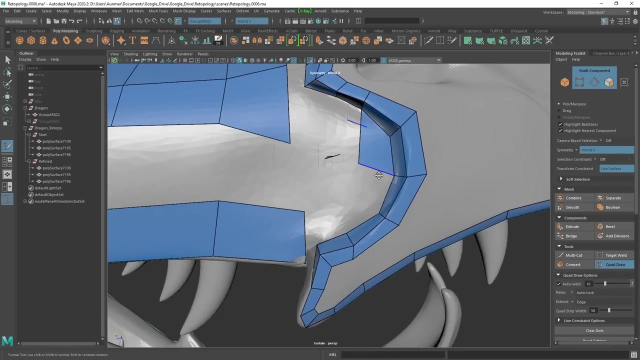 continue this here, kind of left clicking on the inside, and we get something like this right now. so I'll keep this one, I'll just tab this one out, all right, and I'll probably go from here. all right, so we get something like this now. well, that's where I can start to add in this point. you: 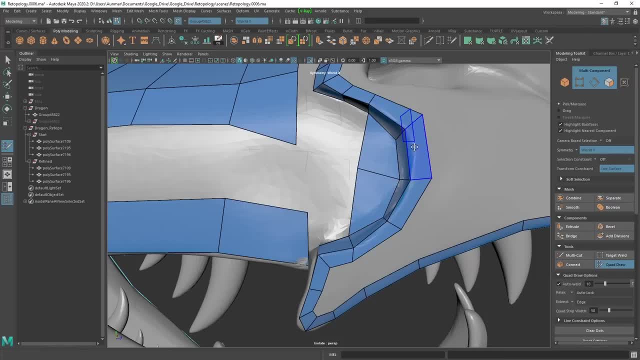 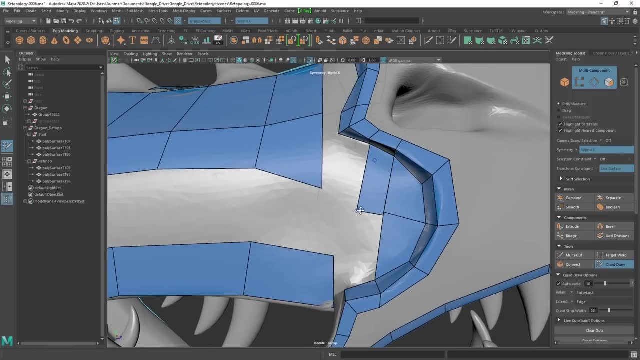 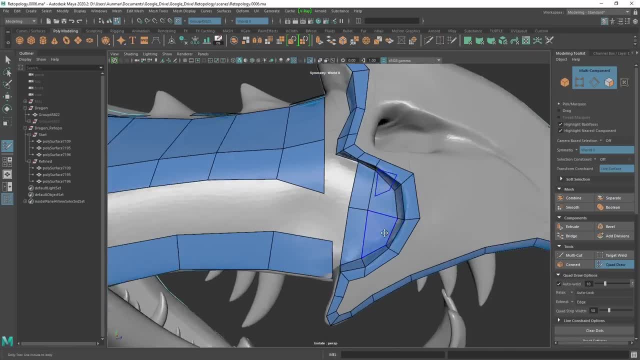 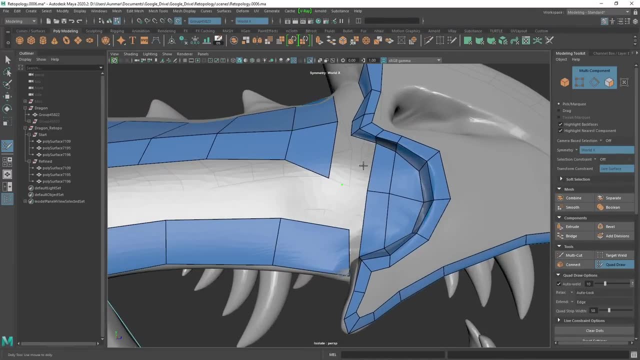 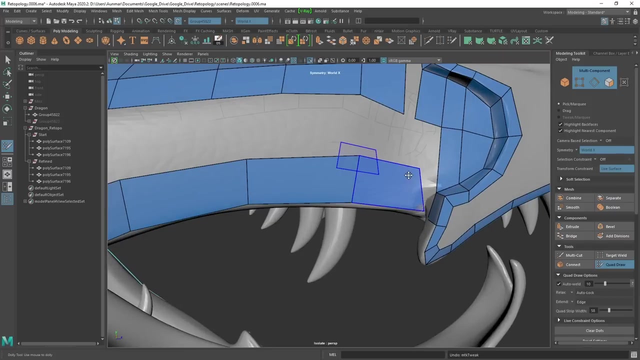 we get something like this and i can weld this edge, so good. so i'm starting to get some pretty good geometry here. i would say i have one more that i can add there and maybe i can bring this down, probably a little bit. i'm much, much closer lower here. 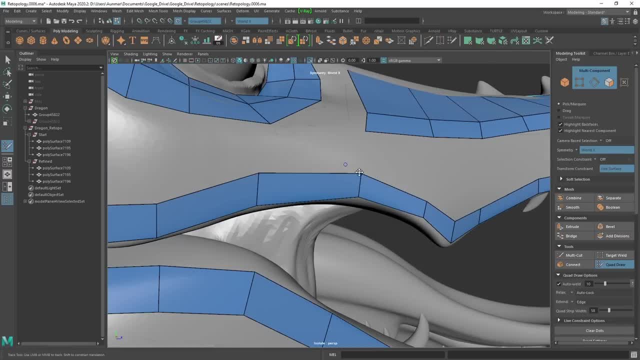 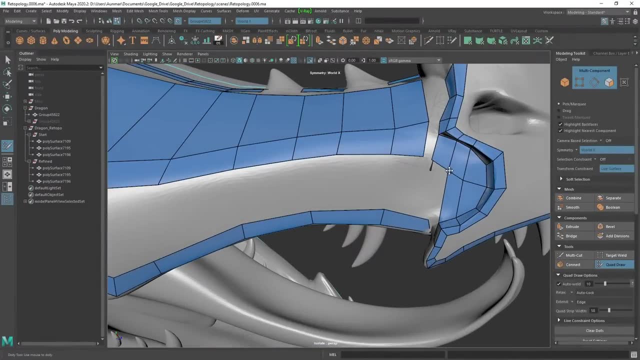 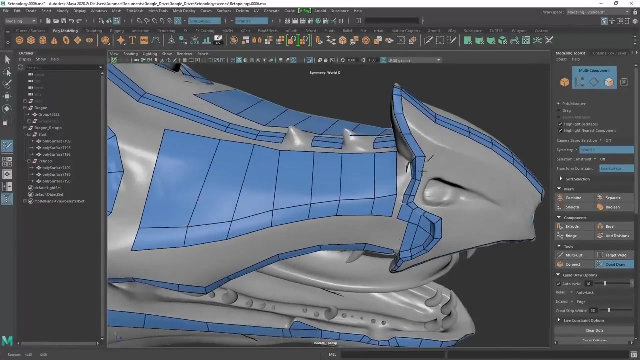 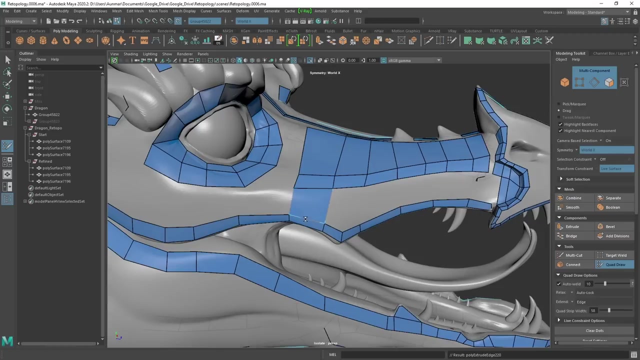 all right, so i'm going to keep this a bit tighter for now. all right, so we have that and we'll keep this kind of following, this main highlight here, and we can focus on that, and we have this so far. so i'll go ahead now so you can see what i have here. i can go ahead and start to weld these together, so i've 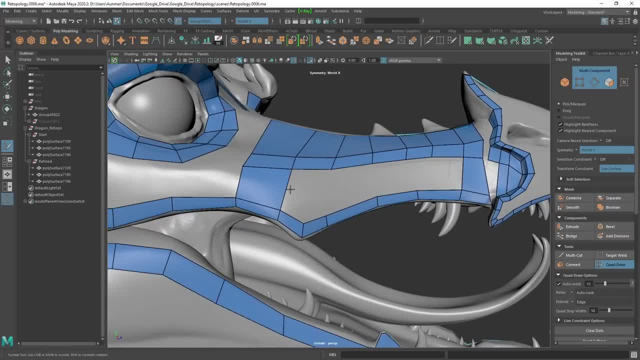 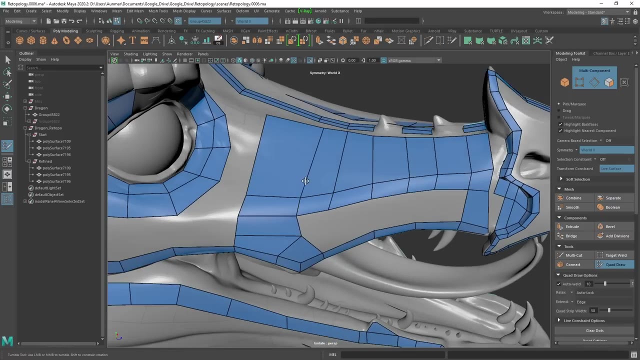 welded those together and then you can see, now i'm going to go ahead and add one more here in the middle which i know i'm going to need, and this is going to be part of this kite quad here. so i can go ahead now and kind of add this, like so, and i can move this a little bit over. 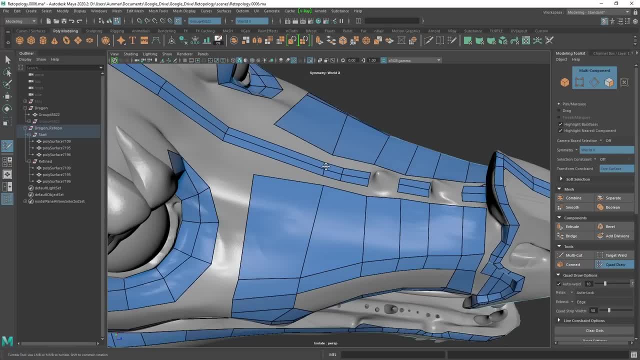 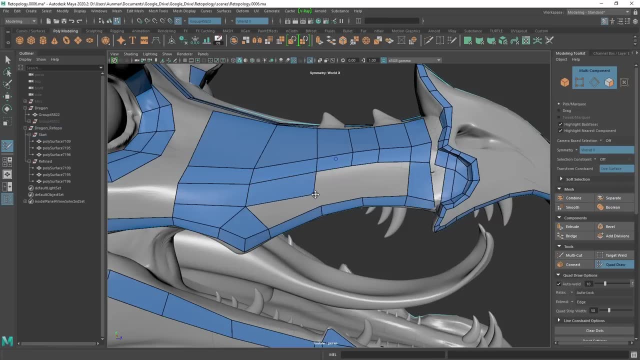 and we can kind of see how we uh deal with that. so it's just kind of adding and removing as we go and you know i'll go ahead and tab uh left click to bring that out and go ahead and snap these verts right so you can start to see again how i'm just 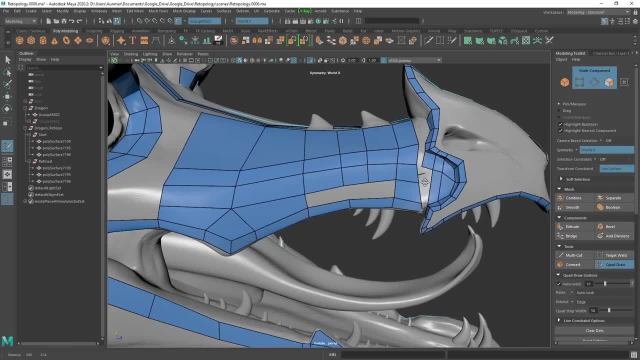 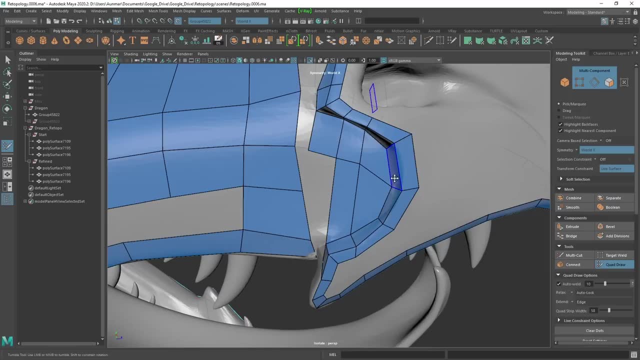 you know, adding this at a high level here and we get something like this, and then now, if i need to, we can go ahead and add a little bit more geometry to this part of that dragon, or the nose of the dragon, so i can go ahead now and add that in there. so i'm only adding in as 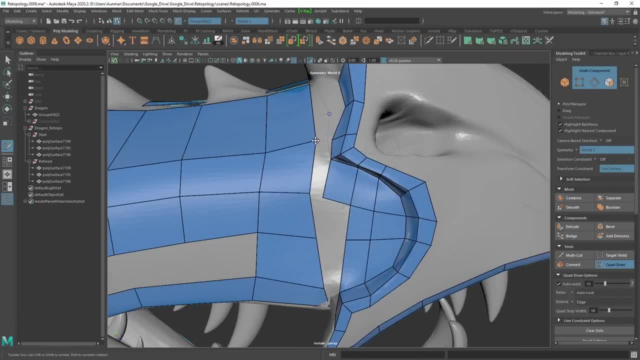 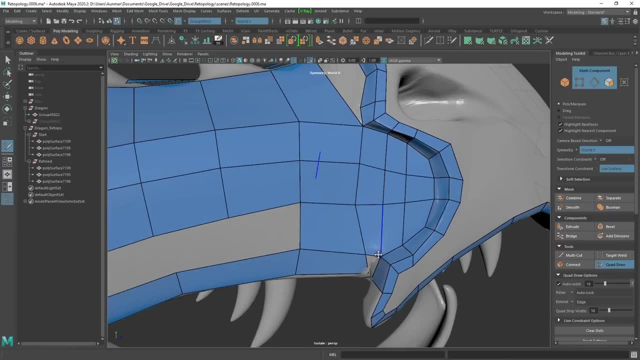 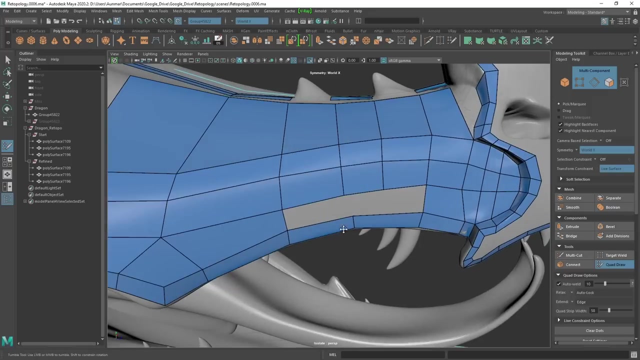 i needed to conform to the geometry, right? so i can go ahead and kind of follow these and start snapping these together, and there we go and i'll just kind of move this, finish that off there, and you can start to see, i'll move this over and just boom. 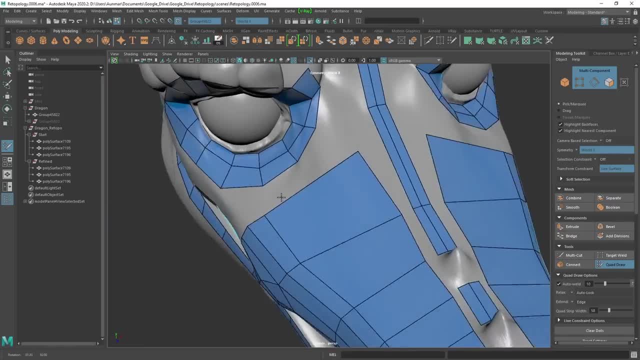 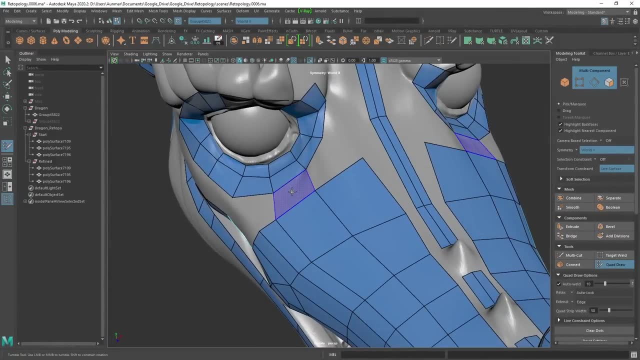 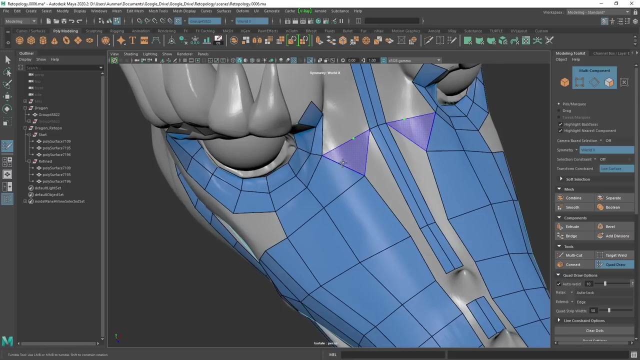 add in that so you can kind of see how i'm going through and doing this part, and then we know we're going to need probably another edge that runs along here. and then now we can start to connect the eye uh portion uh over here and we can kind of come up to this part of the brow. 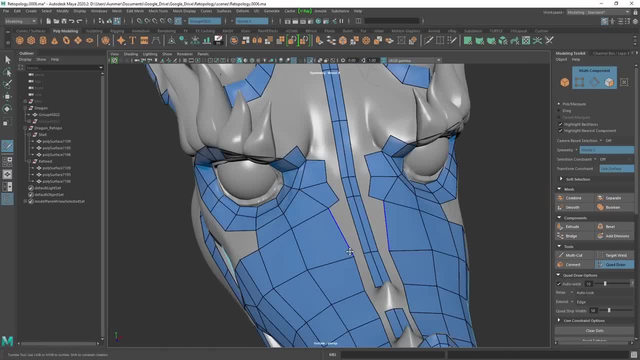 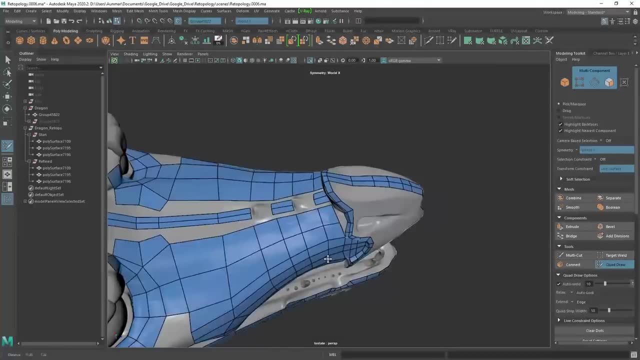 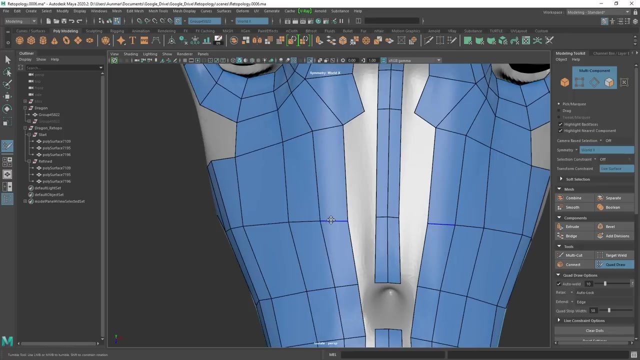 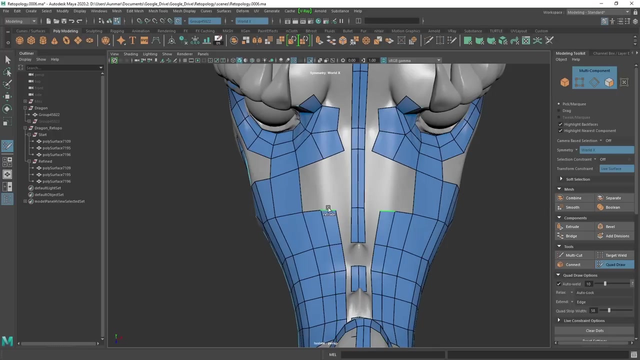 and we can start to add in that geometry there, right, so i'll probably take it to maybe a little, maybe just about here, where i can bridge this, maybe i'll just add in one more edge that runs like: so i'll do it like this and we can tab that to connect this. 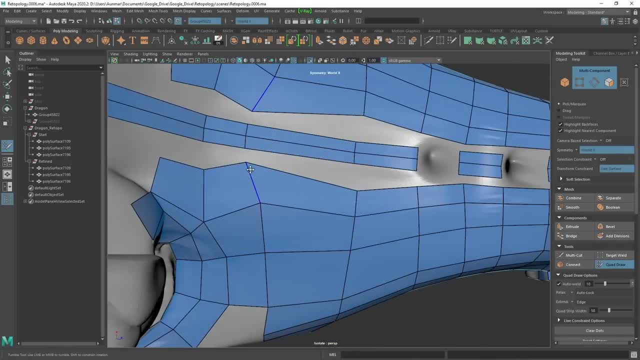 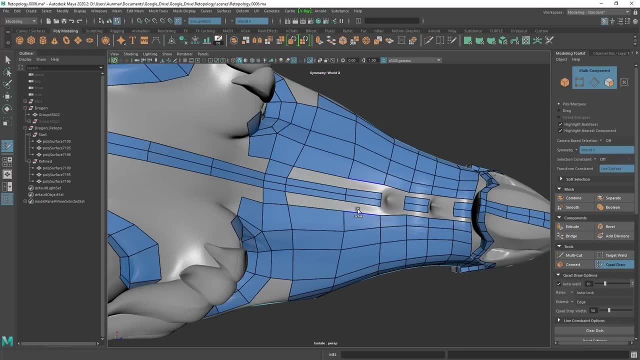 and we'll just, uh, shift, click that you can kind of see again just how we're just manipulating and adding and just making sure that we're keeping the same amount of geometry that we're going to, to make sure that we're keeping the same amount of face loops and edges to add and to connect. 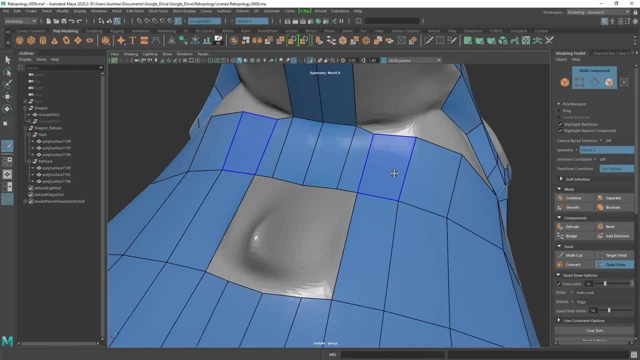 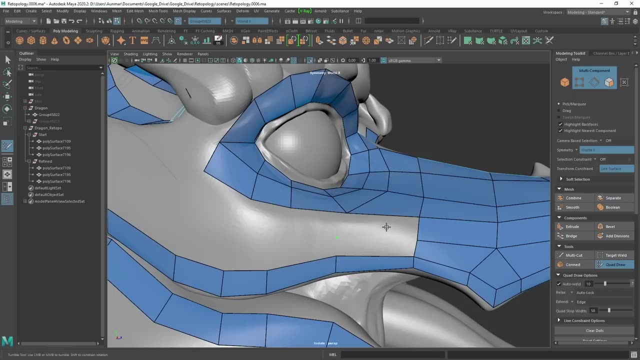 from one end to the other kind of mess that one up there we go. so i i think i can, you know, you, you get the idea i didn't want to go too long here, but uh, because i'll show you kind of uh, a narrated version, uh as well, and so you can kind of see i now i can continue this. 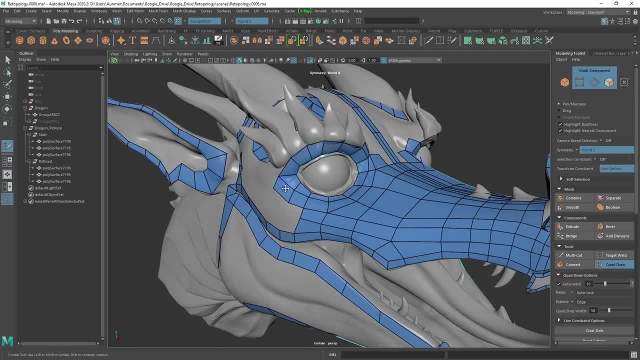 and working my way. so this is just a quick high level of how i'd start with the eye loop in the face loop and then i'm going to add in the edge to connect that, to connect it to the other end of the edge loop, work my way across and you can see now it's a little bit uneven. no worries, that's where i can. 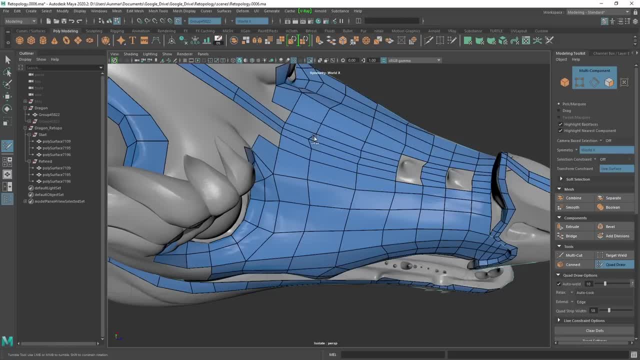 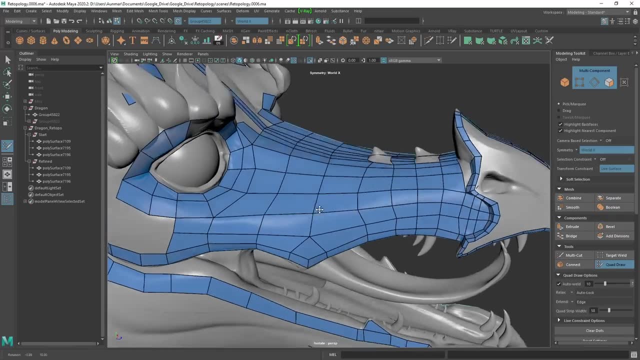 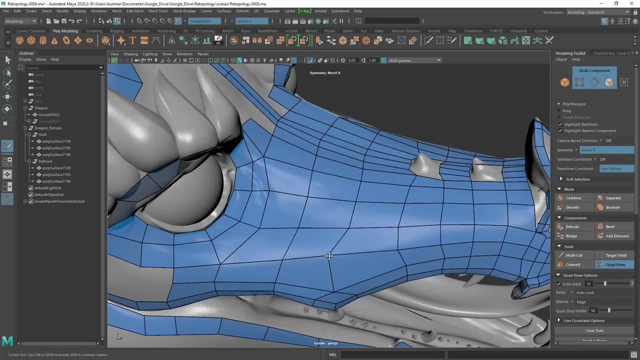 start to hold shift and start relaxing this and getting that nicer detail, um, and distribution of edges along our mesh, and look at that, it's starting to really clean that up. and then now i can space things out even and add in more geometry, without you know, just kind of focusing. 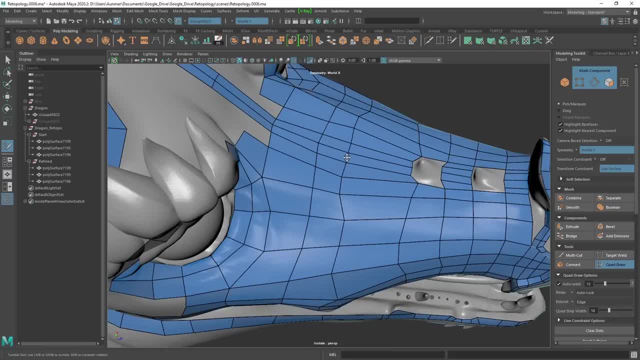 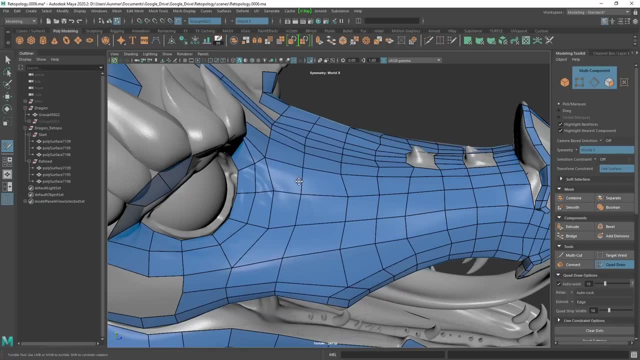 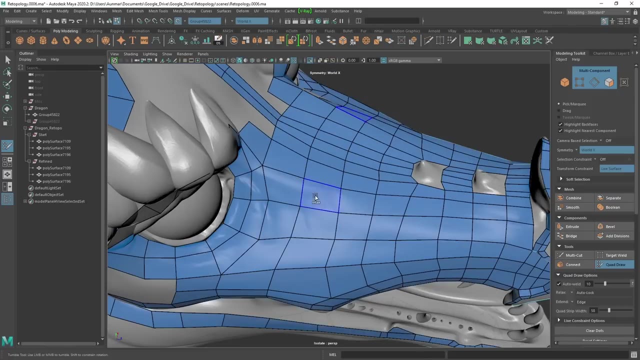 on the overall form and if i need a little bit more. you move things up, you space them out and move that. now you can, of course, entirely manipulate entire edge loops with middle mouse, middle control, shift, middle mouse. there we go, and you can just now start to shift left click. 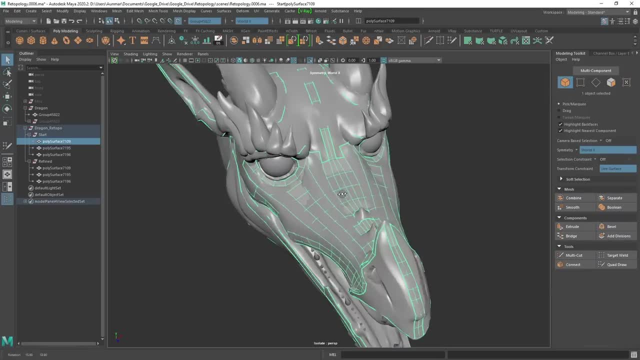 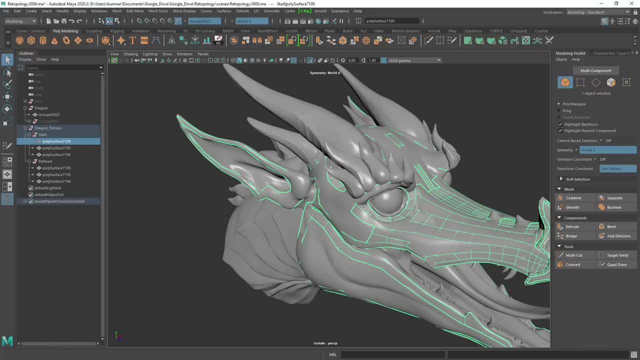 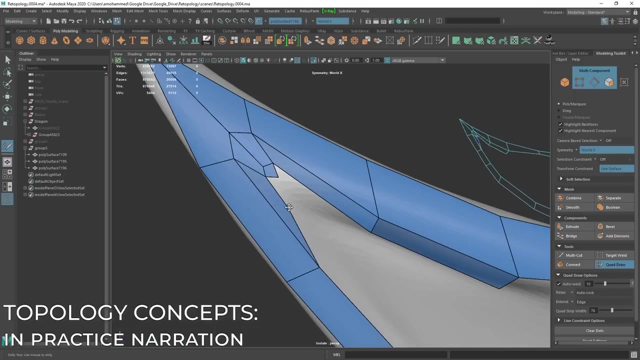 and just kind of relax that out. all right. so, uh, next i will cover um how i handle the ear and narrated uh, and just do a quick narration of that uh working right now. so this is a time lapse. this is sped up just so i can kind of narrate what i'm doing here so you can see that i already have the ear loop. 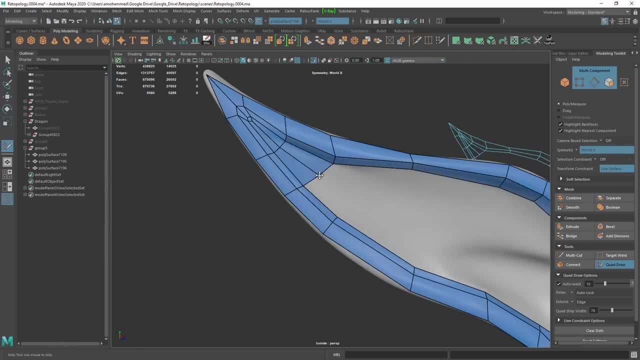 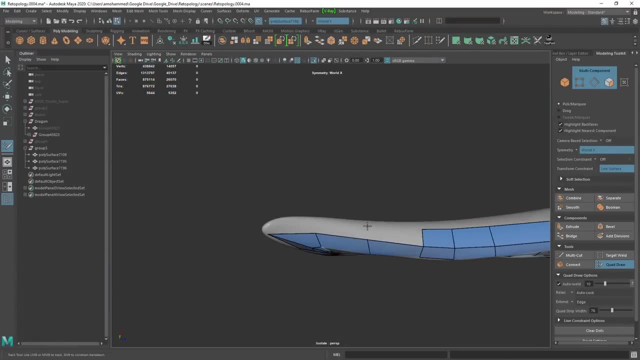 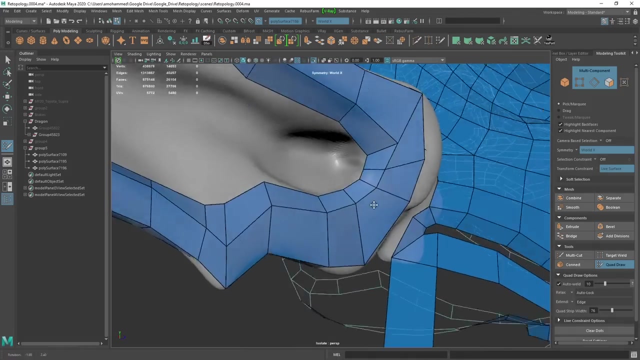 the, the key face loop that runs all the way around the ear, and i'm just kind of building off of that. all right, and once i build off of that, i can then start to continue to add geometry where i need it. so i'm going ahead and kind of adding in the thickness that's around the dragon's ear and 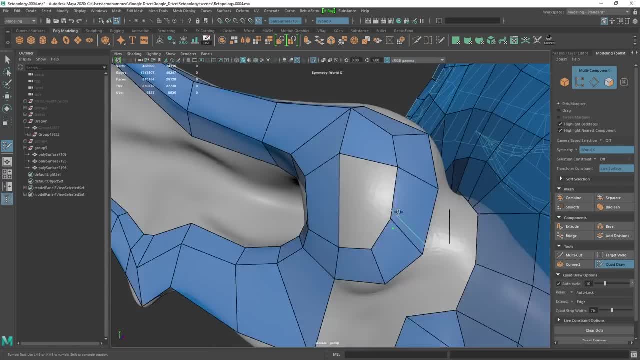 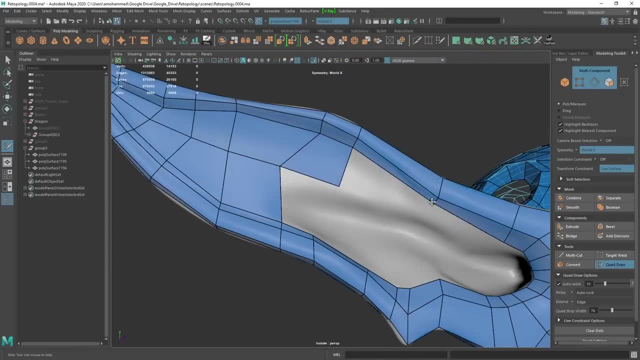 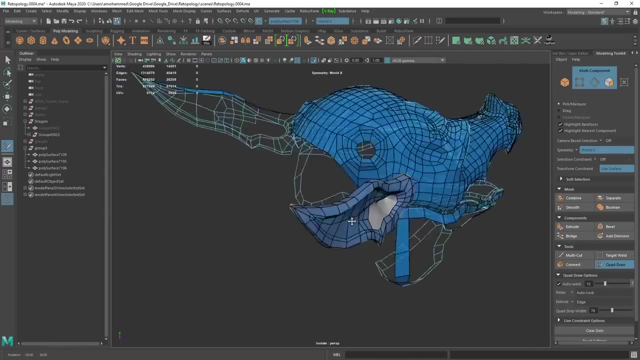 then i'm adding in geometry as i need it and i'm focusing on good, clean face loops and a good even distribution of edges. now i'm going to the inner part so you can see how i'm going from a very narrow tip of the ear and how i'm going into a much wider, deeper, more detailed part of the ear. 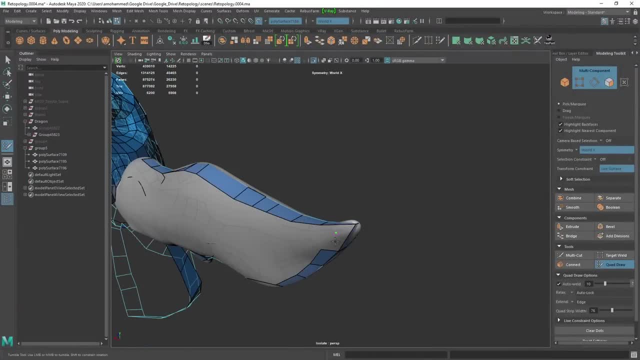 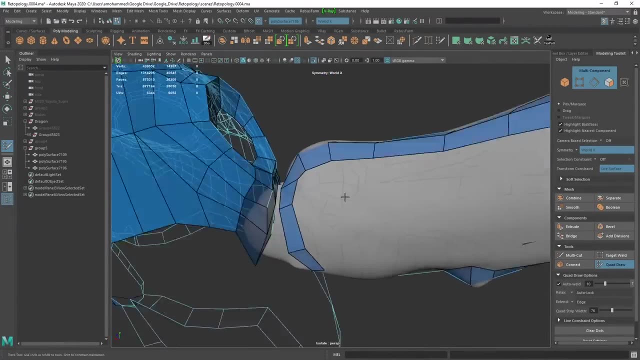 canal. and i'm using that same technique. you guys, i'm using that same technique where i go from six to four, four to six, two to three, um, and then now i'm building, just like the back of the ear. i started building the back of the ear at this point so i can keep the geometry matching all throughout, and 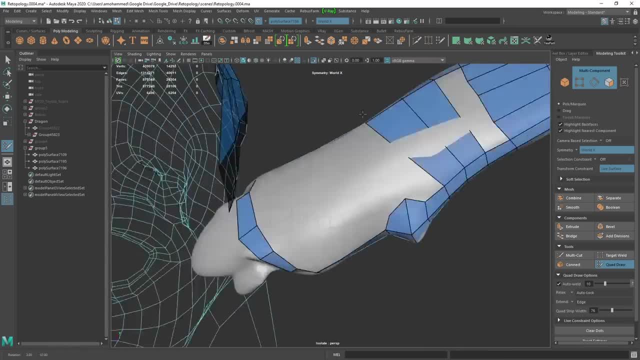 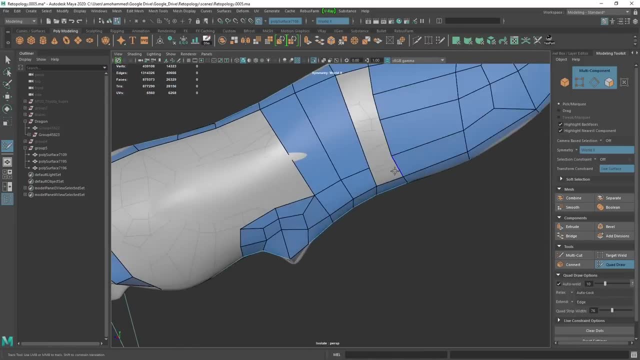 you can see, i've started to add the two of them, and then i'm going ahead, and i'm going ahead, and i'm going through the two to four geometry method, uh, the face method, and then now i'm going through and adding in- you know that technique, all throughout the mesh i'm localizing my topology. 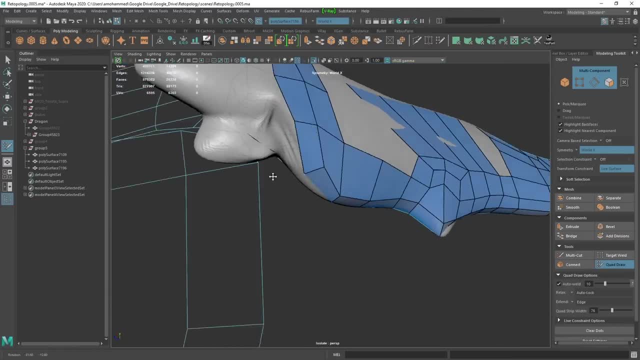 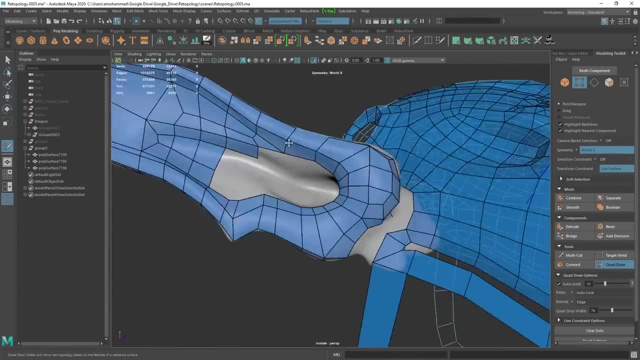 only adding topology where i need it. and you can see, i'm using the technique that we just talked about, where i'm using large faces and then just connecting from one end to the other, which helps save- uh, saves- quite a bit of time. and then i'm back here at the ear canal, now that i got the 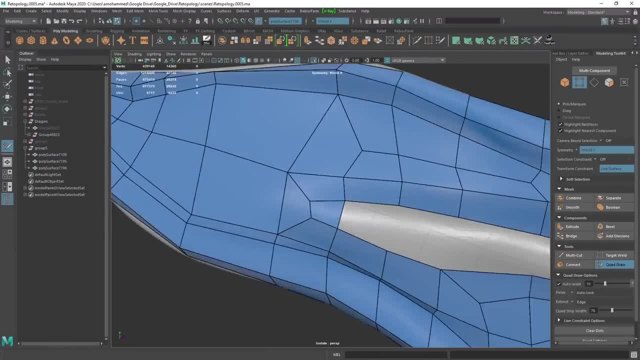 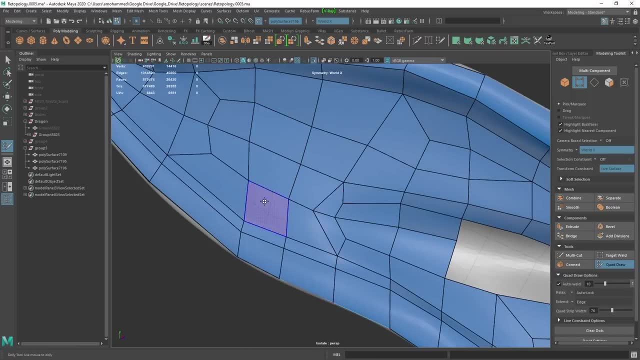 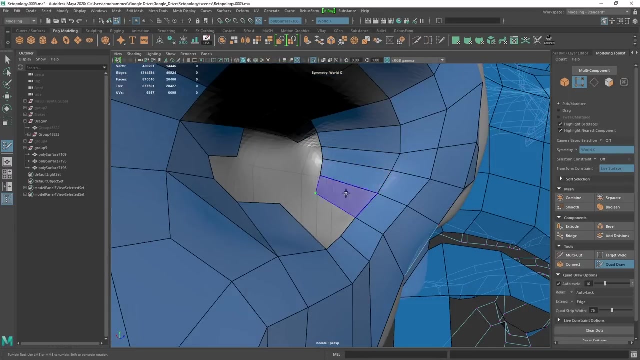 rest of the geometry blocked out and i'm going through and just using a common combination of kites, quads, going from four to six um, adding a triangle, uh, in a rigid area and then just kind of finishing everything out. i have nice clean face loops, nice clean edge loops. 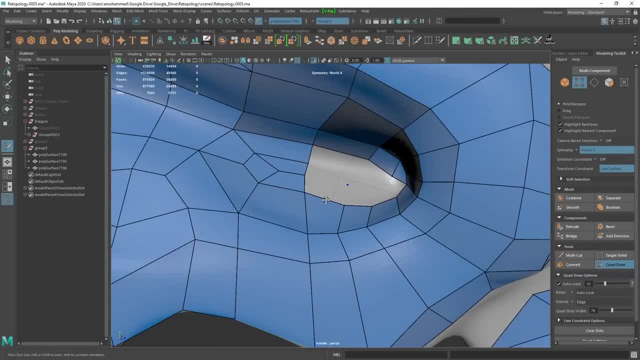 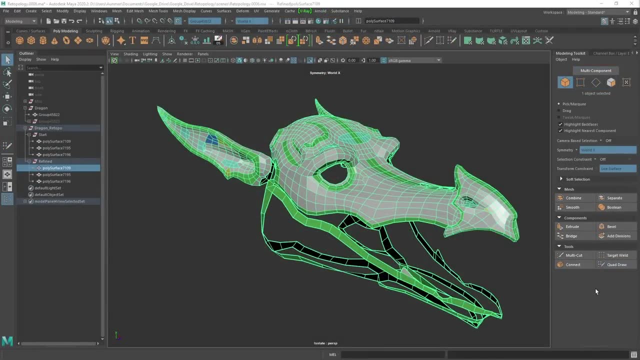 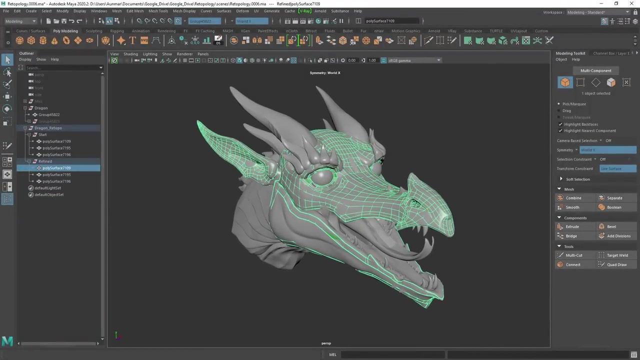 and just controlling the overall topology. so i'm just taking these techniques that we're talking about and applying it through this complex object, all right. and so the last thing i wanted to cover is just to make sure to understand and to look at some good reference and to study, to study, topology, right. so here's, like this shoe. 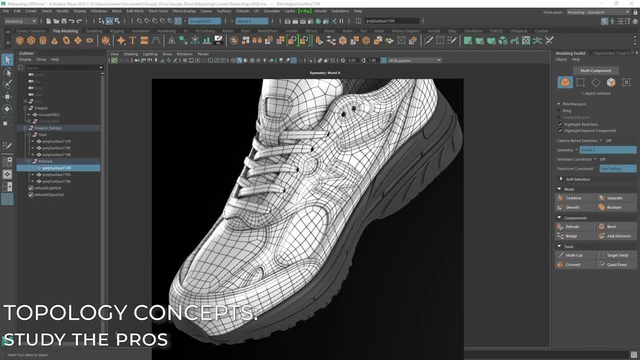 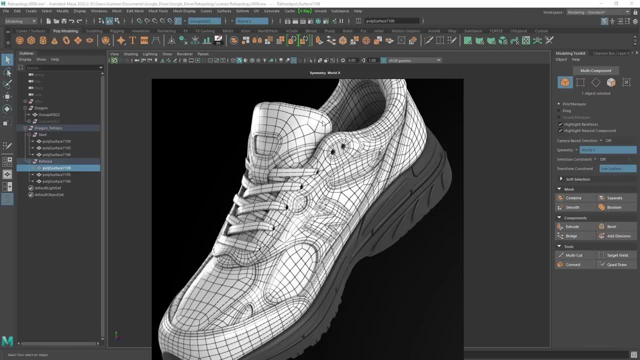 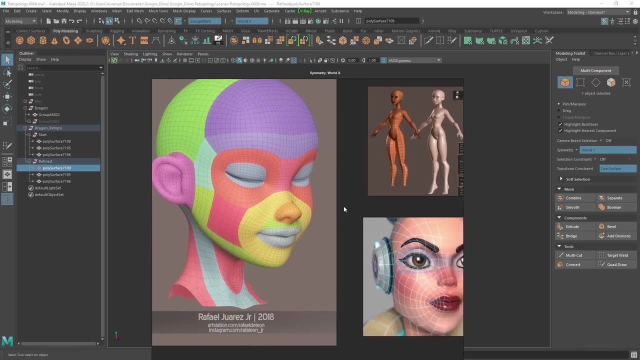 model that you can see that i'm using those types of techniques all over the place. you'll see that i'm using, you know that, uh, double kite here all throughout the mesh. uh, just to add some geometry, i'm using the the, you know, four to two, or two to four, four to six type edge flow, you know, study. 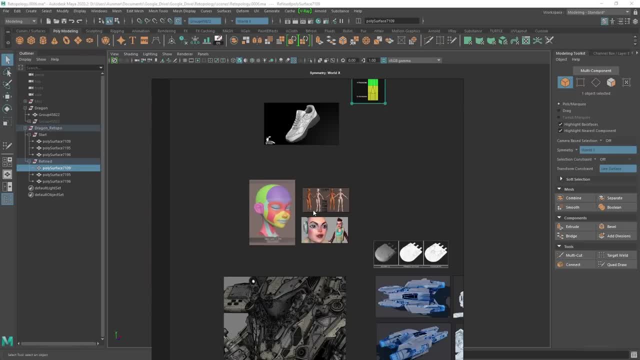 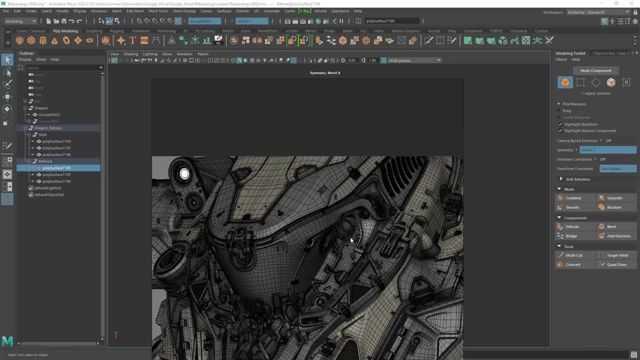 good character, topology as well, hard surface and organic stuff. you know you'll see that everywhere these techniques aren't specific to hard surface, aren't specific to organic characters. you know- and here's some some nice hard surface examples here- that i'll jump to art station in just a moment. 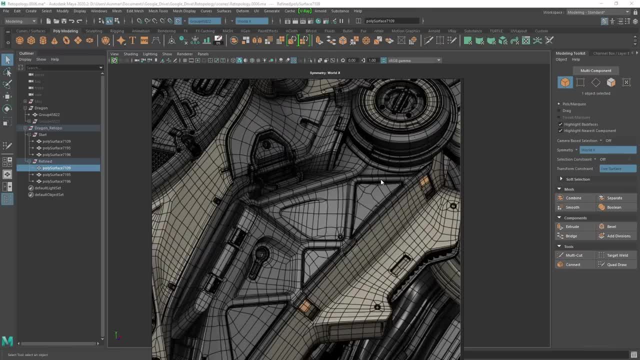 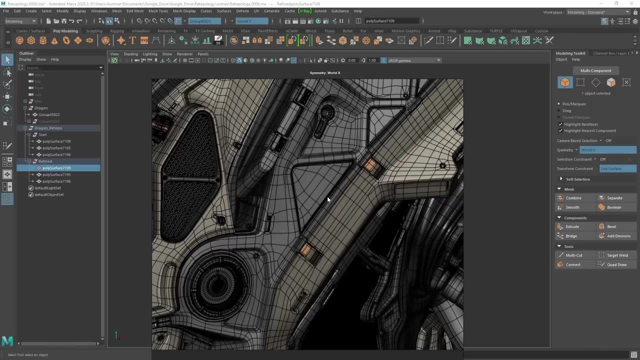 um, where you can see. you know, if you, if you find a good surface model or hard surface modeler, you're going to find these techniques just all over the place. now remember, triangles are 100 fine, especially on flat surfaces. but you'll see, you know, going from you know. 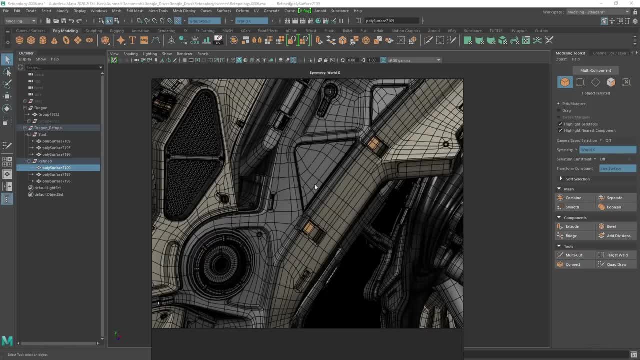 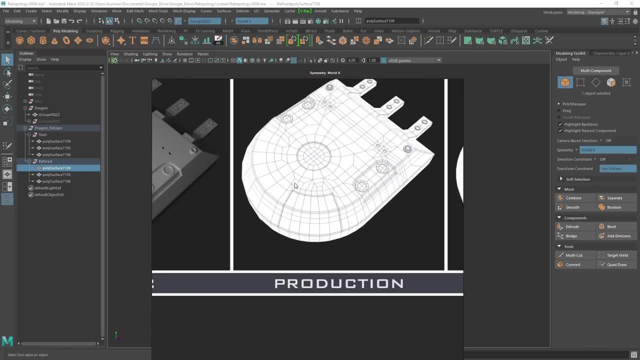 localizing areas of topology where you're going from wide- a lot of topology to narrow, you're going to be using these techniques that i've talked about today. you know exactly here you can see, uh, these, these types of examples with with topology here going from the one. 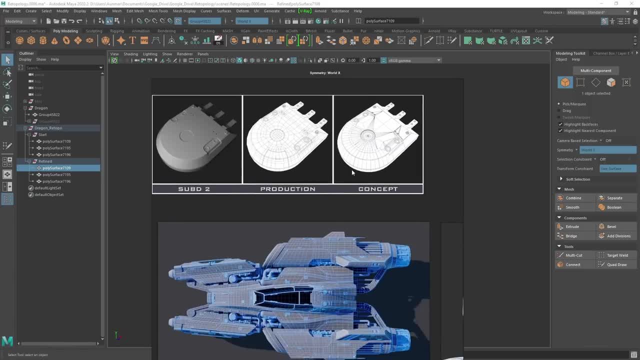 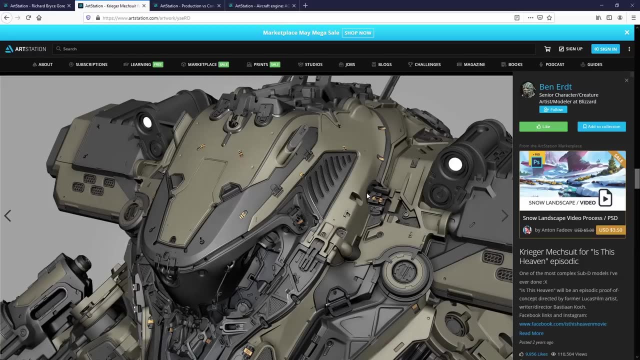 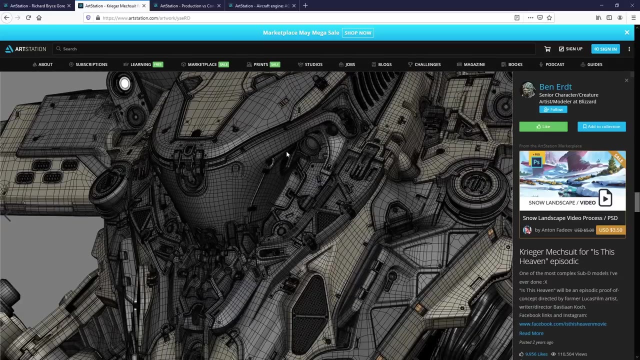 to the two to three uh faces here. it's just, it's just the way to do it all right. so some good examples there. and you know, you can see here the guys that i'm referencing from art station. here's ben ert, um, you know, i think aramis did a good breakdown, aramis3d, uh, where he talked about uh. 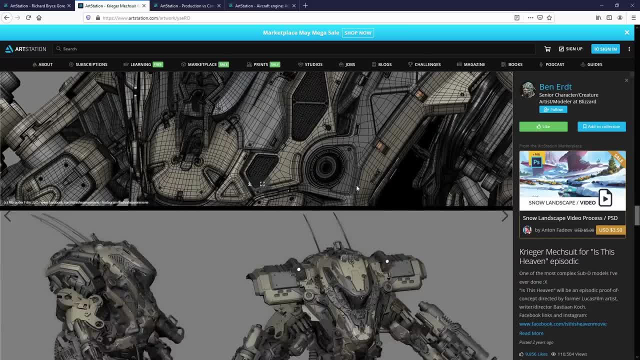 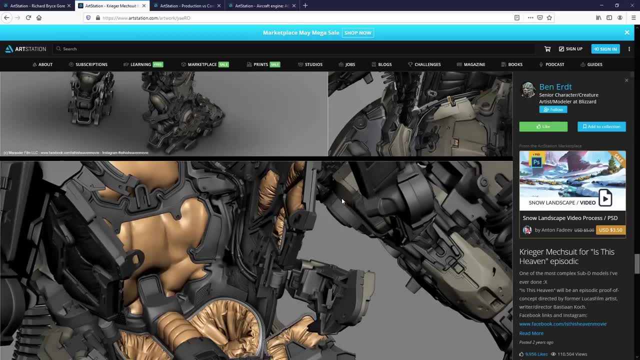 just his workflow and workstation, work style, uh, so make sure to check that out. but you know, just, you know, take a look at what, what a lot of the professionals are doing, uh, industry professionals, you know. so i'm trying to do my best to share my information, but you'll see just so much more information, uh, and examples out there. 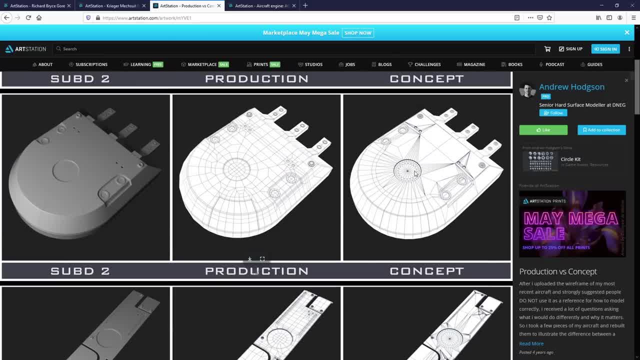 uh, here's andrew hoshton, where he shows how he, you know, starts with the concept- just you know nasty triangulated stuff, just get the form- and then he shows how he goes from that, the concept, to production and then finally the sub d model, which is just a subdivided version of this and 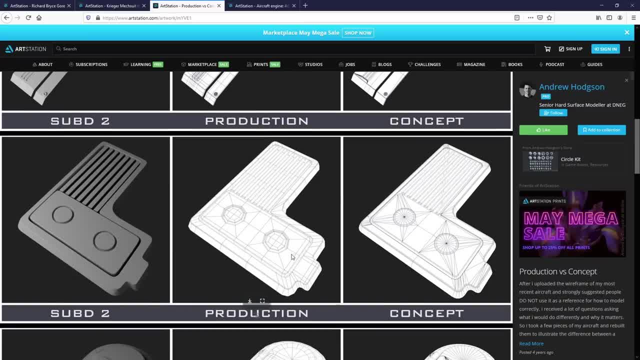 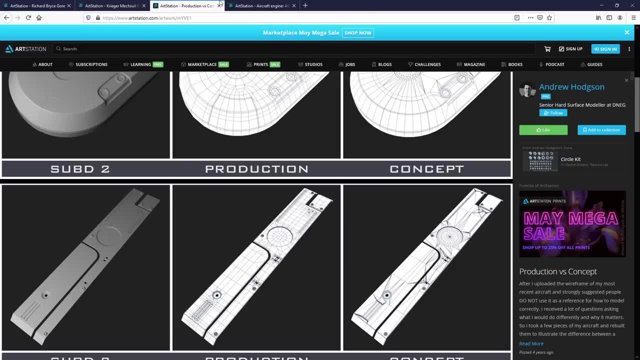 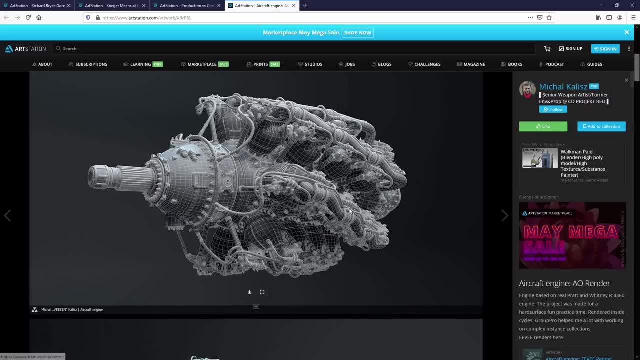 he's using is all throughout um every single one of his models, which is just again just how you do things, all right, so i hope this was helpful. again, it was just kind of another um deep dive and uh, oh yeah, i almost forgot about this one, this cool looking aircraft model by michael um color is: 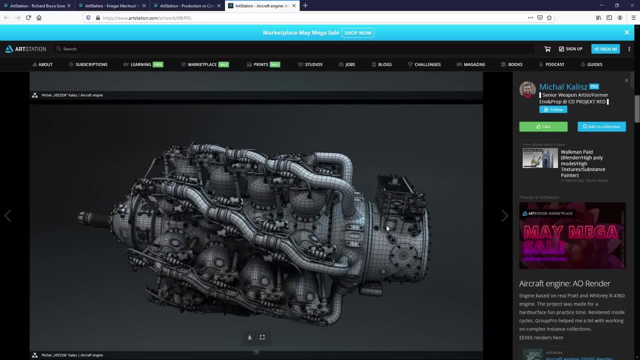 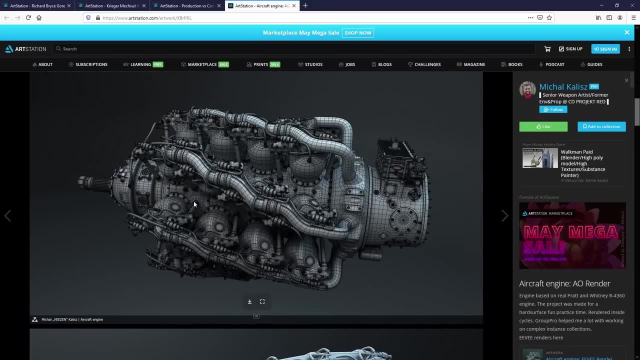 here and he just i mean, what's the cd project red? i mean this was just. i saw this, it was fantastic stuff and you'll see again. you'll just see this stuff all over the place with kite quads, diamond and you know. coming back to this, it's just this being applied over and over and over again, all. 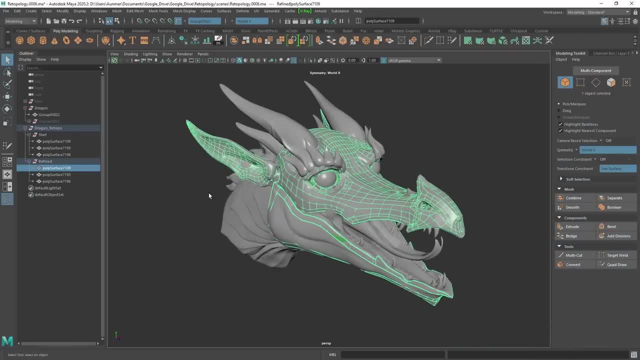 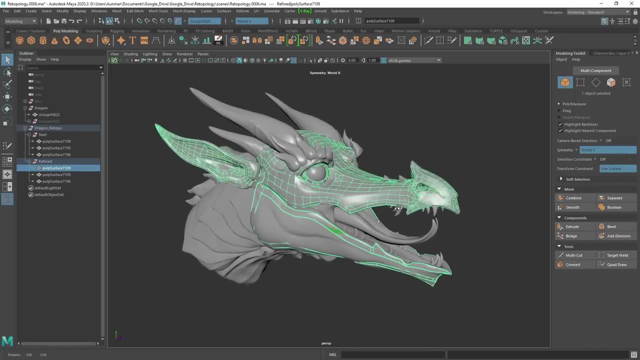 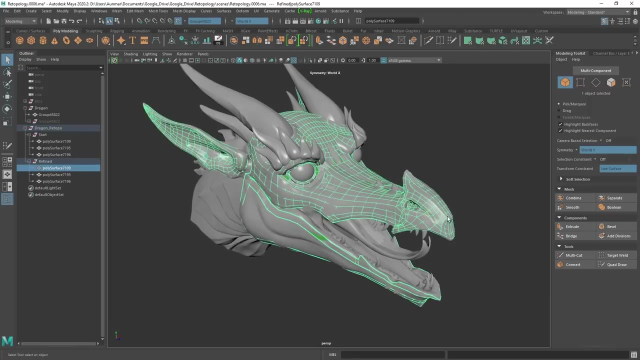 right. so i did my best to show you guys, um, that in practice, on this, what i would say is a fairly complex model, organic model, but it can be broken down into simple topology rules and you can start to create just a good even distribution, a good workflow, all right. so to summarize, 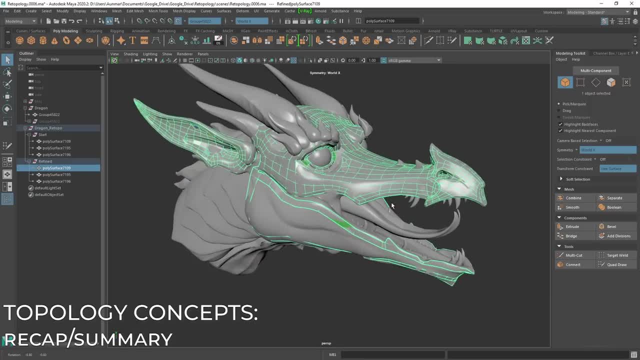 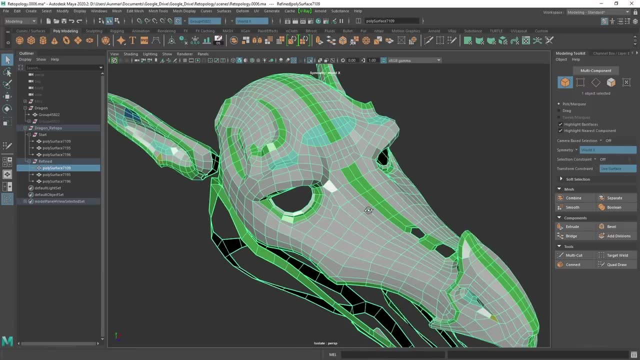 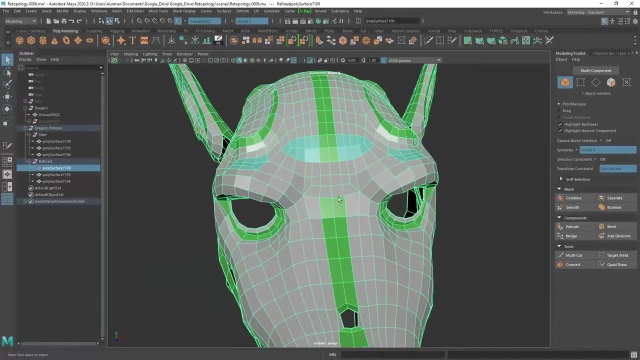 always start with edge loops and face loops. don't do the same thing, uh. just don't make your uh faces and edges too small, right? do localized topology, so making sure that you kind of keep typologies in areas that you need it and don't unneedlessly add geometry where you don't need it. don't just start adding. 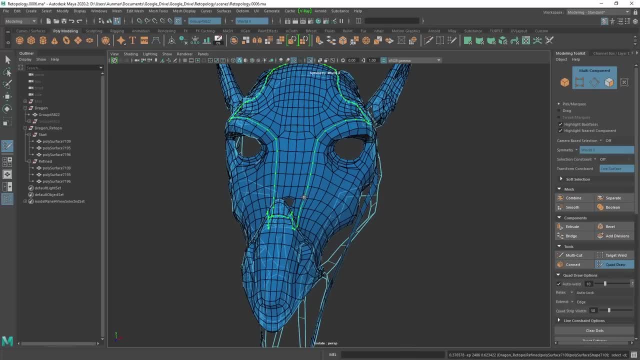 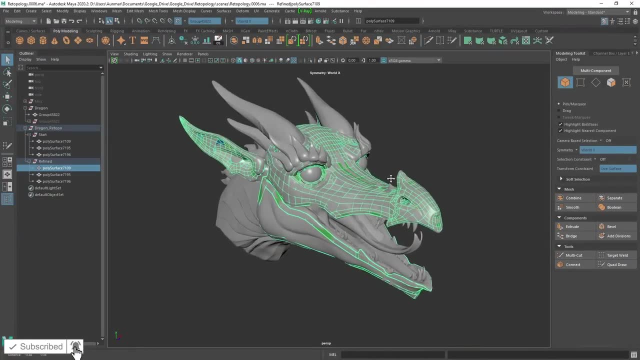 that's not going to add a lot to the form and you can just see it just starts to ruin things that you don't need. okay, so those are just some high level rules, tips, do's and don'ts when doing retopology, So I'll wrap it up there. If you guys have any, 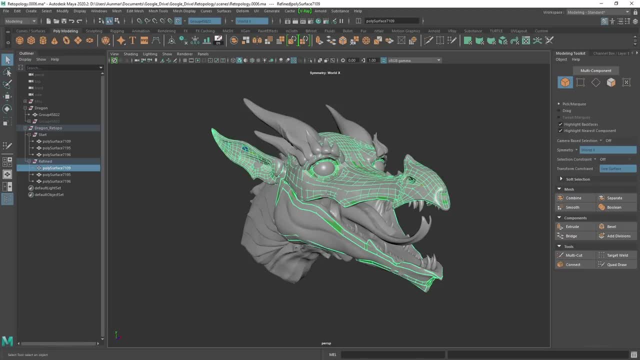 feedback, tips of your own questions, comments- let me know down below I'm hoping to now cover. jump back to the cyberpunk grenade where I'm going to be covering the high to low workflow. So I have the high poly sub D model And then I'm going to work on showing how to create the